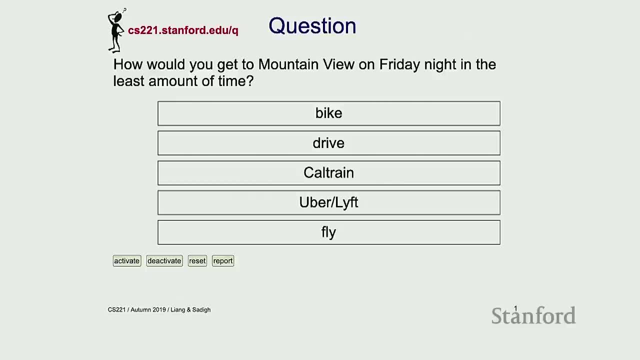 There are a lot of actually startups working on flying cars, Um. but but as you think about this problem, like the way you think about it is, is there are a bunch of uncertainties in the world, right, It's not necessarily a search problem, right? 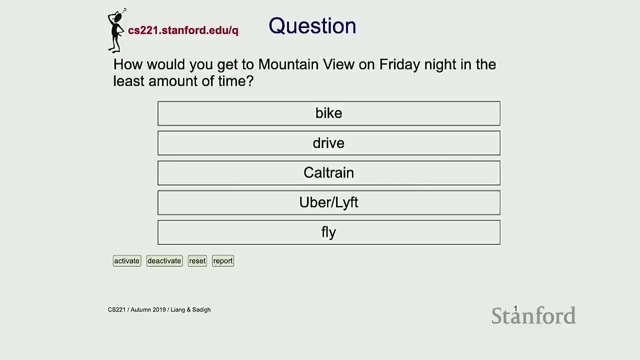 You could, you could bike and you can get a flat tire and you don't really know that right, You have to like kind of take that into account. If you're driving, there could be traffic. If you're taking the Caltrain. 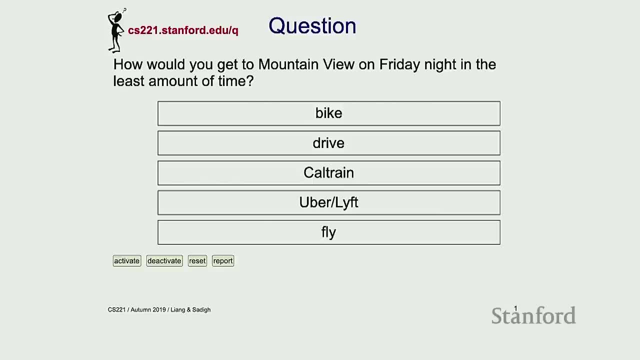 there are all sorts of delay with the Caltrain, Uh and and all sorts of other uncertainties that exist in the world and and you need to think about those. So it's not just a pure search problem where you pick your route and then you just go with it, right? 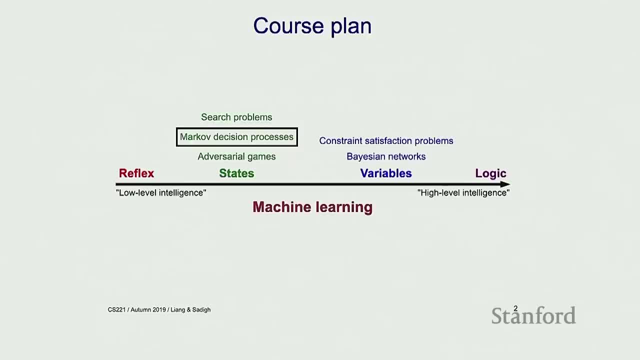 There are. there are things that can happen, that can affect your decision. So- and that kind of takes us to Markov decision processes- We talked about search problems, where everything was deterministic, and now you're talking about this next class of state-based functions. 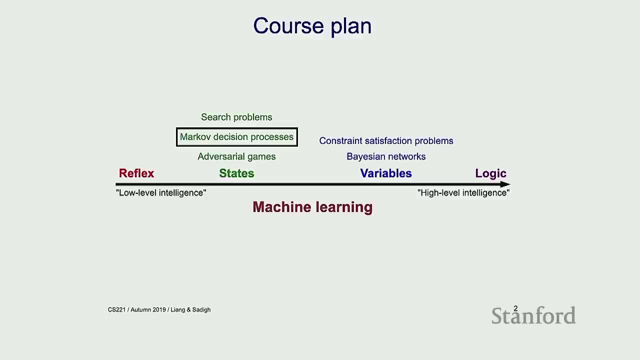 which are Markov decision processes, And the idea of it is: you take actions but you might not actually end up where you expect it to, because there's this nature around you and there's this world around you that's going to be uncertain and do stuff that you didn't expect okay. 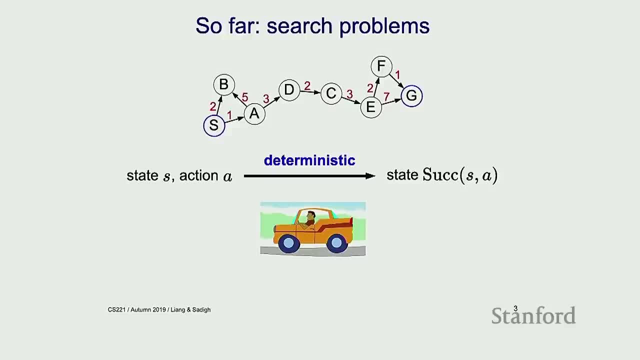 So so so far we've talked about search problems. The idea of it is you start with a state and then you take an action and you deterministically end up in a new state. If you remember the successor function, successor of S and A would always give us S prime. 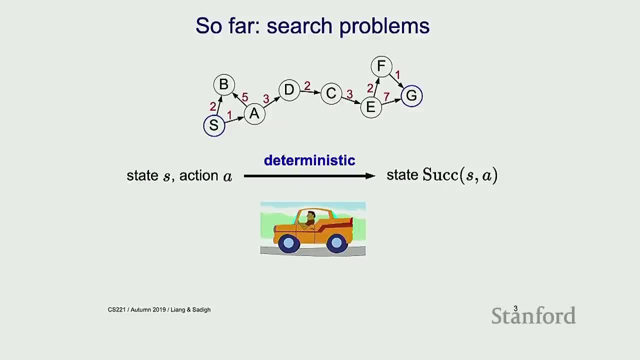 and we would deterministically end up in S prime. So if you have like that graph up there, if you start in S and you decide to take this action one, you're going to end up in A Like there. there's no other option. 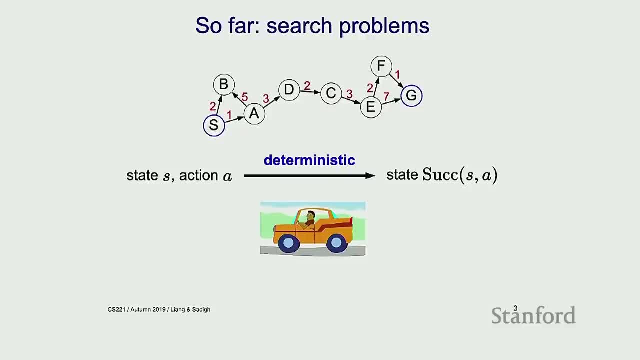 That that's how you're gonna end up in it, okay, And the solution to these search problems were these paths. So we had this sequence of actions because I know if I, if I take action one and action three and action two. 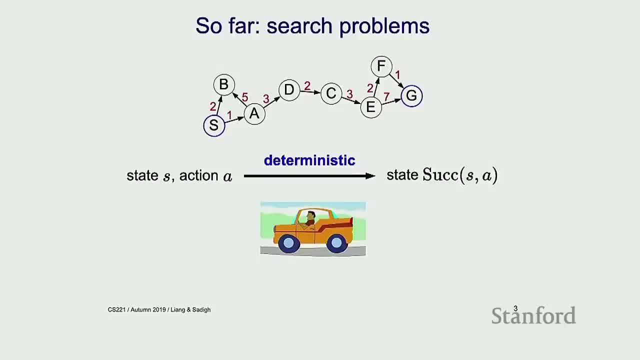 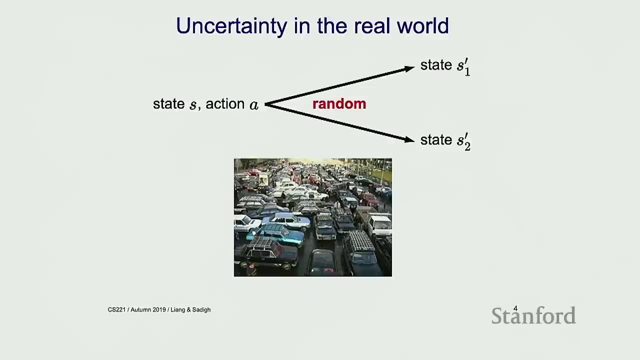 I know like what is the path that I'm going to end up at and that would be ideal, okay. So when we think about Markov decision processes, that is the setting where we have uncertainty in the world and we need to take that into account. 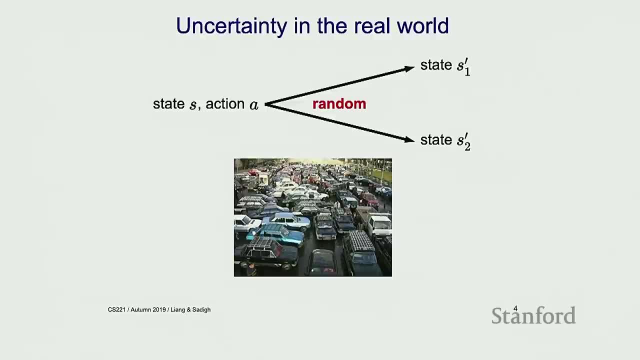 So so the idea of it is: you start in a state, you decide to take an action, but then you can randomly end up in different states. You can randomly end up in S1 prime or S2 prime, And again, because there is just so many other things that are happening in the world. 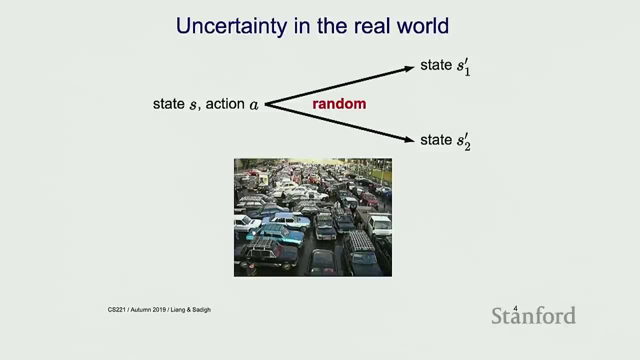 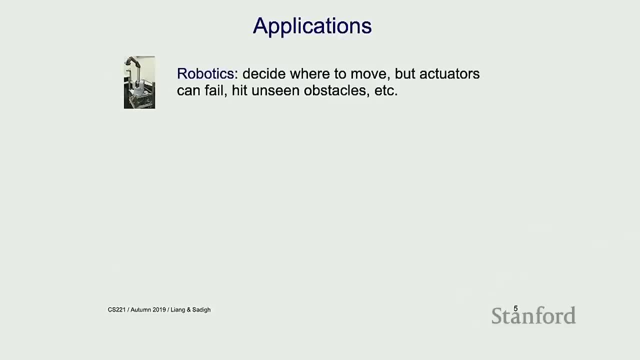 and you need to, you need to worry about that randomness and make decisions based on that. okay, And- and this actually comes up pretty much like everywhere, in every application. So, uh, this comes up in robotics. So, for example, if you have a robot that wants to go and pick up an object, 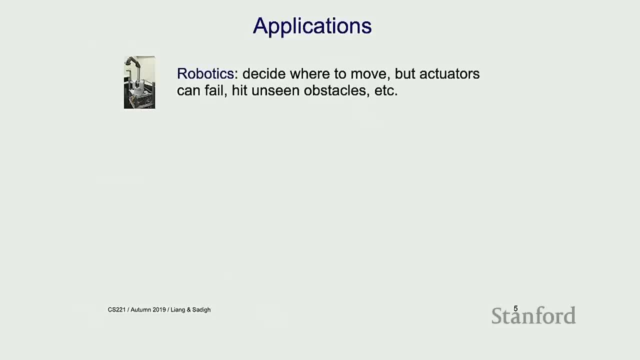 you decide on your strategy, everything is great, But, like when it comes to actually moving the robot and getting the robot to do the task, like the actuators can fail or you might have all sorts of obstacles around you that you didn't think about. 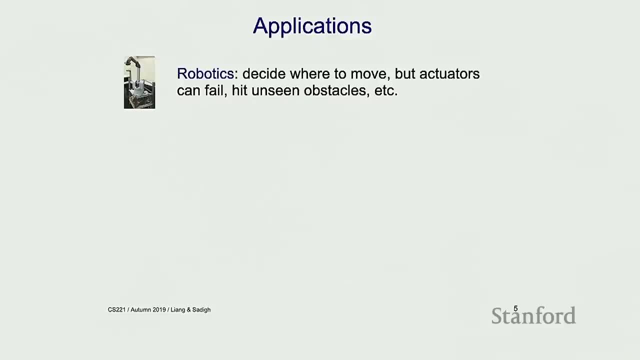 So there is uncertainty about the environment or uncertainty about your model, like your actuators, that that you didn't necessarily think about And in reality, they're affecting your decisions and where you're ending up at. This comes up in other settings, like resource allocation. 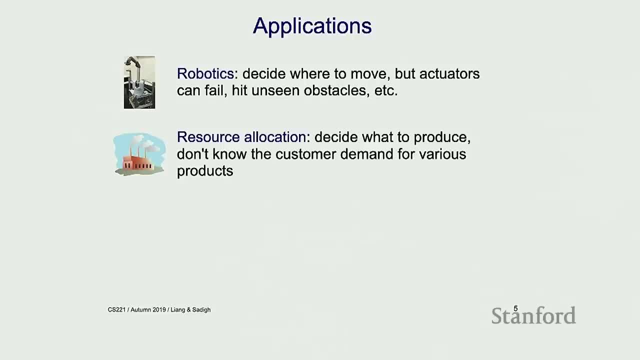 So in resource allocation, maybe you're deciding what to produce, what is a product you would want to produce And and that kind of depends on what is the customer demand And and you might not have a good model of that and and that's uncertain right. 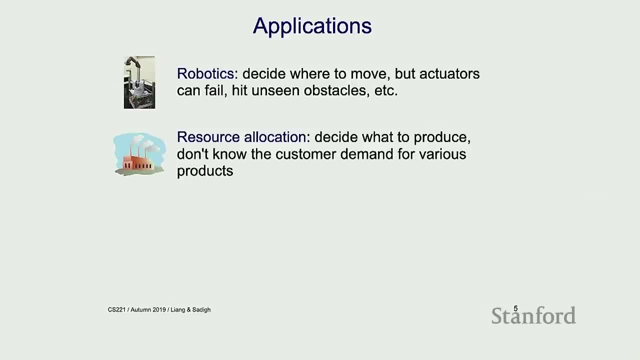 It really depends on what, what, what products customers want and what they don't. And you might have a model, but it's not gonna be like accurate And and you need- you need to do resource allocation under those assumptions of uncertainty about the world. 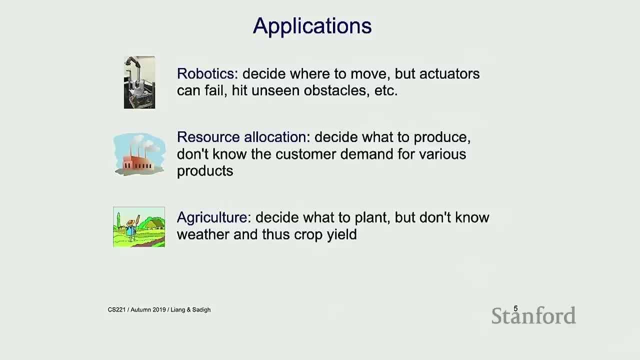 Similar thing is in agriculture. So, for example, you want to decide, uh, what sort of uh, what, what to plant, But but again, you might not be sure about the weather, or if it's gonna rain, or if the, if, the, if the crops are going to yield or not. 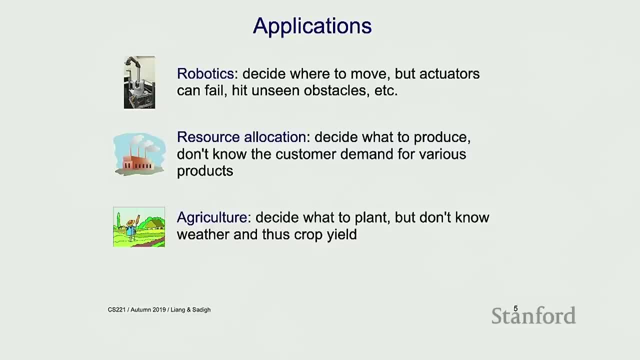 So there's a lot of uncertainty in these decisions that we make And and they make these problems to to go beyond search problems and become problems where, where we have uncertainty and we need to make decisions under uncertainty. Okay, All right. 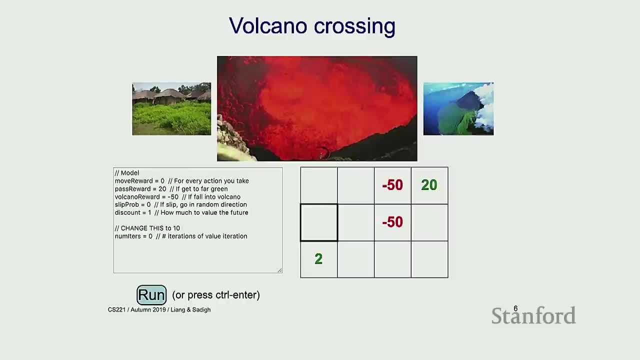 So let's look at another example. So this is a volcano crossing example. So so we have an island and we are on one side of the island And what we wanna do so we're in that black square over there And what we wanna do is we wanna go from this black square to this side of the island. 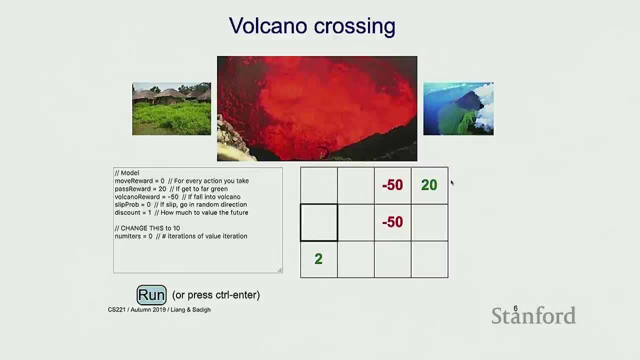 where we have the scenic view, and that's gonna give us a lot of reward and happiness. So so my goal is to go from one side of the island to the other side of the island, But the caveat is here is that there's this volcano in the middle of the island that I need to actually pass. 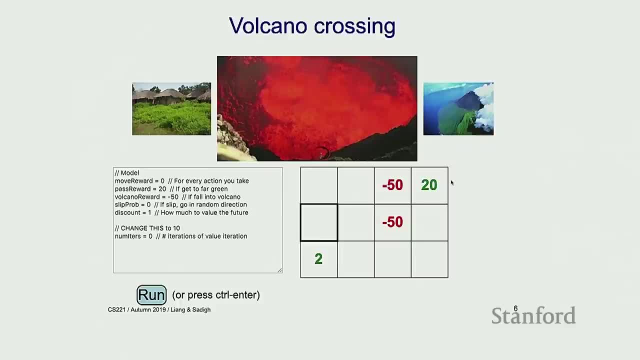 Okay, So, and and if I fall into the volcano, I'm going to get a minus 50 reward, more like minus infinity. But but for this example, like imagine, you're getting a minus 50 reward if, if you fall into the volcano. 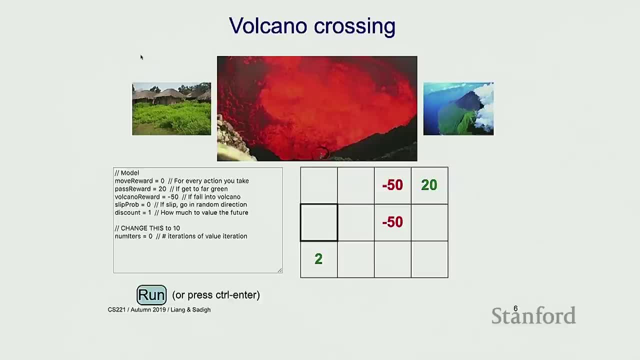 Okay, So all right. So so, if I have this thing here on this side, So if my slip probability is zero, which is I'm sure I'm not gonna fall into a volcano, should I cross the island? No or yes? Well, I should cross the island. 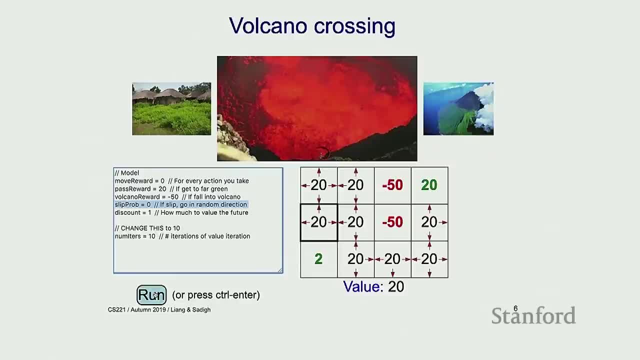 uh, because I'm not gonna fall right Like I'm. I'm not gonna fall into that minus 50.. Um slip probability is zero. I'll get to my 20 reward. everything will be great, Okay, But the thing is like we've been talking about how the world is. 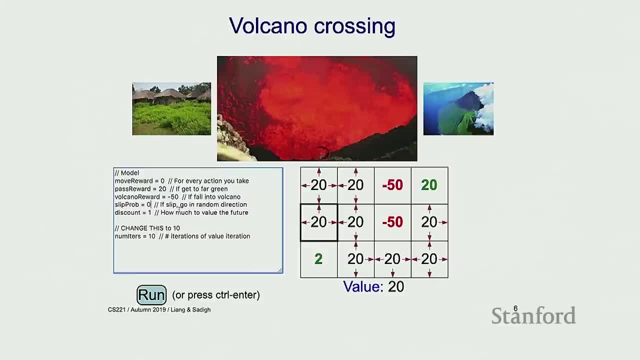 is stochastic and slip probability is not gonna be zero. Maybe, maybe it is 10 percent. So if there's 10 percent chance of falling into the volcano, how many of you would would still cross the island? Good number, So um. 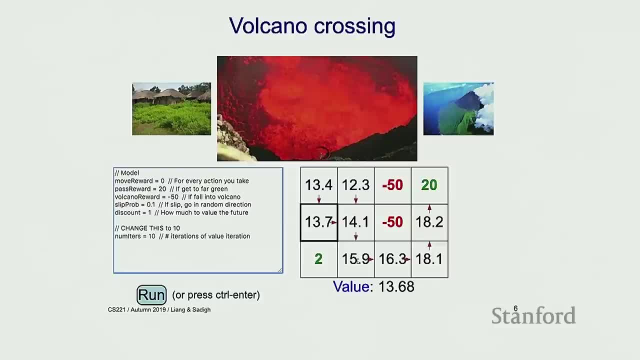 the optimal solution is actually shown by these arrows here And, yes, the optimal solution is still to cross the island, Like your value here we're gonna talk about all these terms, But the value here is basically the value you're gonna get. 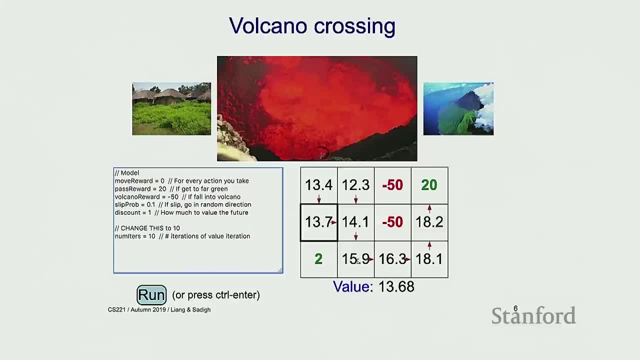 uh, at that beginning like state, which is the kind of we'll we'll talk about it. It's the expected utility that you're gonna get. It's gonna go down because there is some probability that you're gonna fall into a volcano. 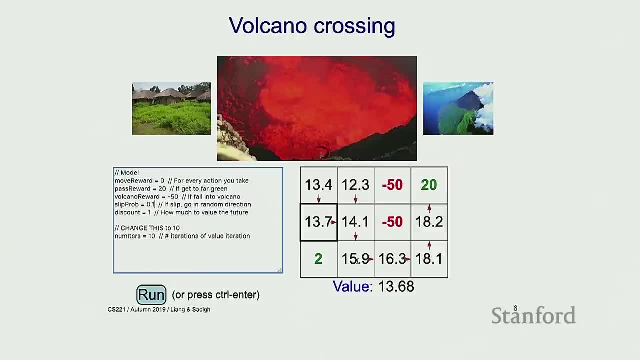 But still like the best thing to do is to cross the island. How about 20 percent? How many of you would do it with 20 percent? Some number of people, It's less. Um, still turns out that the optimal strategy is to cross 30 percent. 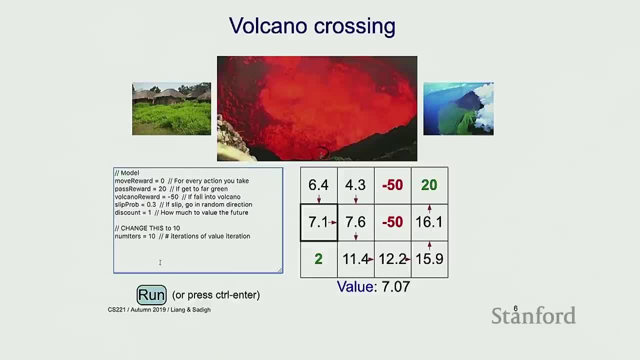 One percent. So with 30 percent, that's actually the point that you kind of you'd rather not not cross, because there is this volcano And then with a large probability you could, you could fall into the volcano and the value is going to go down. 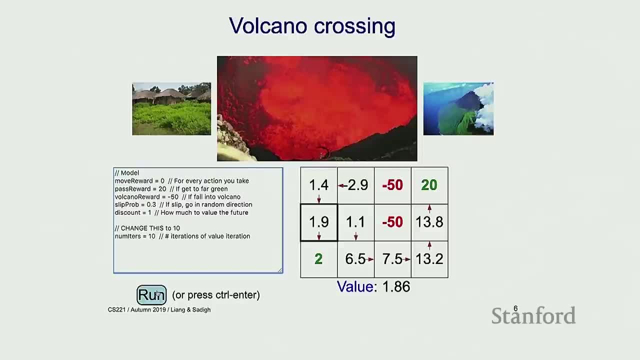 Okay. So these are the types of problems you're gonna- we're gonna- work with. Yes, Is the value like what you're spending in 2?? Because 2 is like what you can do, So 2 is like a value. 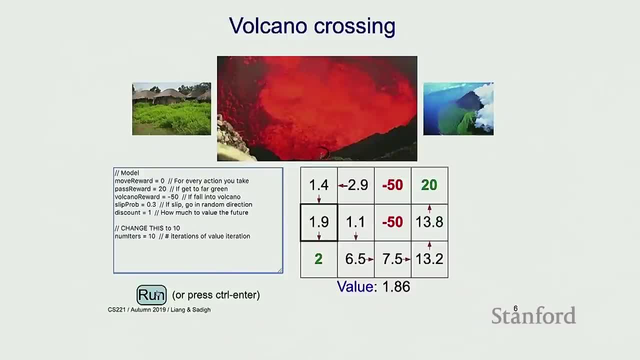 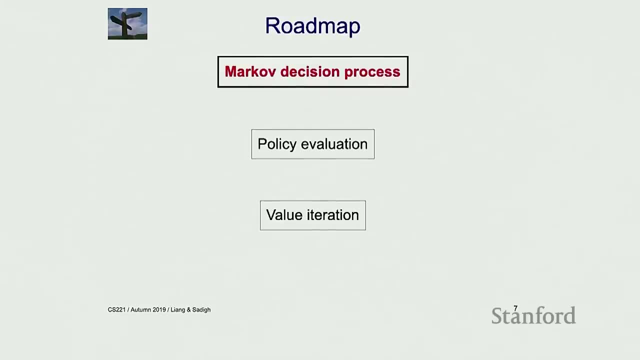 the reward that you're going to get at at that state and then, value you compute, that you propagate it back. We'll talk about that in details on on how to compute the value. Okay, All right. Okay, So that was just an example. 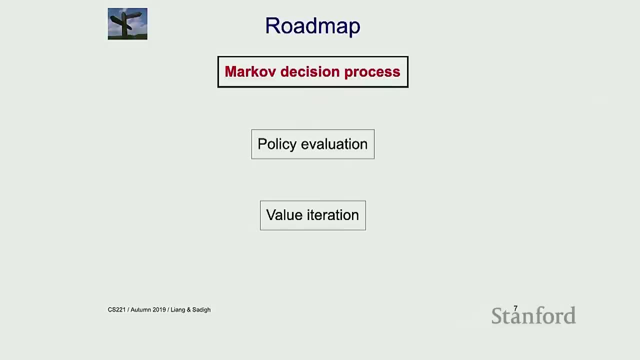 So so that was an example of a Markov decision process. What we want to do in this lecture is we're going to like again model these uh types of systems as Markov decision processes. Then we are going to talk about inference-type algorithms. 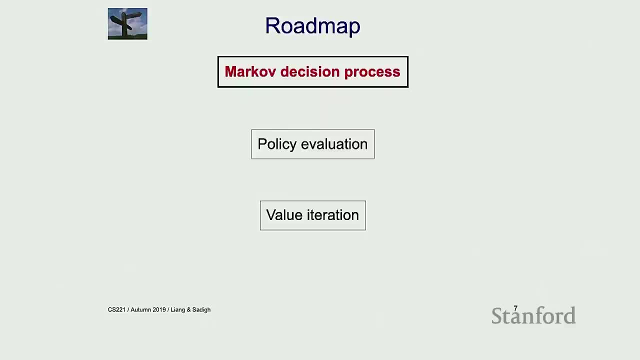 So how do we do inference? How do we come up with this best strategy path? Um, and in the middle I'm going to talk about policy evaluation, which is not an inference algorithm, but it's kind of a step towards it. 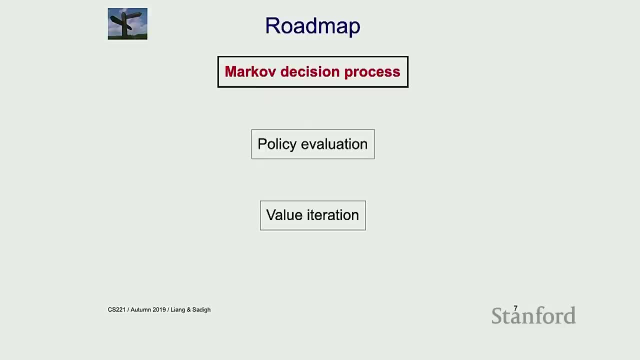 And it's basically this idea of: if someone tells me this is a policy, can I evaluate how good it is? And then we'll talk about value iteration, which tries to figure out what is the best policy that I can take. okay, So that's the plan for today. 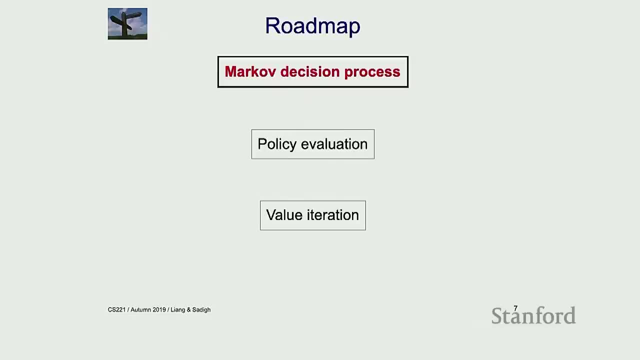 Then next lecture, we are going to talk about reinforcement learning, where we don't actually know what the reward is and we don't know what the, what the transitions are, Uh, so so that's kind of the learning part of part of this. uh, MDP lectures. 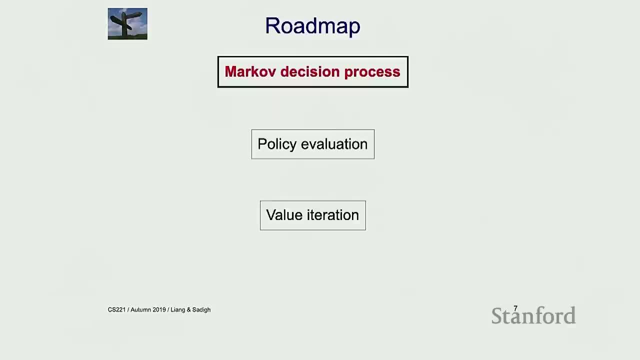 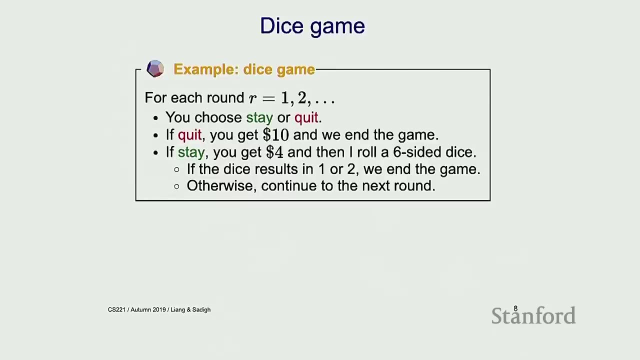 So Reid is going to actually do the do the lecture next next on on Wednesday, right, Okay? So let's get into. let's get into Markov decision processes. So we have a bunch of examples throughout this lecture. So let's look at another example. 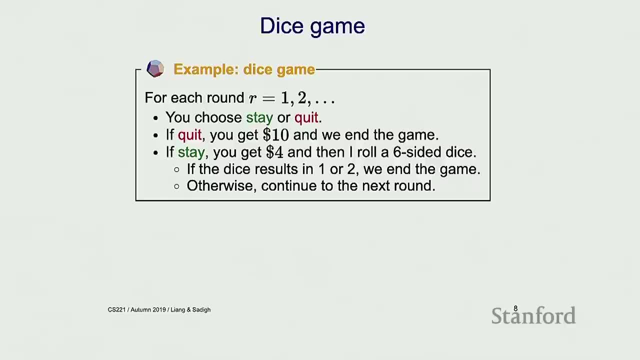 So all right. So actually I do need volunteers for this. So in this example, uh, we have a bunch of rounds And the idea is you can, at any point in time, you can choose two actions. You can either stay or you can quit. okay, 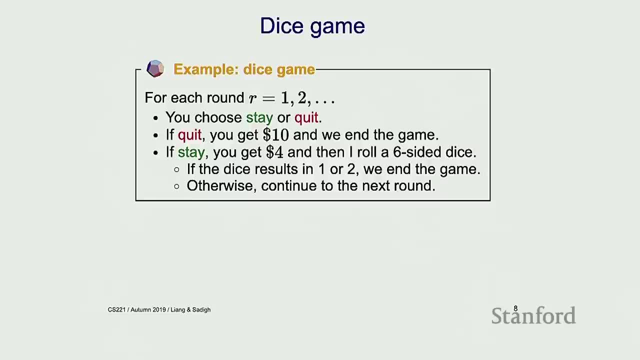 If you decide to quit, I'm going to give you $10.. I'm actually I'm not gonna give you $10, but imagine I'm gonna give you $10 and then we'll end the game, okay, And then if you decide to stay, 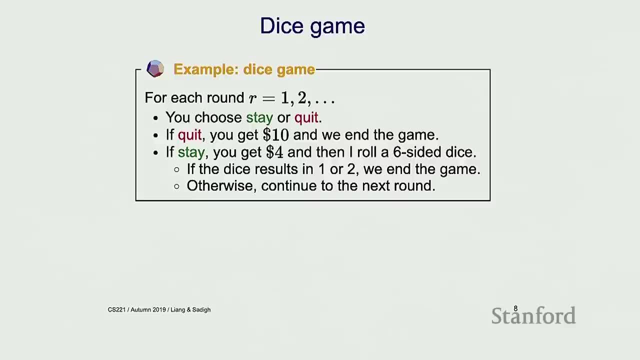 then you're gonna get $4 and then I'll roll the dice. If I get one or two, we'll end the game. Otherwise, you're going to continue to the next round and you can decide again. okay, So who wants to play with this? 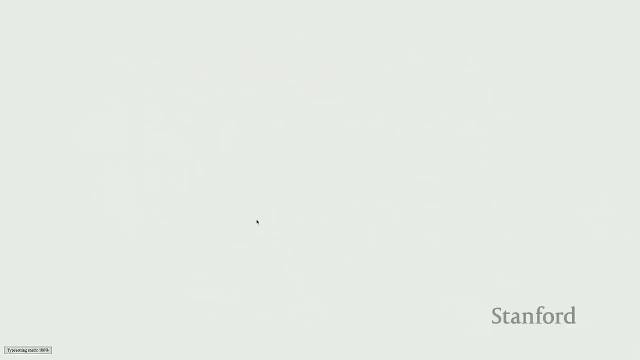 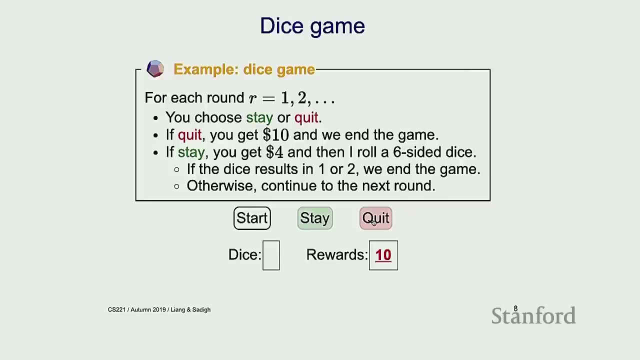 Okay, All right, Volunteer, Do you wanna stay or quit? Quit, So that was easy. You got your $10.. Is there anyone else on the way? Stay, Stay, Stay. Oh, you got eight, eight dollars. Sorry, The dice is two. 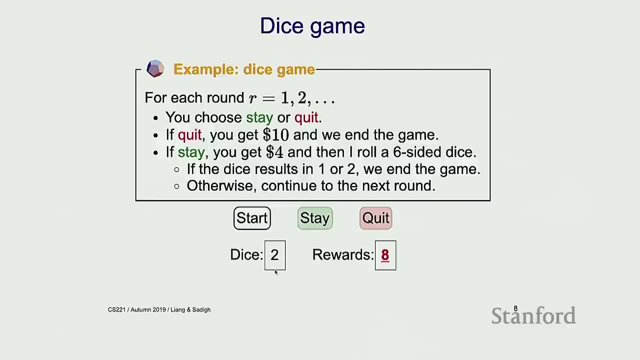 Um, so kind of, you know, I'm gonna give you $10.. I kind of get the idea here right. So, so you have these actions and then with one of them, like if you decide to quit, you deterministically will get your $10 and you're done. 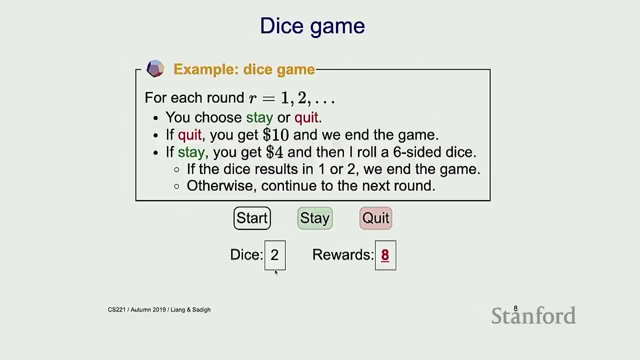 Uh, with the other one, it's it's probabilistic and you kind of wanna see which one is better and what. what would be the best policy to take in this setting? So we'll come back to this question, We'll formalize this and and we'll go over this. 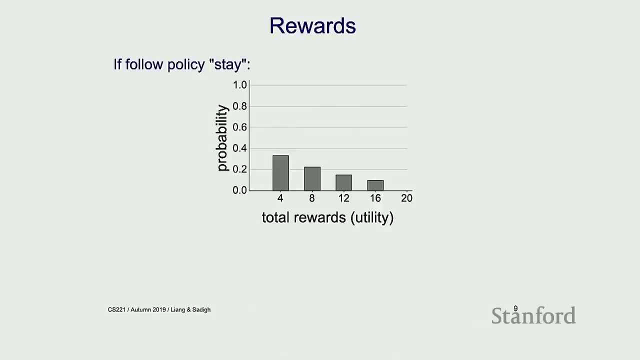 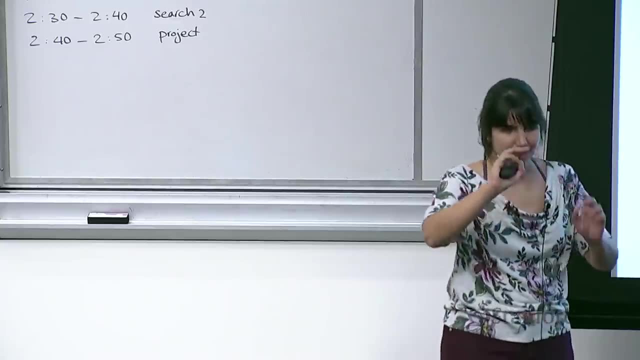 Always like, just continue once and then quit, Like isn't it better to switch, or So when, when, not okay, so, so then you need to actually compute what is the expected utility, right? So, and that's what we wanna do, right? 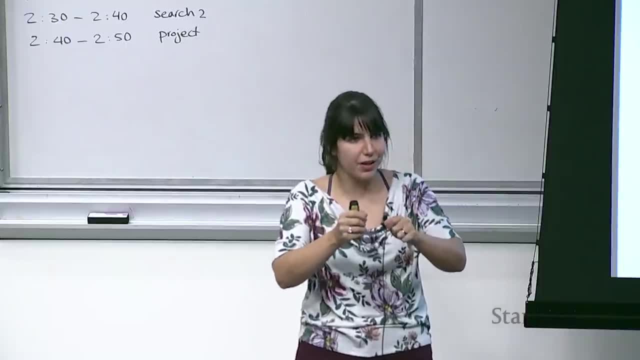 So so you might say, oh, I wanna, I wanna stay, and then I get my $4, and then I wanna quit, and then I get 14, and maybe that is the way to go. Um, that that could be a strategy. 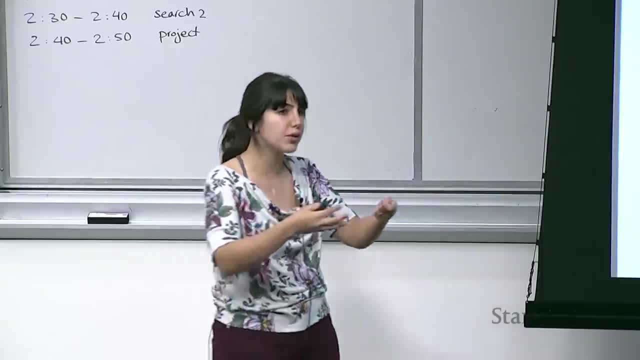 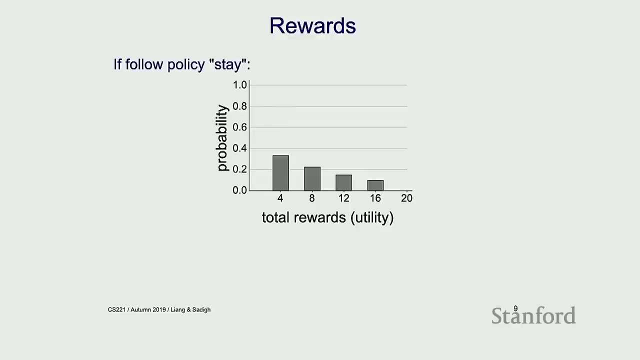 but for doing that right, like we are going to actually talk about that, For doing that, we are going to define what would be the optimal policy. One other thing that, uh, for this particular problem, we are going to keep in mind is: 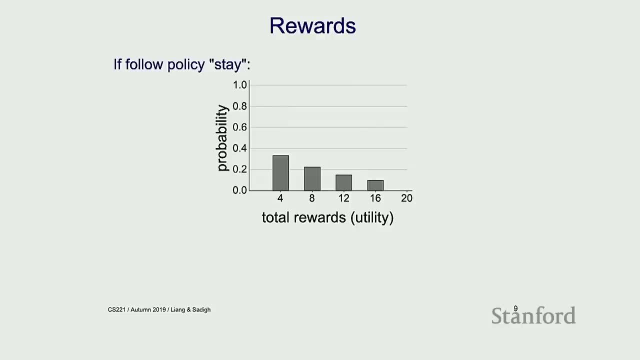 I'll. I'll talk about it when, when I define a policy. But. but the policy, the way we define it, is it's a function of state. So if you decide to stay, that is your policy. If you decide to not stay, that is your policy. 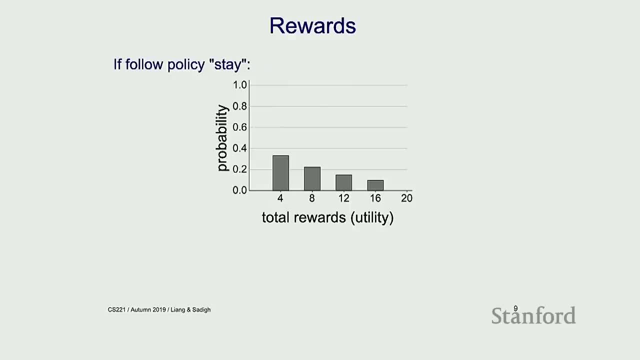 Like you're not allowing switching right now, like as I talk about this later in the lecture. But, but I'll come back to this problem, okay, So if you, if you decide that your policy, the thing you wanna do is to just stay, like, keep staying. 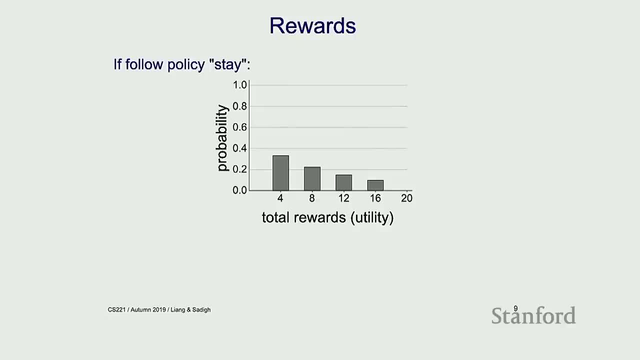 This is the probability of like the total rewards that you're gonna get. So you're gonna get four with some probability, And then, if you're lucky, you're gonna get eight And then, even if you're luckier, you're gonna get 12.. 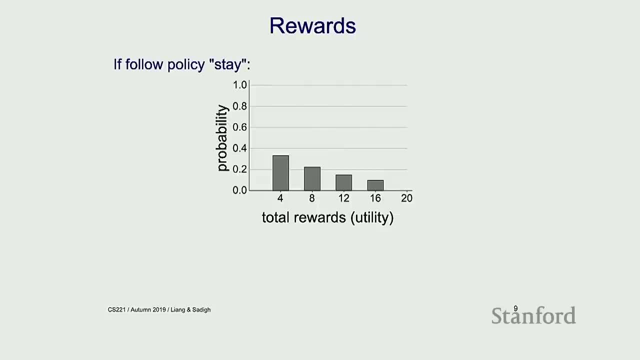 And if you're luckier you're gonna get 16.. But uh, but the probabilities are going to come down pretty much like really quickly. So the thing we care about in this setting is: is the expected utility, right? 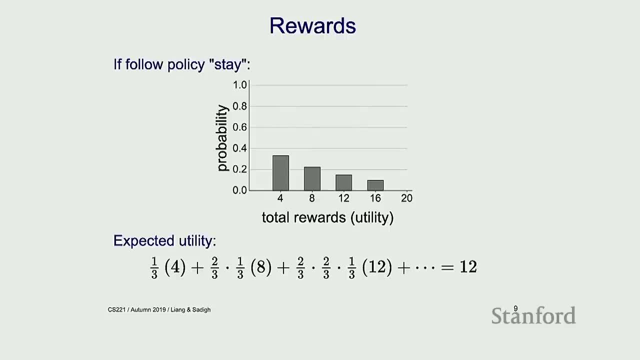 In expectation, like if I, if I, if I run this, if I average all these possible paths that I can do, what would be the value that I get? And for this particular problem, it turns out that, in expectation, if you decide to stay, 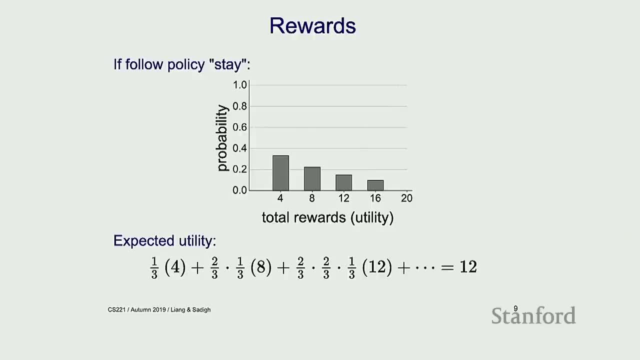 you should get 12.. So so you got really unlucky that you got eight, But but in general, in expectation, you should decide to stay okay, And then we actually wanna spend a little bit of time in this lecture thinking about how we get that 12,. 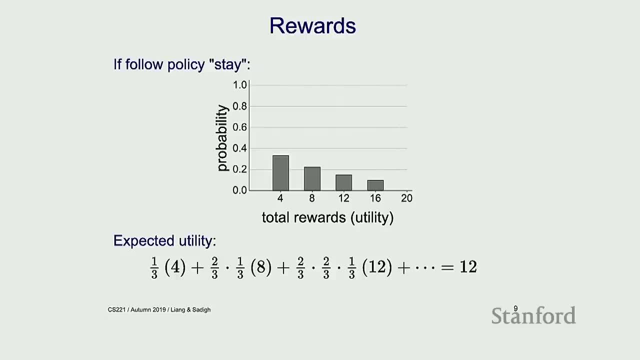 and then how to go about computing this expected utility And and, based on that, how to decide what policy to use, right, Okay, And then if you decide to to quit, then the expected utility there is kind of obvious, right. 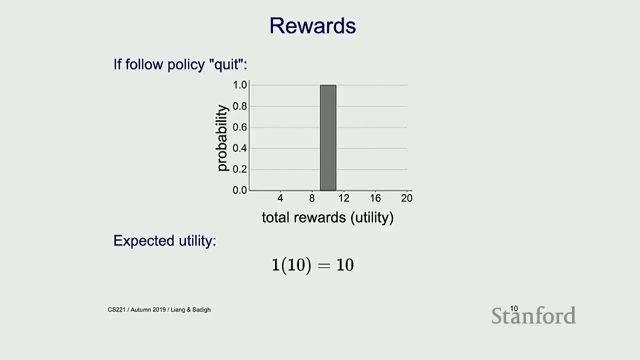 Because that that you're quitting, and that's your probability one, you're getting $10.. So you're just gonna get $10 and that is the expected utility of quitting. So when you, when I said, when you roll a die, 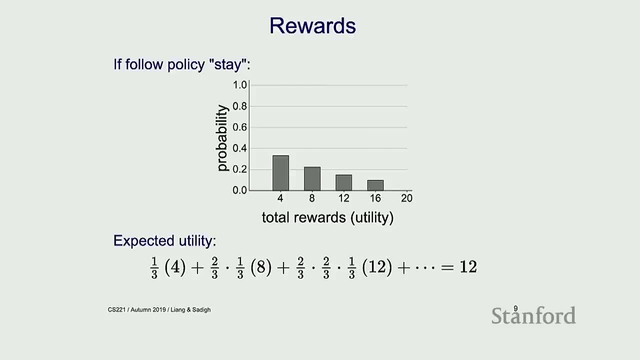 I said, if you get one or two, you, you, you say yeah, And then if you get the other, so the two-thirds of it, you continue. So so it's a one-third. two-third comes from there, okay. 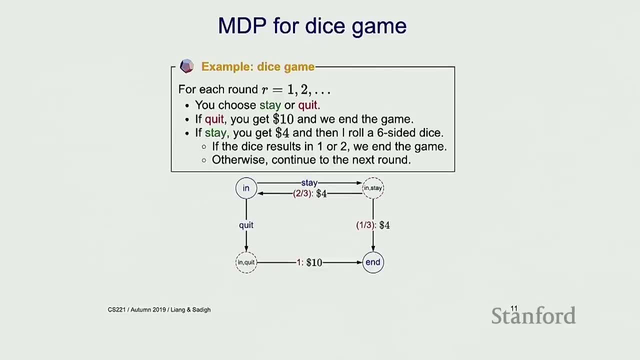 All right, I'll, I'll come back to this example. This is actually the the running example throughout this lecture. okay, So you're going to talk about that. That's what the lecture is about. Okay, So let's, let's actually. 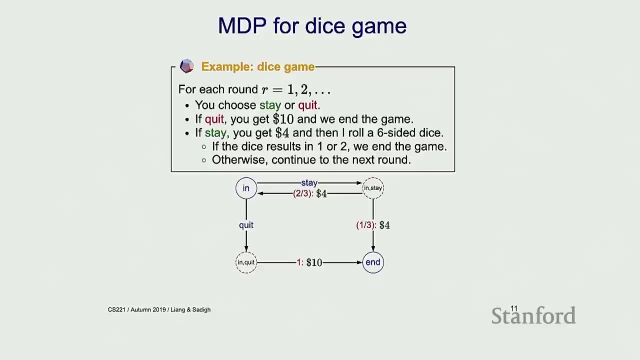 I do want to finish in an hour. That's why maybe I'm rushing things a little bit, But we are going to talk about this problem like throughout the class, So so don't worry about it If it's not clear at the end of it. 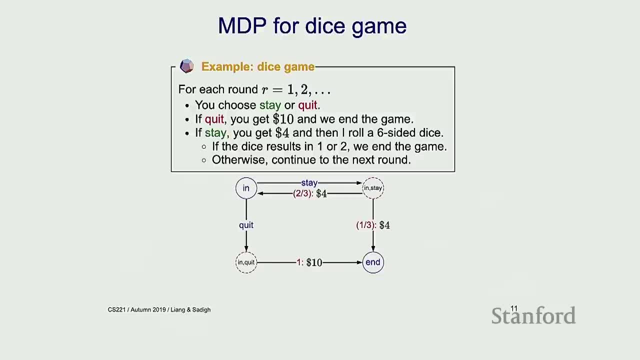 we can clarify things, okay, All right, So I do want to formalize this problem. The way I want to formalize this problem is using an MDP, So I want to. I want to formalize this as a as a Markov decision process. 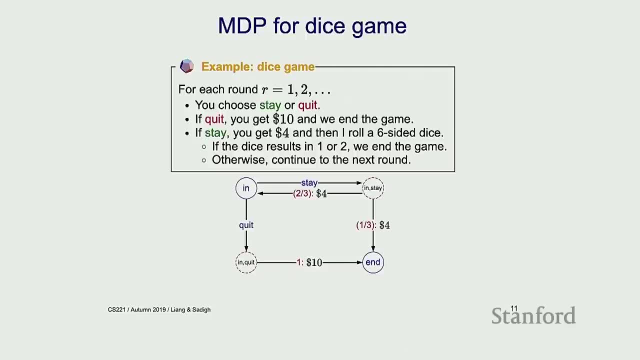 Maybe I can just use this. So in Markov decision processes, similar to search problems, you're going to have states. So in this particular game I'm going to have two states. I'm either in the game or I'm out of the game. 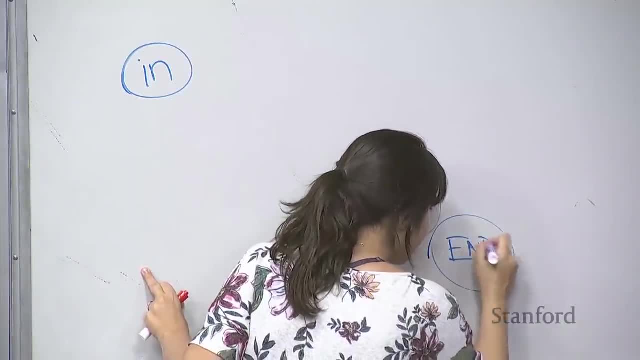 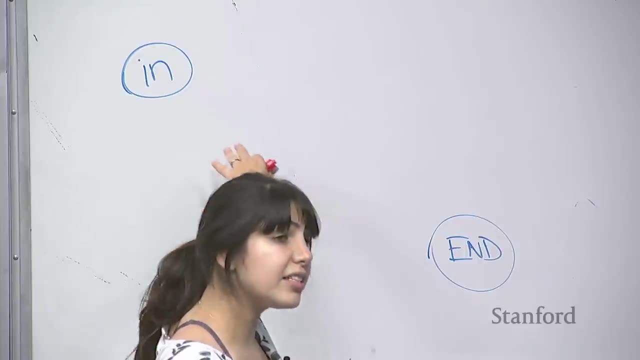 So I'm in an end state where everything we ended, you're out of the game, you're done, Okay, So so those are my states Then. um, when I'm in these states, I'm in each of these states. 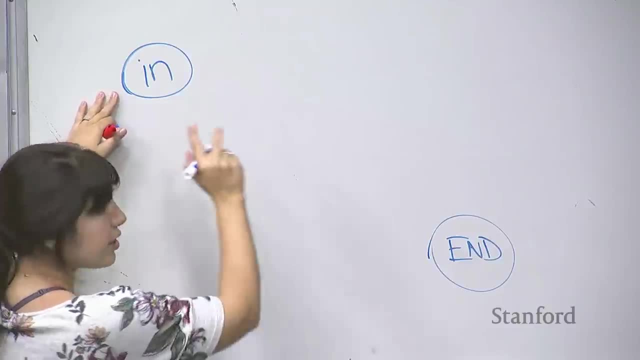 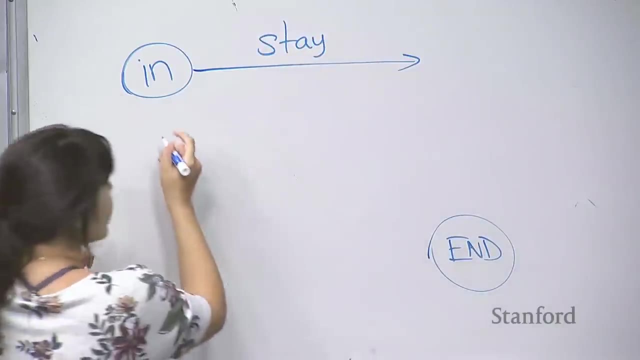 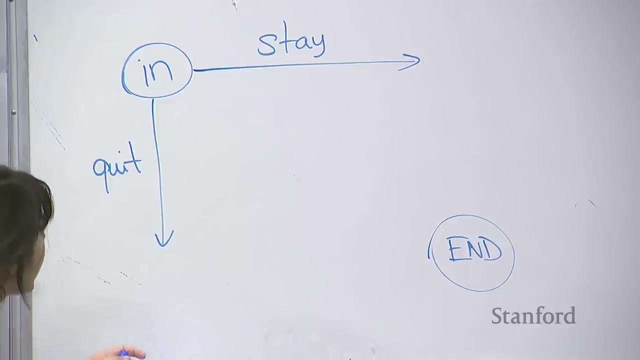 I can take an action. And if I'm in an end state, I can take two actions. right, I can either decide to stay right Or I can quit. Okay, And if I, if I decide to stay from end state, 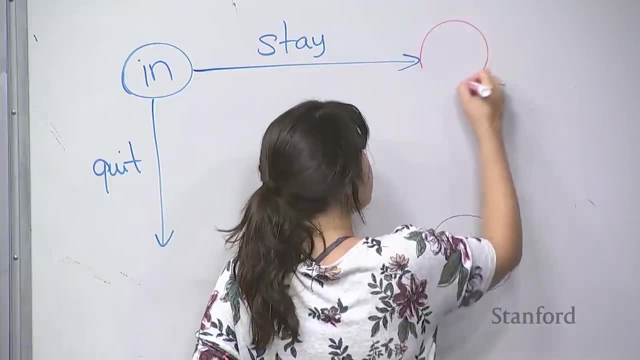 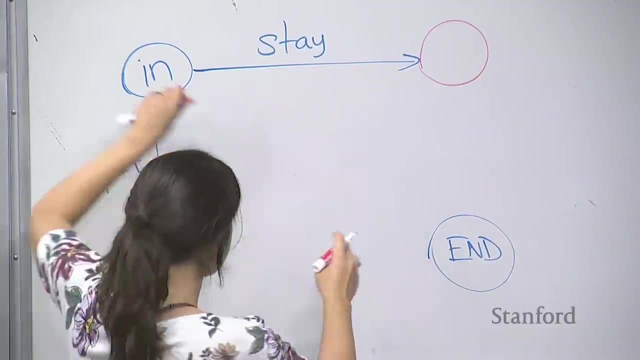 that takes me to something that I'm going to call a chance node. So a chance node is a node that represents state and action. So it's not really like the blue things are my states, but I'm creating these chance nodes as a way of kind of going. 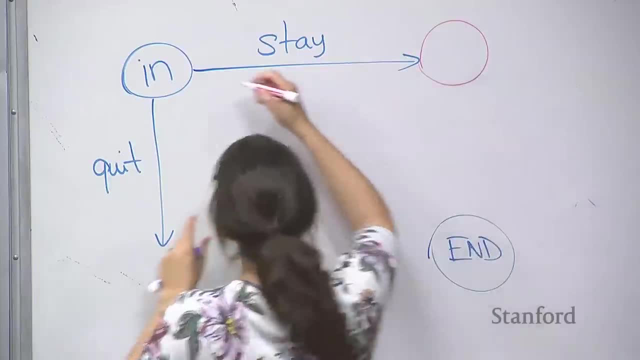 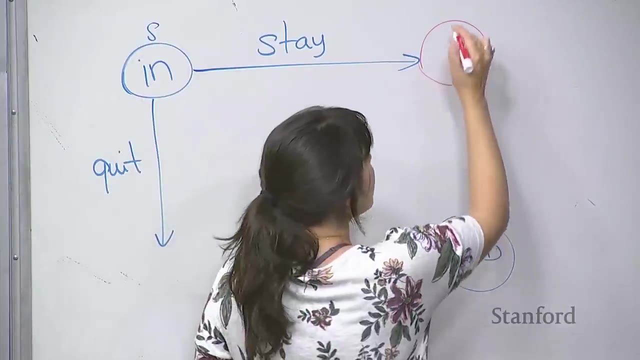 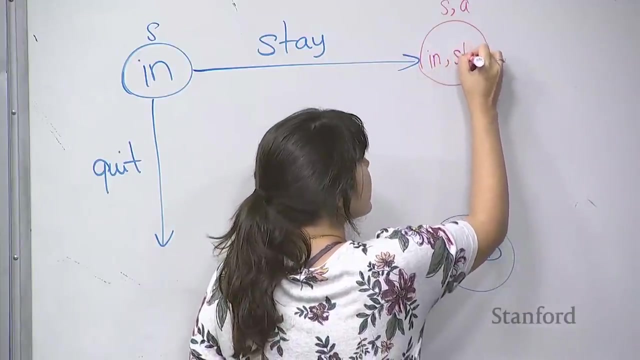 through this example to to see where things are going. So so these, these blue states are going to be my states. I'm in S. These chance nodes are over state and action. So, basically, this node tells me that I started with n and I decided to stay. 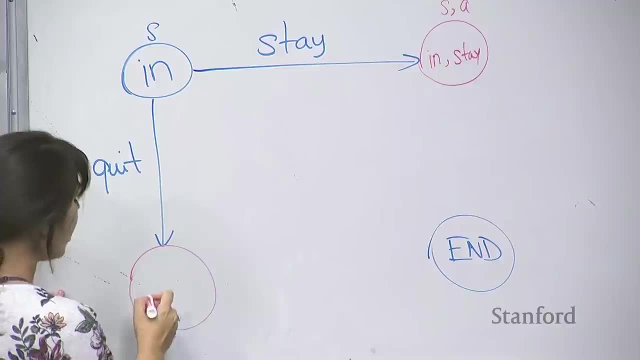 Okay, And a chance node here basically tells me that I started with n and I decided to quit. Okay, Yes, in this case no, even though it's deterministically. So I deterministically go there. but then, from the chance node, 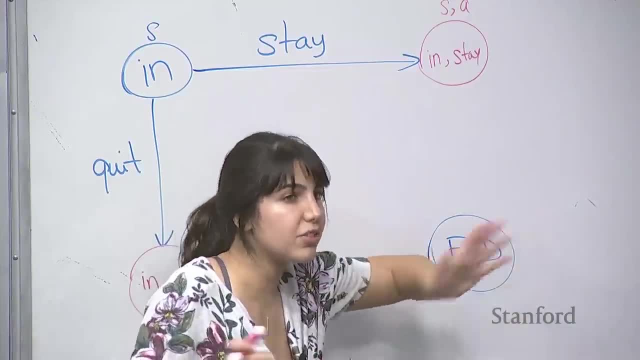 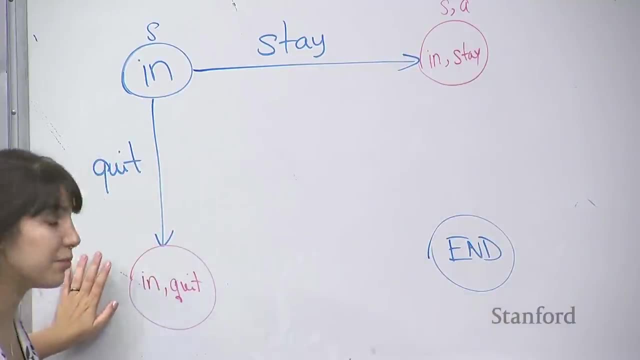 that's where I'm introducing the probabilities. So from the chance node I can like probabilistically end up in these different states. In the case of quit, it's also deterministic. In the case of the quit. in this case it's deterministic. 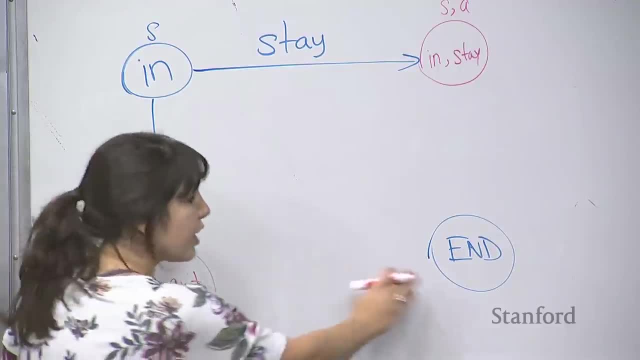 Yeah. So in the case of the quit, you'll say probability one. I'm going to end up in this end state. So I'm gonna draw that with the no, uh no with the with the edge that comes from my chance node. 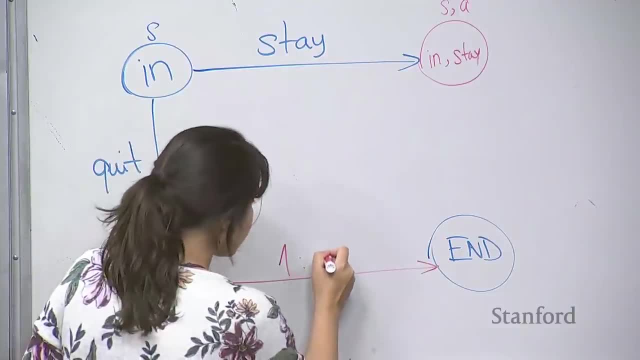 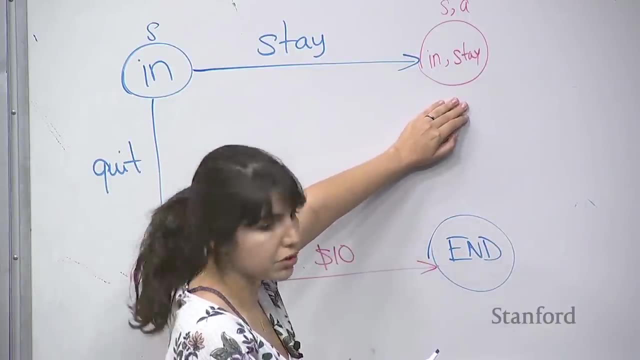 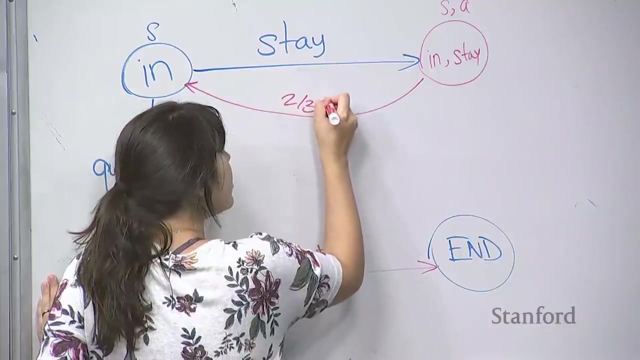 And I'm gonna say, with probability one, I'm going to get $10 and just be done Okay. But if you're in this state- this is actually the state where interesting things can happen- With probability two-thirds- I'm going to go back to in and get $4.. 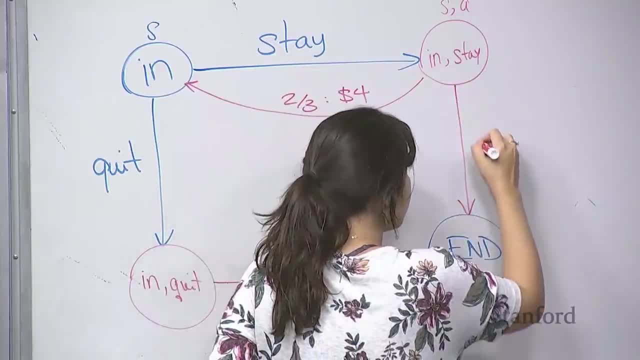 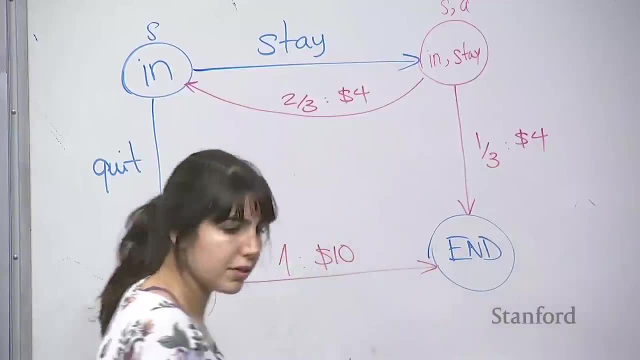 Or, with probability one-third, I'm going to end up in end And I get still $4, okay, So so that is my Markov decision process. So so I had. maybe you can keep track of a list of things you're defining in this lecture. 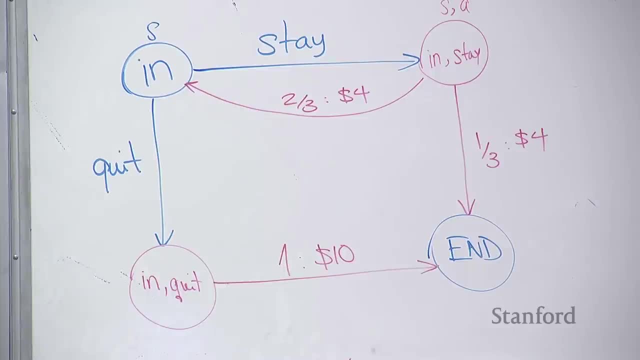 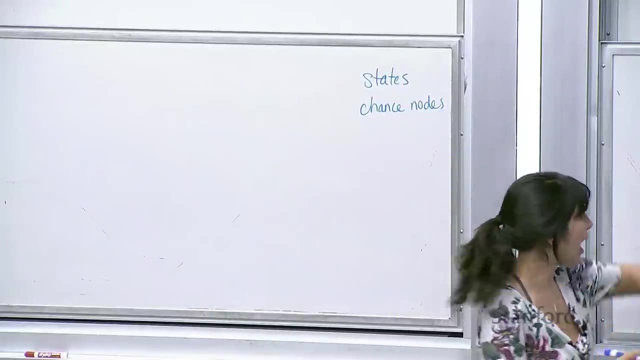 So we just define states. And then we said, well, we're gonna have these chance nodes, because from these chance nodes, probabilistically we're going to come out of them, depending on what happens to nature. right, Like I end up, this is the decision I've made. 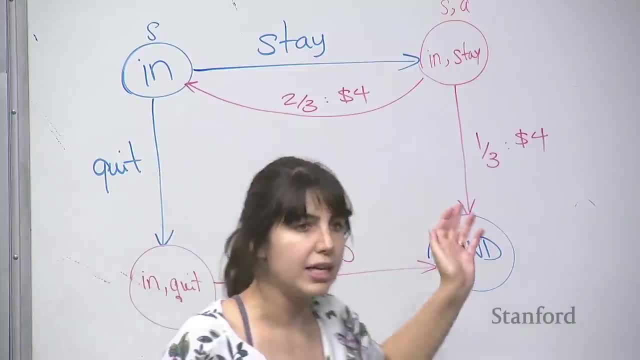 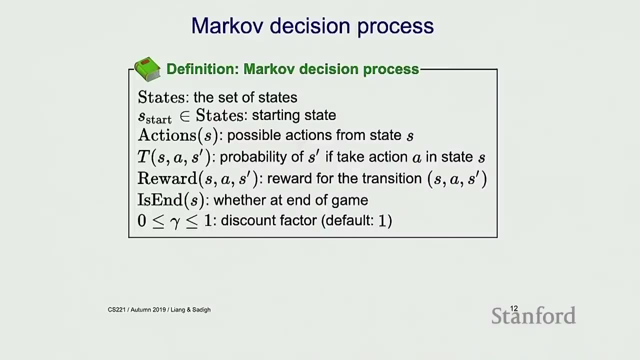 Now nature kind of decides which one we are gonna end up at and and based on that, we we move forward. okay, All right. So so more formally, we have a bunch of things when we define an MDP Similar to search problems, we 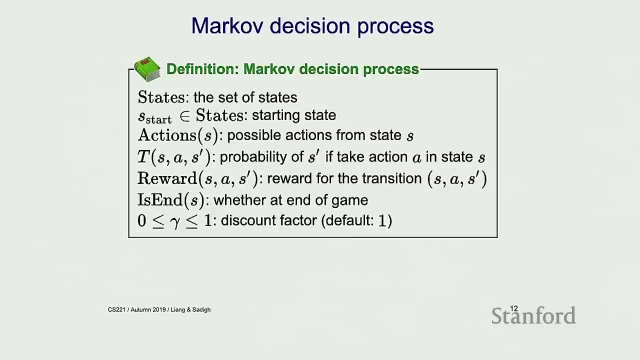 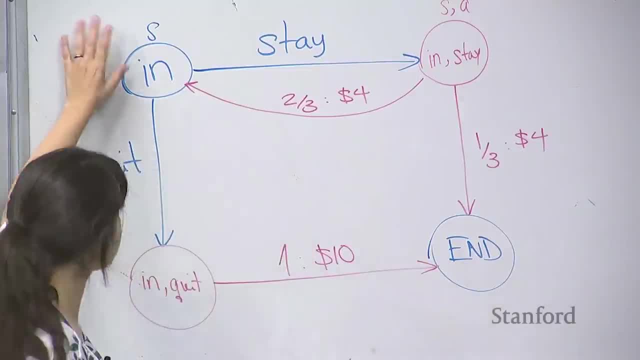 like we, we now need to define the same set of things. So so we have a set of states. In this case, my states are in and end. okay, We have a start state I'm starting with in, so that's my start state. 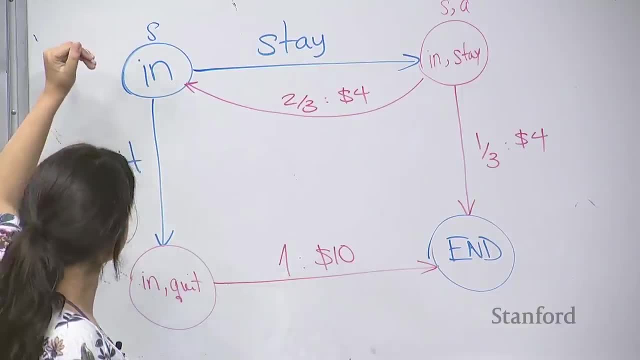 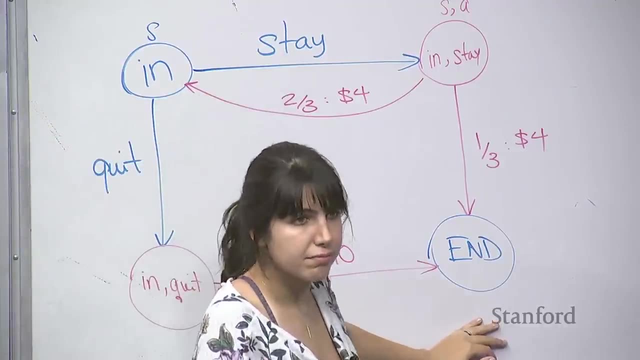 I have actions as a function of states. So when I ask what are the actions of the state? my actions are going to be stay or quit? What are actions of end? I don't have anything right. End state doesn't have any actions that come out of it. 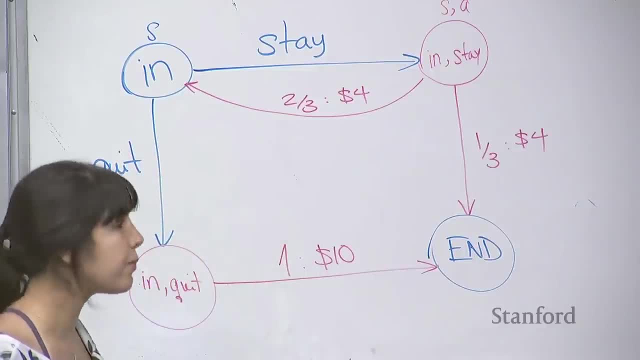 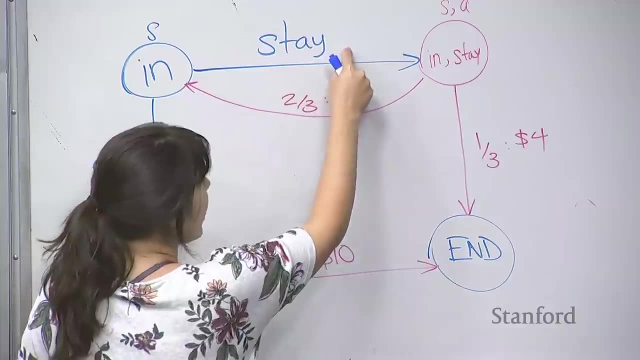 And then we have these transition probabilities. So transition probabilities: more formally: take a state, an action and and a new state, so S A S prime and tell me what is the transition probability of that? It's one-third in this case. 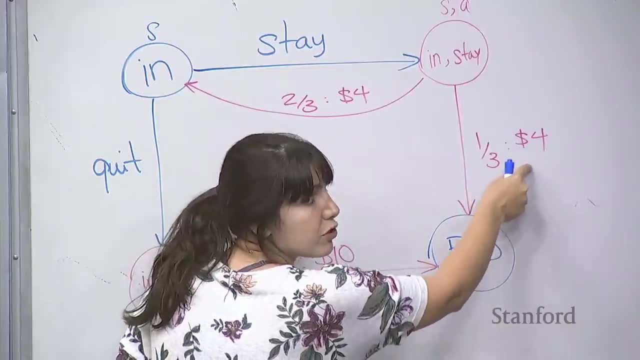 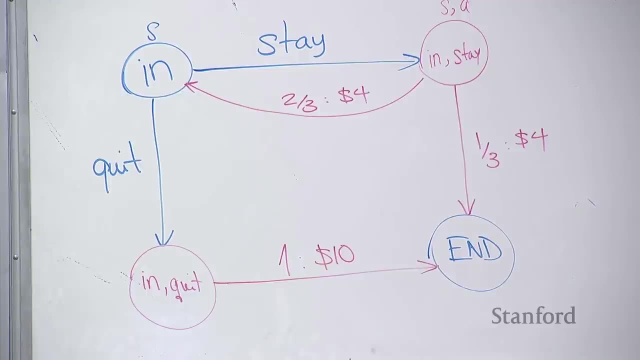 And then I have a reward which tells me how much was that rewarding? that was $4, okay, So, so I'm defining, so when I'm defining my MDP, kind of the new things I'm defining, is this transition probability? 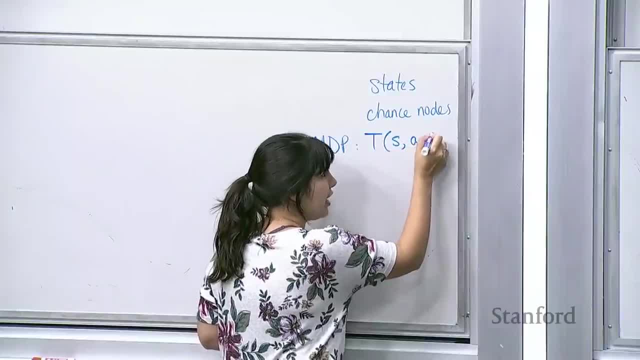 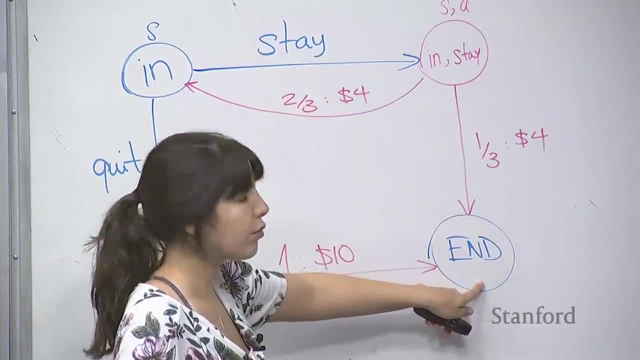 which tells me: if you're in state S and take action A and you end up in S prime, what is the probability of that? I'm in, in, I decide to stay and then I end up in end. What's the probability of that? 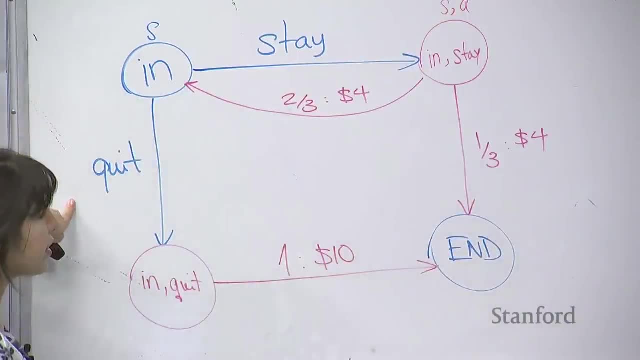 That's one-third, Maybe I'm in in, I decide to quit, I end up in end. What's the probability of that? That's equal to one, okay, And then over the same state, action state primes like next states we are going to end up at. 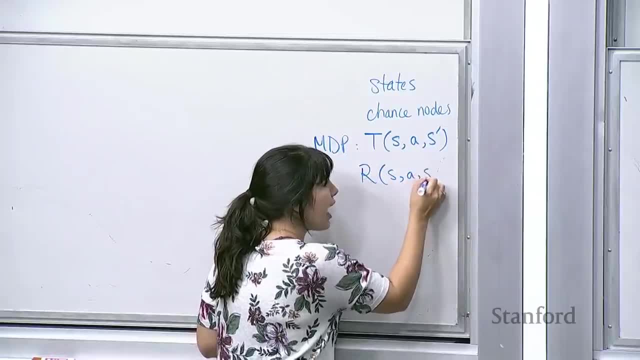 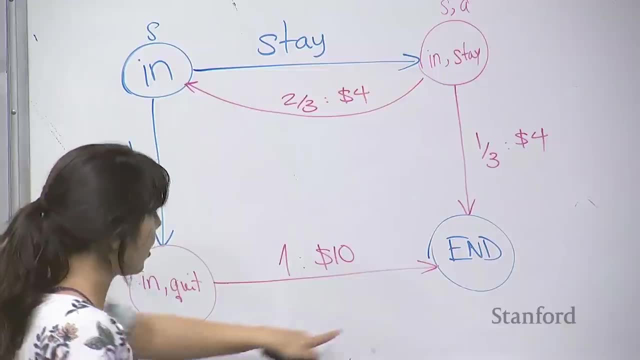 we are going to define a reward which tells me how much money did I get? or like, how, how good was that? So it was $4 in this case. or or, if I decide to quit, I got $10, okay. 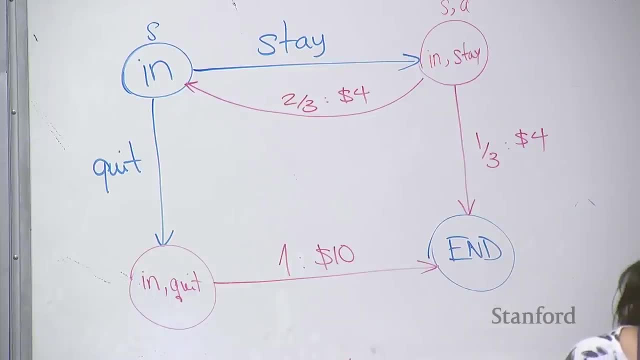 Um, and if you remember, in the case of search problems we were talking about cost. I'm just flipping the sign. here We wanted to minimize cost, Here we want to maximize the reward. It's just a more optimistic view of the world, I guess. 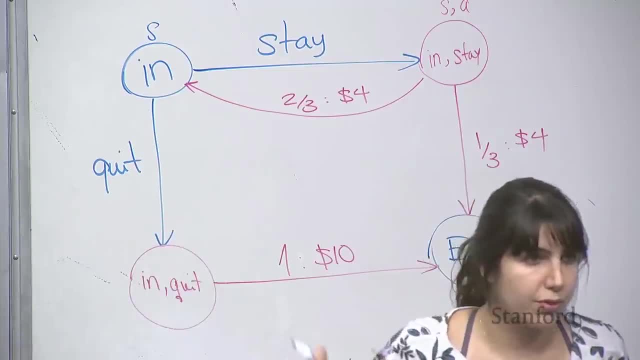 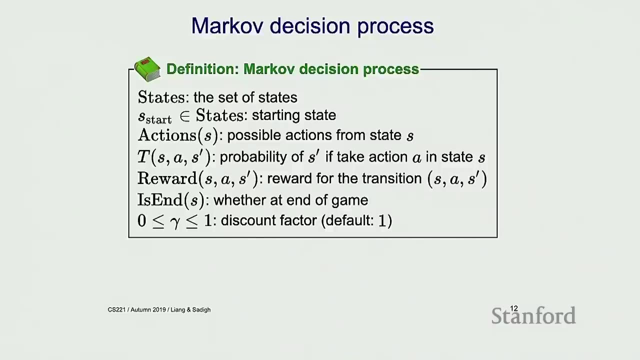 Um, so, so that is what the rewards are going to be defined on. okay, We also have- this is end function which, again similar to search problems, just checks if you are in an end state or not. And in addition to that, 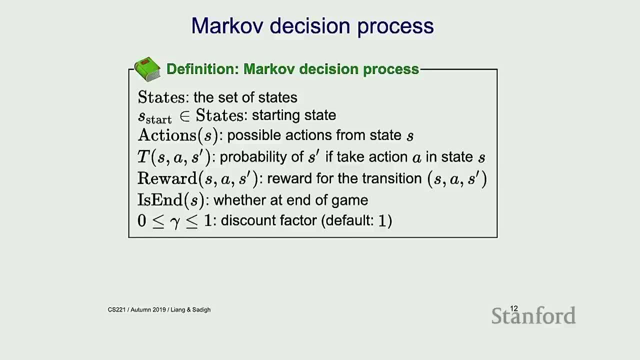 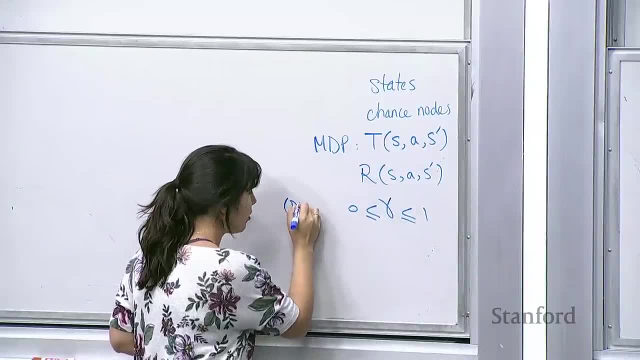 we have something that's called a discount factor. It's it's this value gamma, which is between 0 and 1.. And I'll talk about this later. Don't worry about it right now, But it's a thing we define for our search prob- for our MVPs. okay, 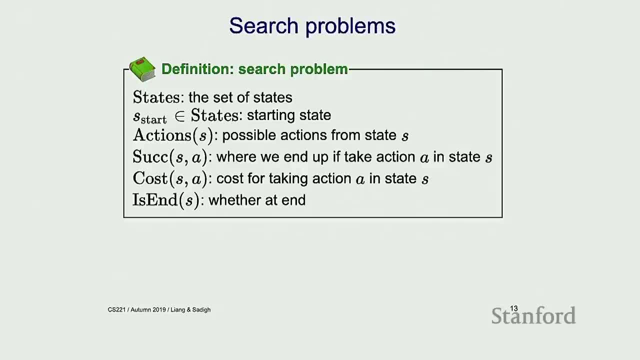 All right. So how do I compare this with search? Again, these were the things that we had in a search problem. We had the successor function that would deterministically take me to S prime, And we had this cost function that would tell me what was. 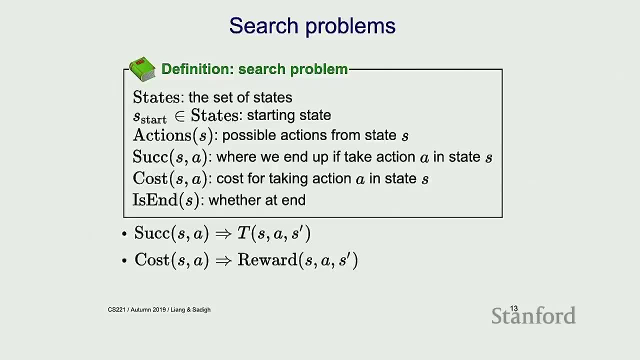 the cost of being in state S and taking action A. So so the major things that are changed is that, instead of a successor function, I have transition probabilities, these Ts that that basically tell me what's the probability of starting in S. 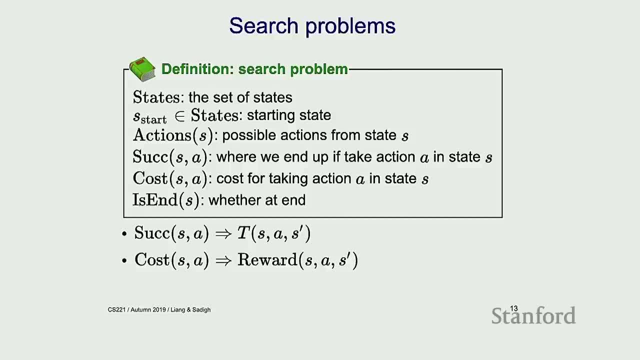 taking action A and ending up in S prime, And then the cost just became reward, okay, So. so those are kind of the major differences between search and MDP, because things are, things are not deterministically okay, All right, So so that was the formalism. 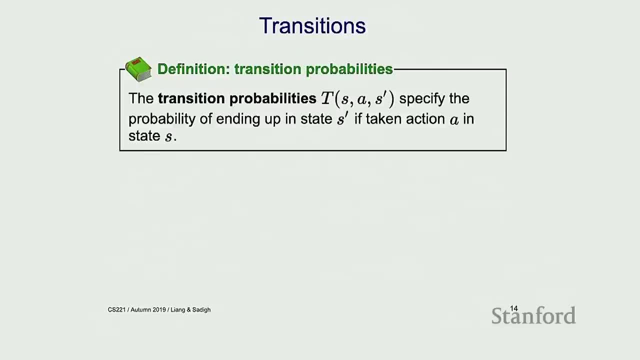 Now, now I can define any, any MDP model, any Markov decision process. And then one thing, just one thing to point out is this: transition probabilities. this T basically specifies the probability of ending up in in state S prime if you take action A in state S. 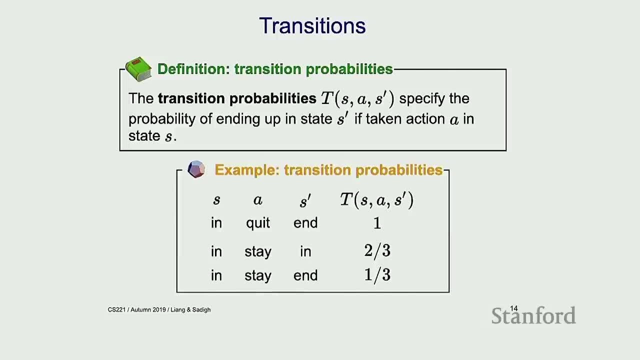 So so these are probabilities right. So so, for example, again, like we have done this example, but let's just do it on the on the slides again: If I'm in state N, I take action, quit, I end up in end. what's the probability of that? 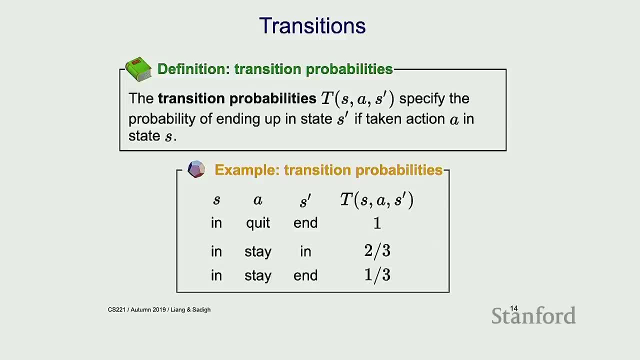 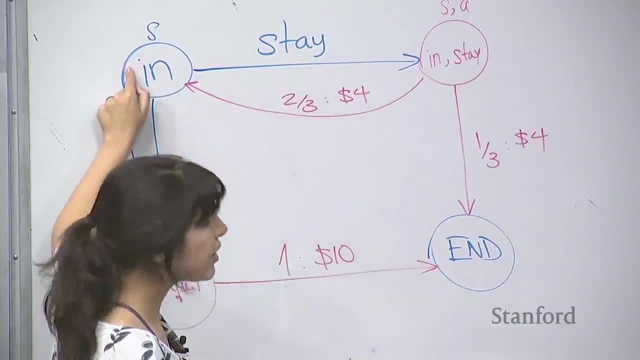 One And then, if I'm in state N, I take action stay. I end up in state N again. what's the probability of that? I ended up in N again two-thirds And then, if I'm in state N, I take action stay. 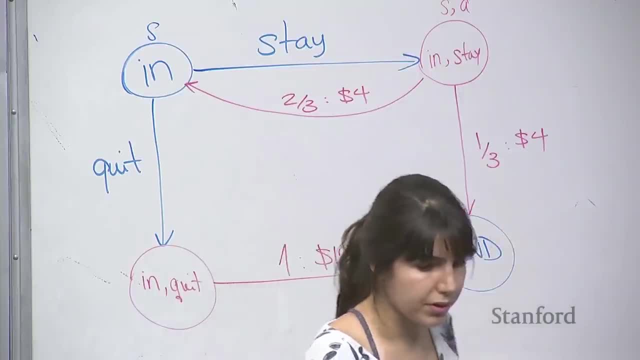 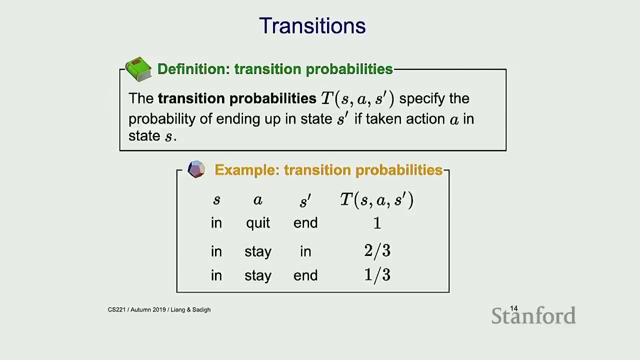 I end up in N. what's the probability of that? One-third, Okay, And, and these are probabilities. So what that means is they need to kind of add up to one. But one thing to notice is: well, just what is gonna add up to one. 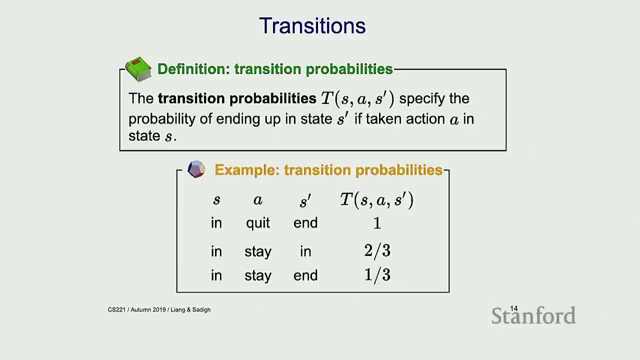 Like, like, all of the things in the column are not gonna add up to one. The thing that's going to add up to one is, if you consider all possible these different S primes that you're going to end up at, those probabilities are gonna add up to one. 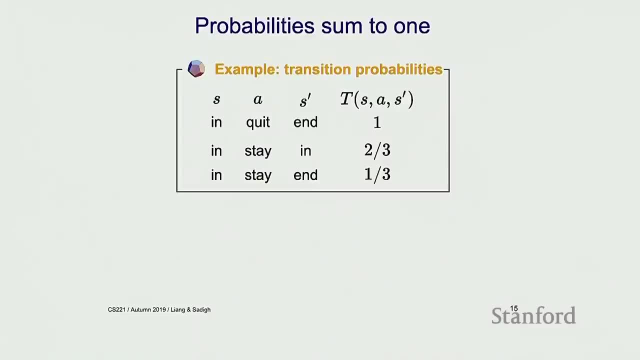 So. so if you look at this, this, uh, this table again, if you look at deciding and being in state N and taking action state, then the probabilities that that we have for different S primes are two-thirds and one-third. 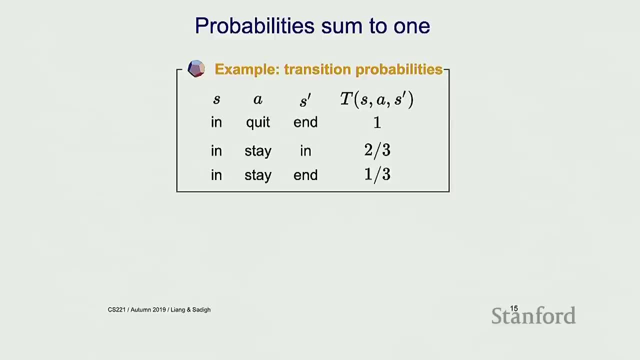 and those two are the things that are gonna add up to one, And, in the first case, if you're in state N and you decide to quit, then wherever, whatever S primes you're gonna end up at, in this case it's just N state. 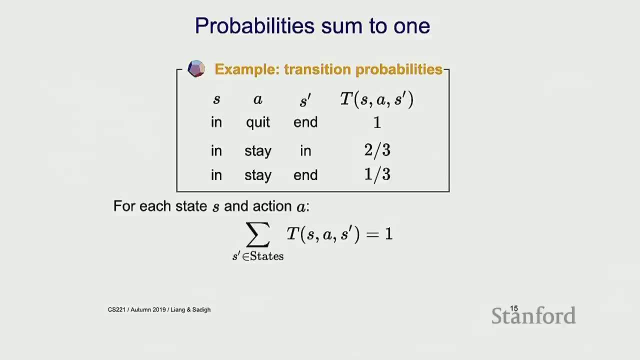 those probabilities are gonna add up to one, So so, more formally, what that means is, if I'm summing over S primes, these new, new states that I'm gonna end up at, the transition probabilities need to add up to one, okay. 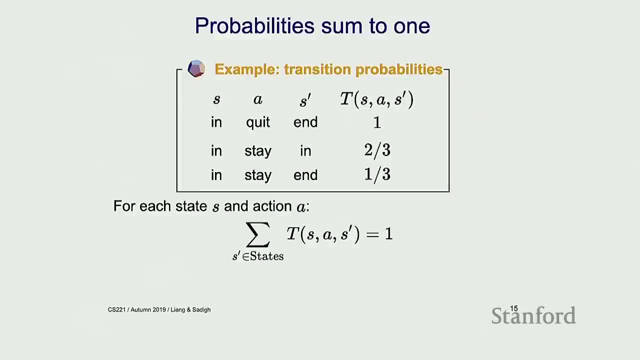 Because they're basically probabilities that tell me what are the, what are the things that can happen if I take an action, okay, And then, uh, this transition probabilities are going to be, uh, non-negative, because they are probabilities. So that's also another property, okay. 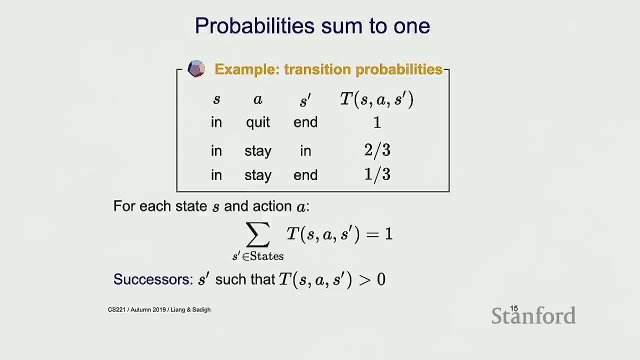 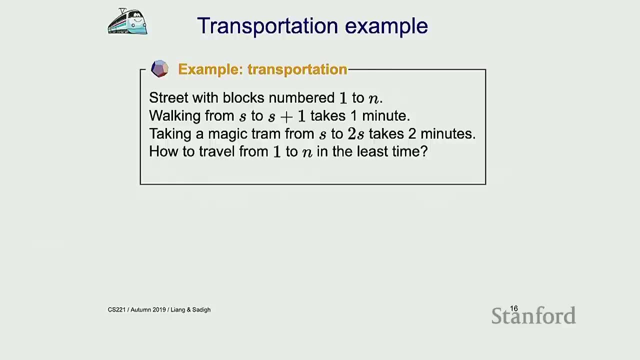 So usual things, All right. So so that's a search problem. Let's actually formalize another search problem. This is: uh, let's actually try to code this up. Uh, so what is this search problem? This is the tram problem. 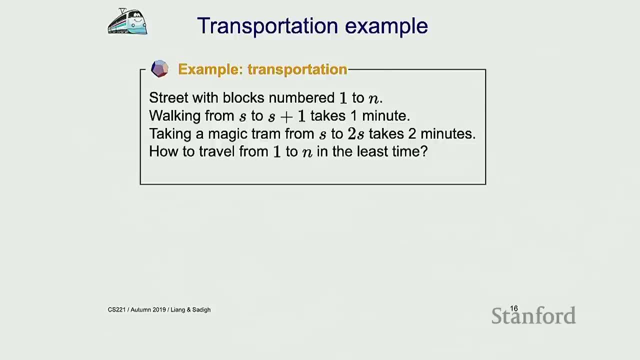 So, remember the tram problem. I have blocks, one through N. What I wanna do is, uh, I have two possible actions. I can either walk from state S to state S plus one, or I can take the magic tram that takes me from state S to state 2S. 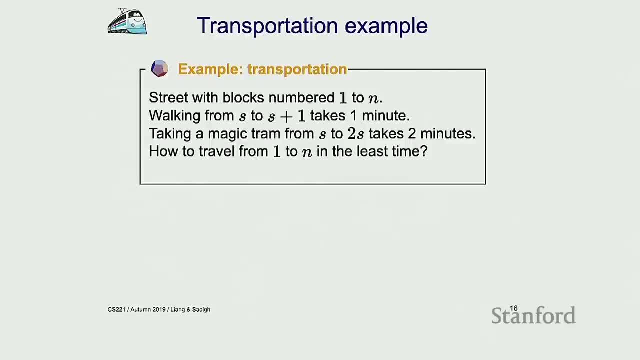 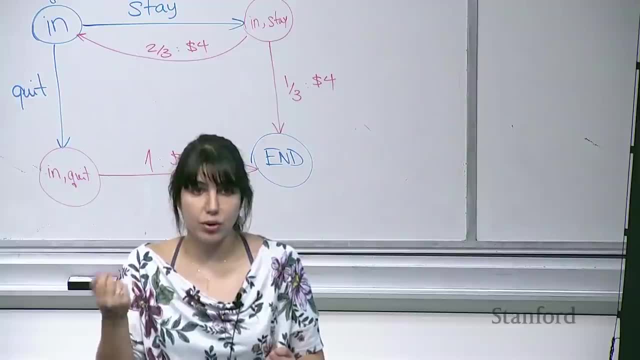 If I walk, that costs one minutes. okay, Means, reward of that is minus one. If I, if I take the tram, that costs two minutes. Uh, that means that the reward of that is minus two, Okay, Uh. and then the question was how? 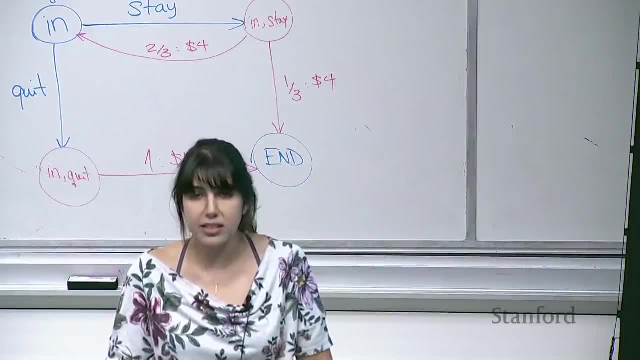 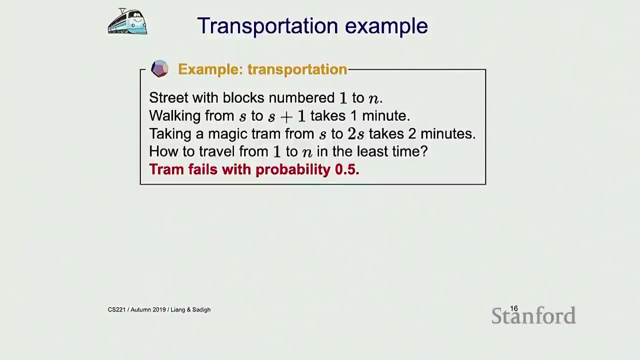 like: how do we wanna travel from from one to N in in the least amount of time? So so nothing here is is probabilistic yet right? So I'm gonna add an extra thing here, which says the tram is going to fail with probability 0.5. 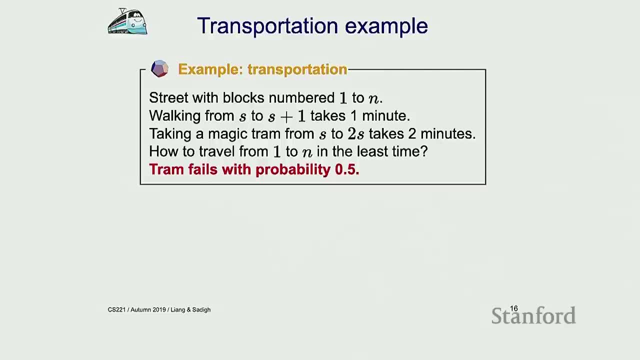 So I'm gonna decide, maybe take take a tram at some point and that tram can can fail with probability 0.5. If, if it fails, I end up in my state Like I don't go anywhere And and actually like in this case, 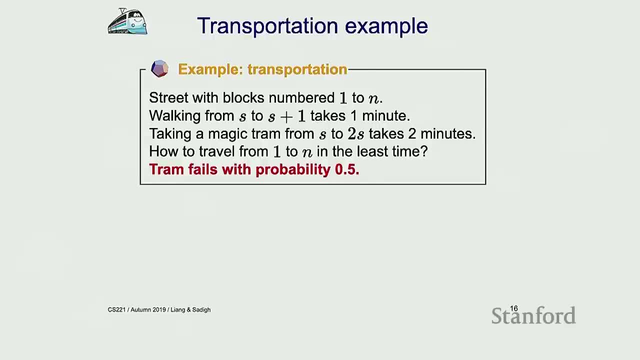 you're assuming you're still losing two minutes. So if I decide to take the tram, I'm gonna lose two minutes. Maybe it'll fail, maybe it will not. Okay, All right, So let's try to formalize this. So we're gonna take our tram problem from two lectures ago. 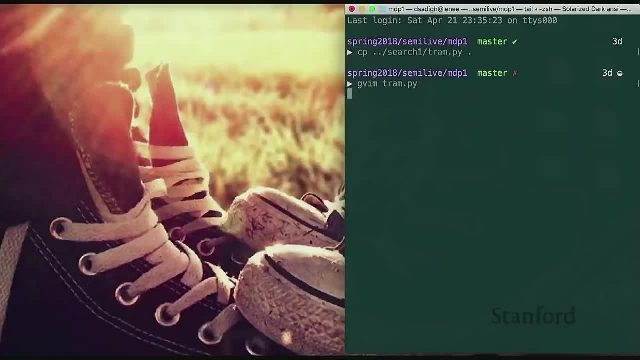 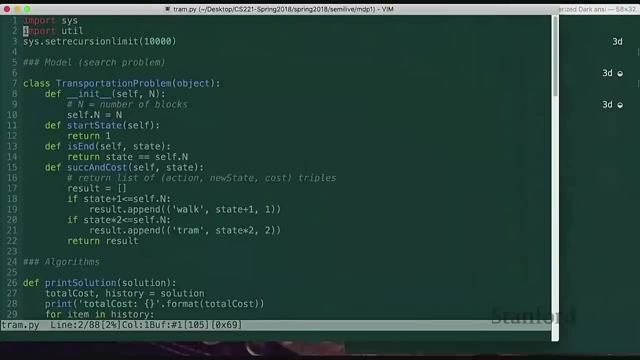 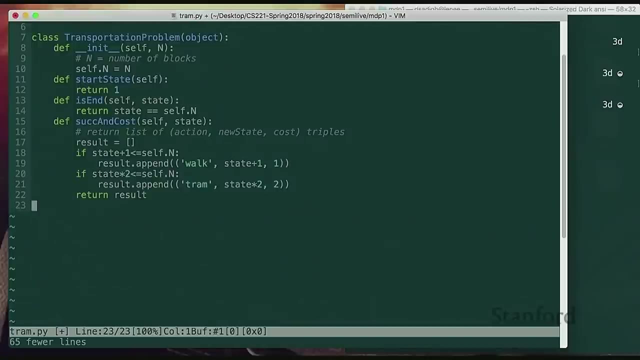 So this is from search one. We're gonna just copy that, So all right. So this was what we had from last time. We had this transportation problem and we had all these like algorithms to solve the search problem. We don't really need them because we have a new problem. 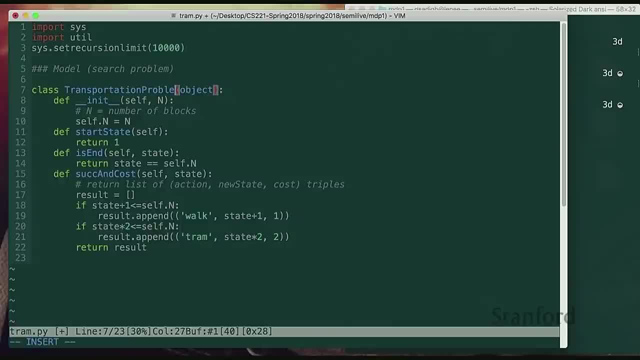 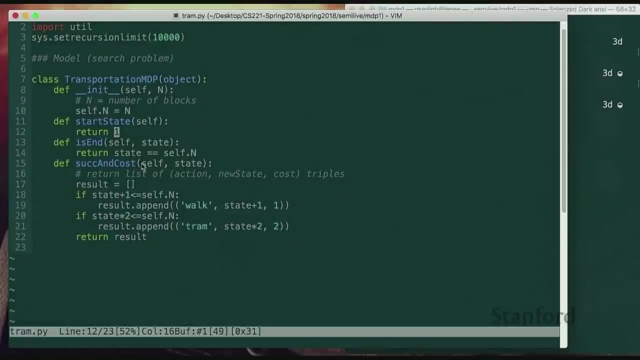 So let's just get rid of them. And now I just want to formalize an MDP. So so it's a transportation MDP, okay. The initialization looks okay. Start state looks okay. I'm starting from one Is end looks okay. 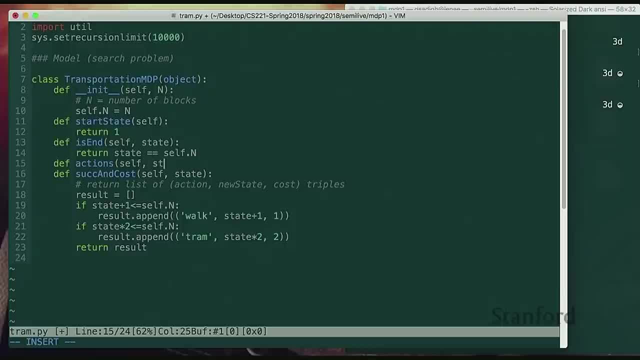 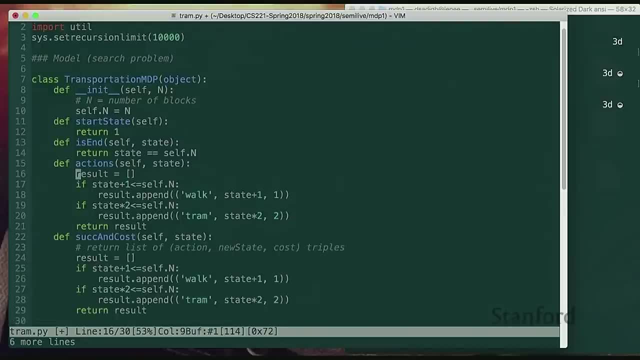 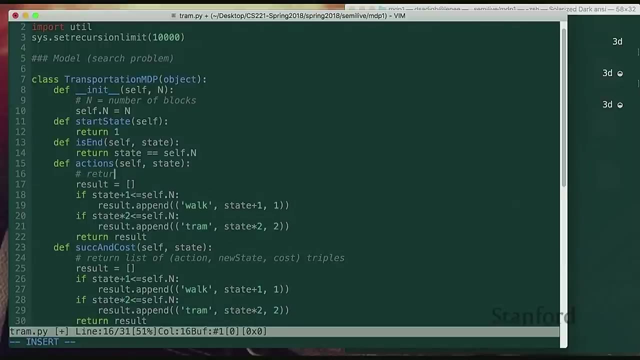 So the thing I'm gonna change is the first off, I need to add this: actions function okay, So what? what would actions do? it's going to return a list of actions that that are potential actions in a given state. So I just copy-pasted stuff from down there to just edit. 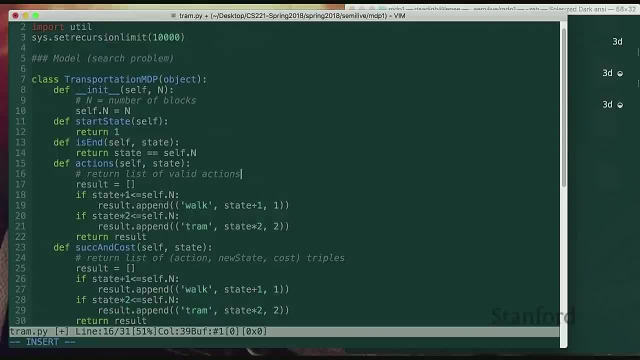 So it's gonna return a list of valid actions. okay, So what are the valid actions I can take? I can either walk or I can tram, So I'm gonna remove all these extra things that I had from before and just keep it to be. 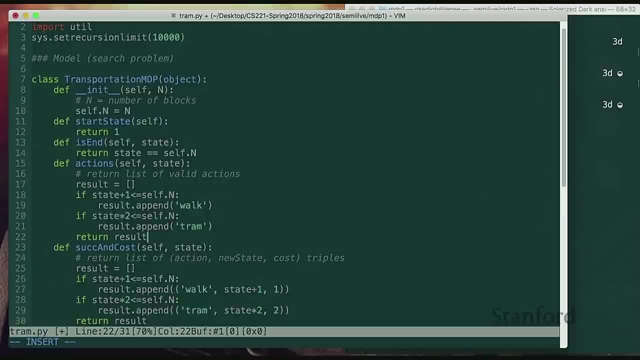 I'm either walking or I'm taking the tram. okay, As long as it's a valid state. So so that looks right for actions. The other thing we had was a successor and cost function, So so now we want to just change that and return these transition probabilities and and reward. 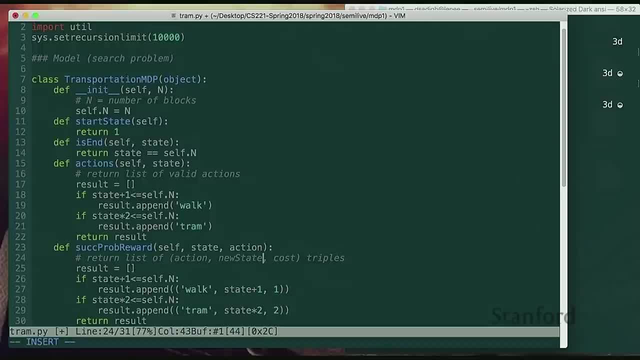 So so it's basically the successor, probabilities and reward, okay, So I'm putting those two together, similar to before we had successor and cost. Now I'm returning probabilities and reward, okay. So so what this function is going to return is it's going to return this new state. 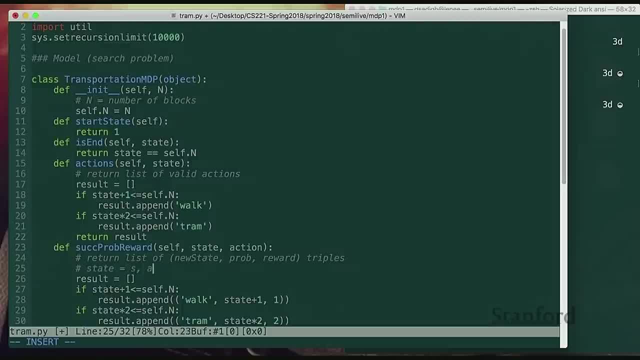 this S prime I'm going to end up at and the, the probability value for that and reward of that. okay, So so, given that I'm starting in state S and I'm taking action A, then what are the potential S primes that I can end up at? 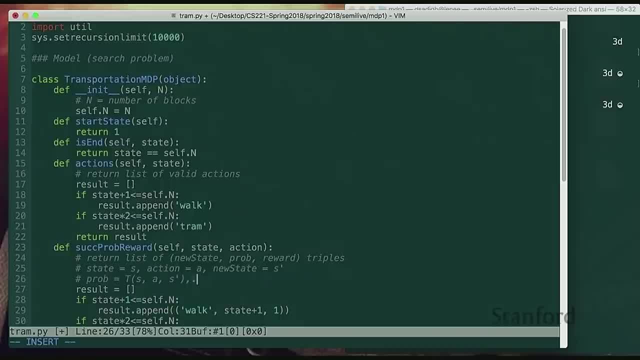 And what are the probabilities of that? Like, then, what? what is T of S A S prime And what is the reward of that? What is the reward of S A S prime? I? I wanna have a function that just returns these, so I can call it later, okay. 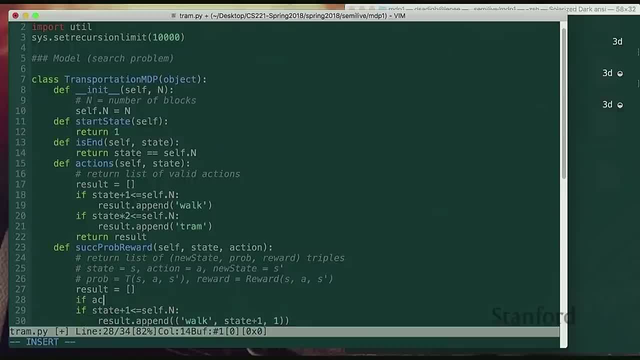 All right. So I need to basically check um like for for each one of these actions I can for. for action walk: What happens? for action walk, What's new state I'm gonna end up at? Well, I'm gonna end up at S plus 1.. 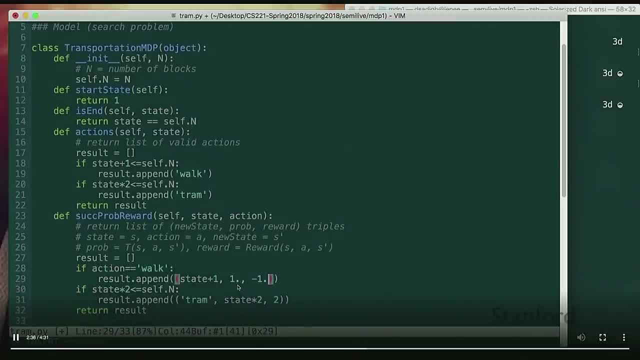 It's a deterministic action, so I'm gonna end up there with probability 1.. And what's the reward of that? Minus 1, because it's one minute cost, so it's minus 1. reward Then for action tram. 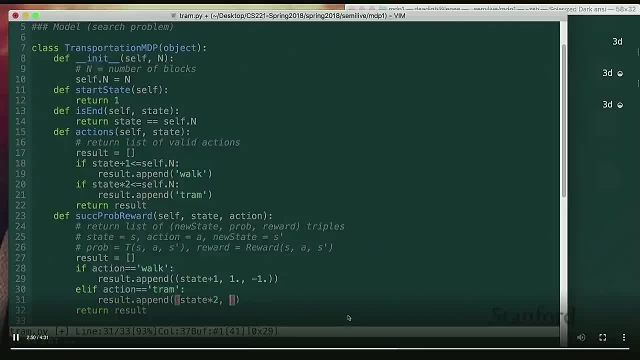 we kind of do the same thing but we have two options here. I can, I can end up in 2S. Tram doesn't fail. I end up in 2S with probability 0.5.. That cost, that reward of that is minus 2.. 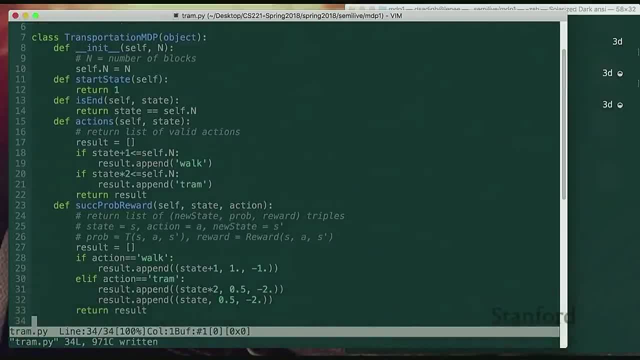 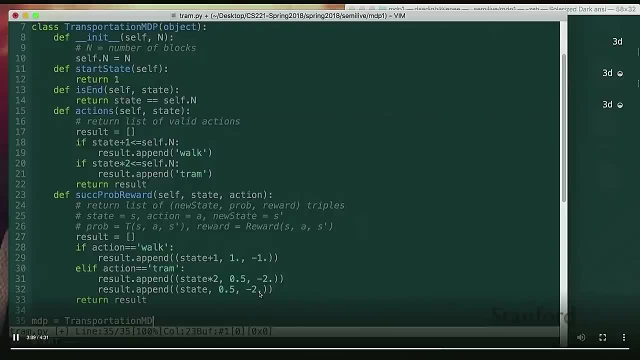 Or the other option is I'm going to end up in state S because I didn't go anywhere, because with probability 0.5, the tram did fail And that that the reward of that is minus 2. And that's pretty much it. 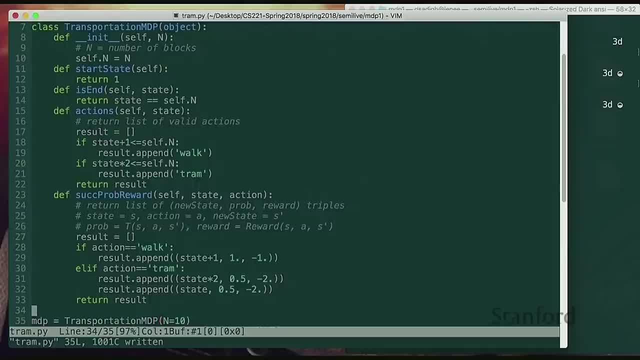 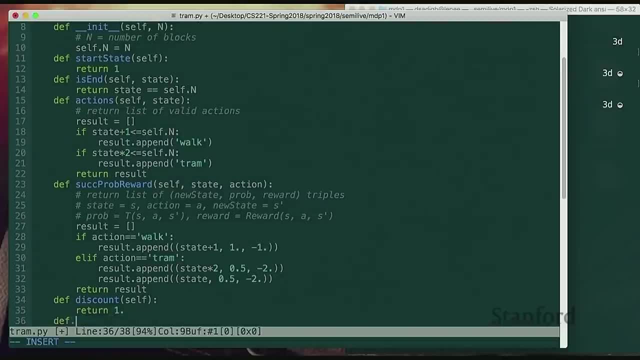 That. that is my, my MDP, So I can just define this for a city with, let's say, 10 blocks, Oh, and we need to have the discount factor, but we'll talk about that later. Let's say it's just 1 for now. 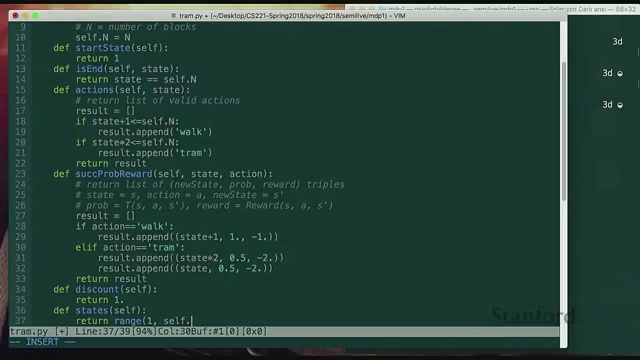 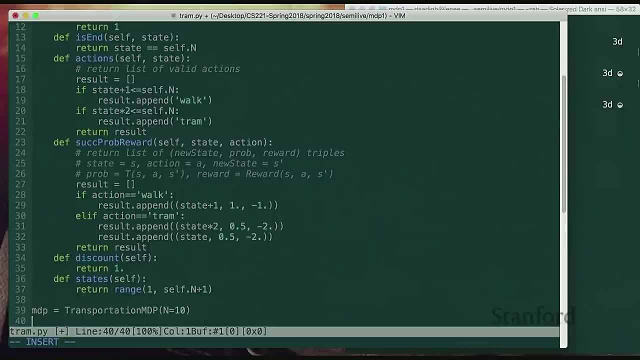 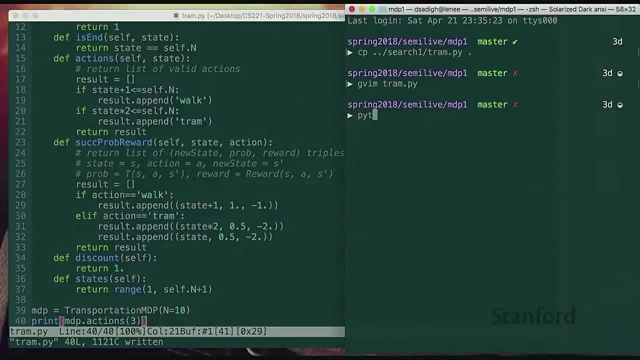 Okay, And I'll use write. I'm writing this. other states function for later. but Okay, Does that look right? We just formalized this MDP, So let's check if it does the right thing. So maybe we wanna know what are the actions from state 3?. 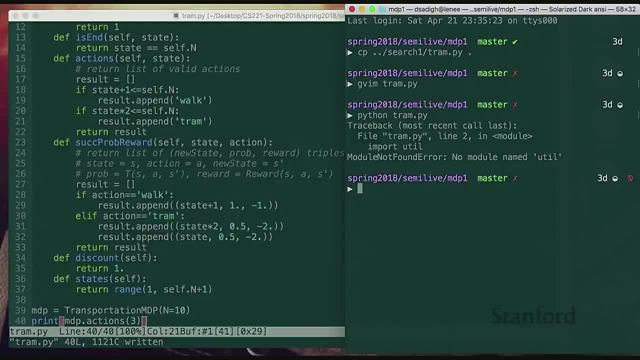 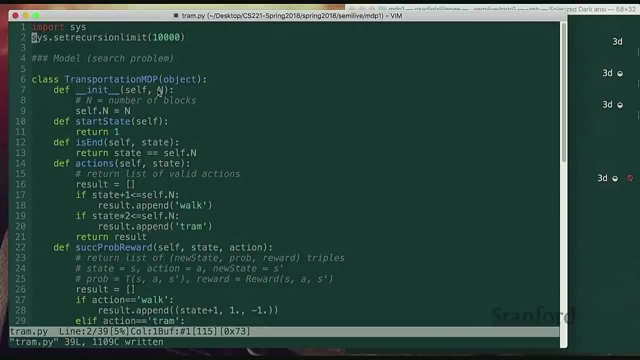 What are the actions from state 3?? Oh, we need to remove this util function from before because we don't have it in the folder. So remove that. What? what are the actions from state 3?? I have 10 blocks. 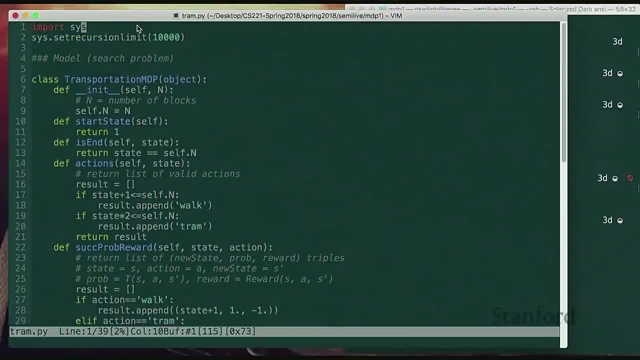 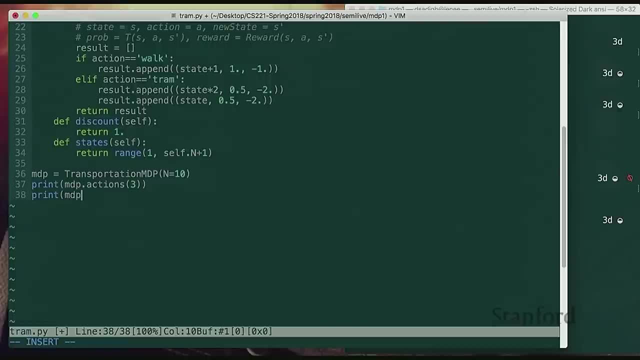 If I'm in state 3, I can either walk or tram. Either one of them is fine, right, So so that did the right thing. Maybe we wanna just check if this successor probability and reward function does the right thing. So maybe maybe we can try that out. 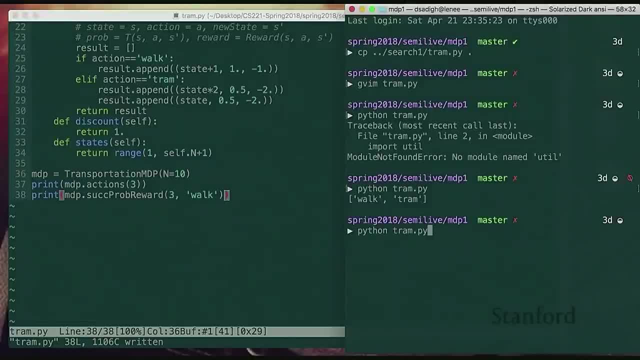 For state 3 and walk. So, so for state 3 and action walk. then what do we get? Well, we end up in 4, and, uh, that that is with probability 1, with the reward of minus 1.. 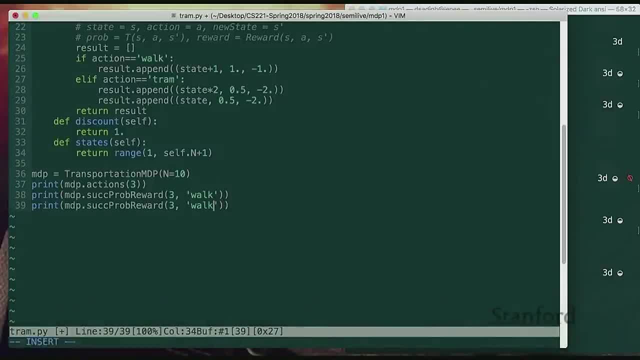 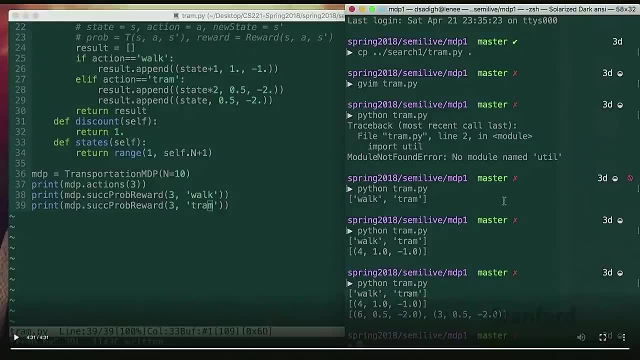 Okay, Let's try that for tram Again. remember, tram can fail, So I'm gonna get two things here. So these are the things I'm gonna get for tram. I'm going to either end up in 6 with probability 0.5,. 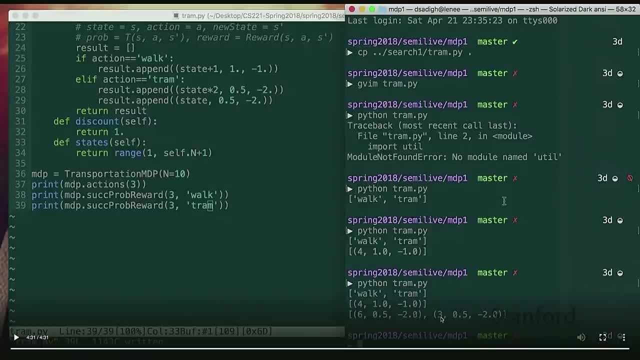 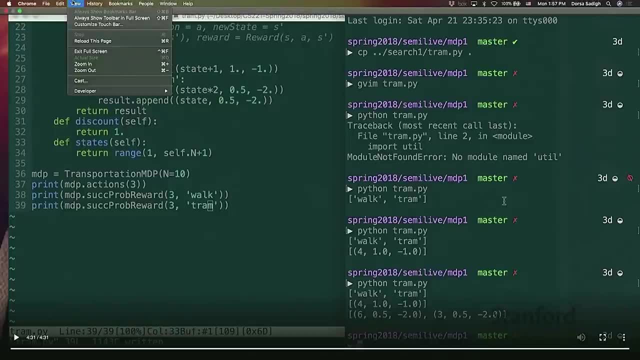 with the reward of minus 2, or I will not go anywhere. I'm still at 3 with probability 0.5,, and that is with the reward of minus 2.. Okay, All right, So that was just a tram problem. 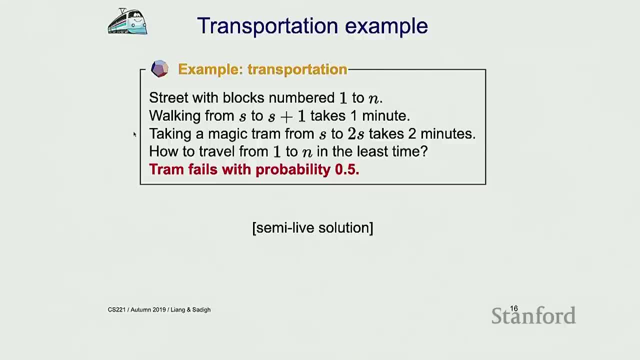 and we formalized it as an MDP. Again, the reason it's an MDP here is is that the tram can fail with probability 0.5. So we added that in when we defined our transition function and our prob- and our reward function. 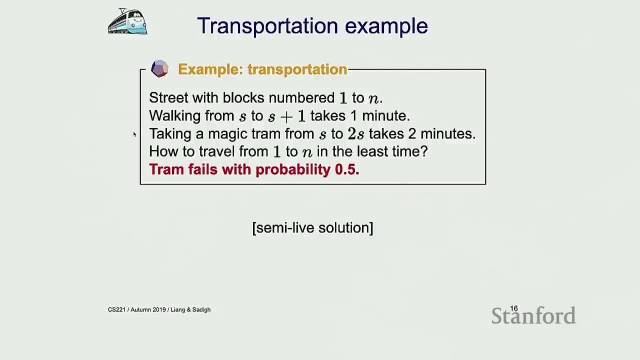 Okay, All right, Everyone happy with how we are defining MDPs? Yeah, Okay, Pretty similar to search problems, except for now we have these probabilities. Okay, All right. So so now I have defined an MDP. That's great. 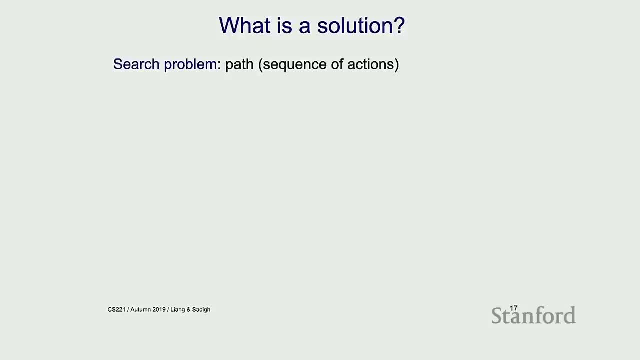 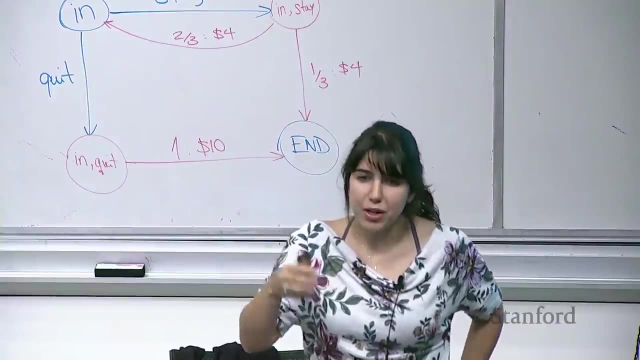 Uh, the next question that, in general, we would like to answer is to give a solution, right? So there's a question. So what does the Markov part of MDP mean? So the Markov part means that you just depend- so 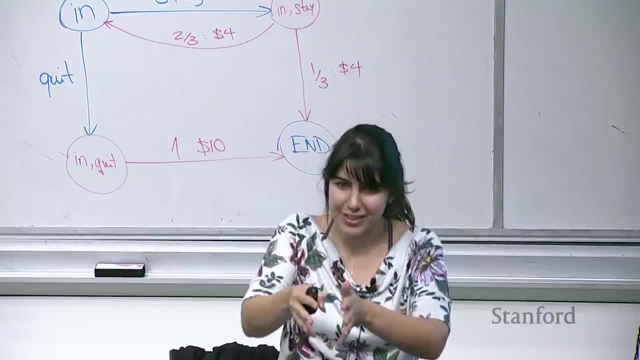 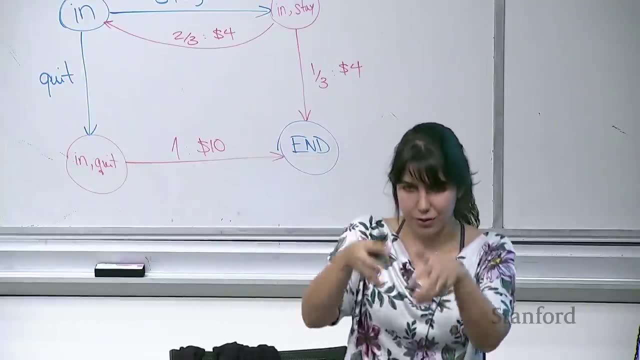 so when you, you just depend on the state, and and this current state, like the way we define our state, remember Our state is sufficient for us to make optimal decisions for the future. So the Markov part means that your Markovian only depends on. 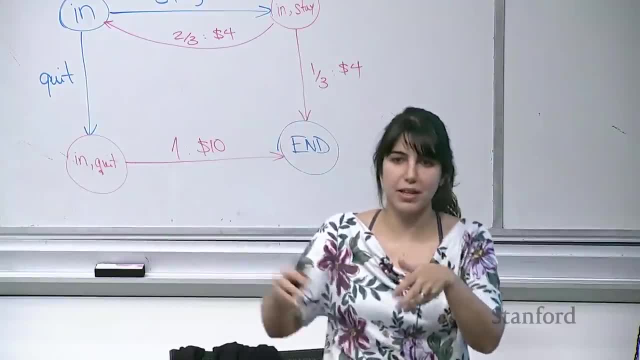 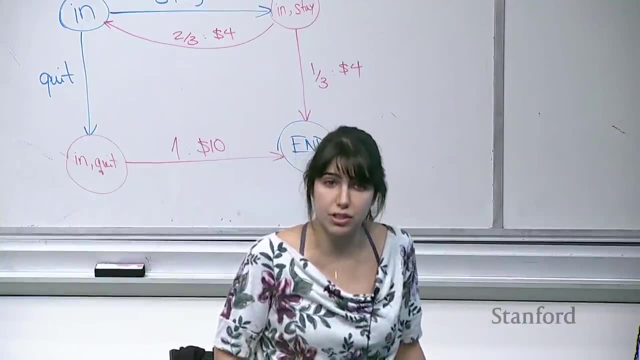 the current state and actions to end up in the probabilistically end up in the next next state. So, yeah, so the interesting question we would like to do is: well, we want to find a solution, right, I want to figure out what is the optimal path to. 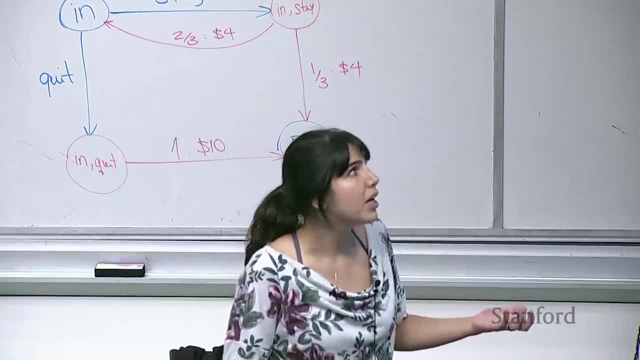 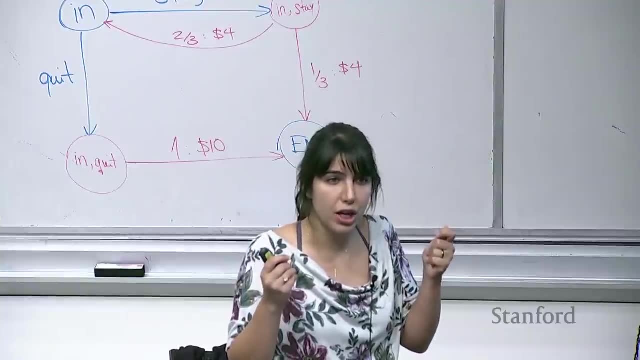 to actually solve this problem. And again, if you remember search problems, the solution to search problems was just a sequence of actions. That that's all I had Like a sequence of actions, a path that was a solution, And the reason that was a good solution was like everything was deterministic. 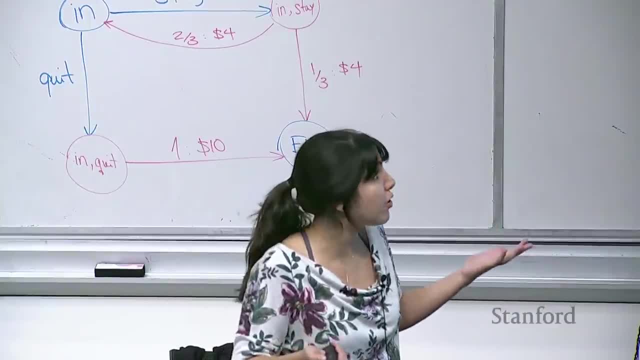 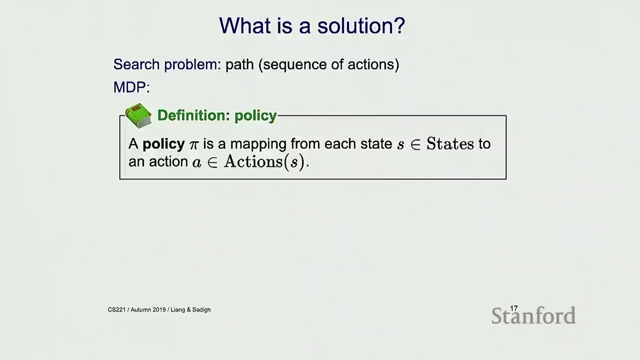 So I could just give you the path and then that that was what you would follow. But in the case of MDPs, the way we are defining a solution is by using this notion of a policy. So a policy. let me actually write that here. 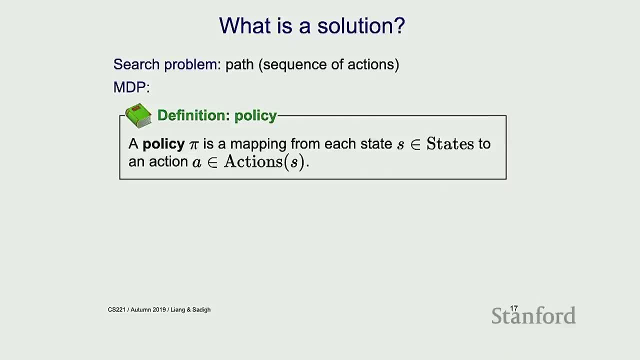 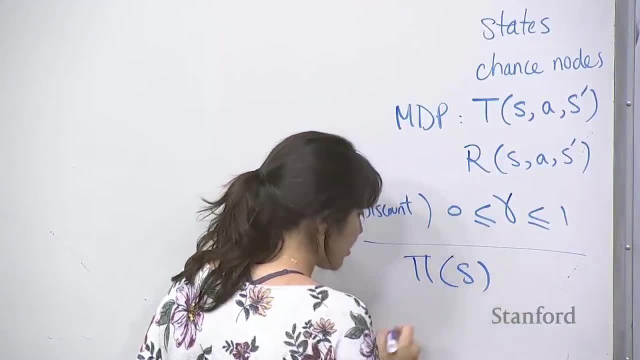 So so you've defined an MDP, But now I want to say: well, what is a solution of an MDP? A solution of an Markov decision process is a policy, Pi of S so, And this policy basically goes from states. 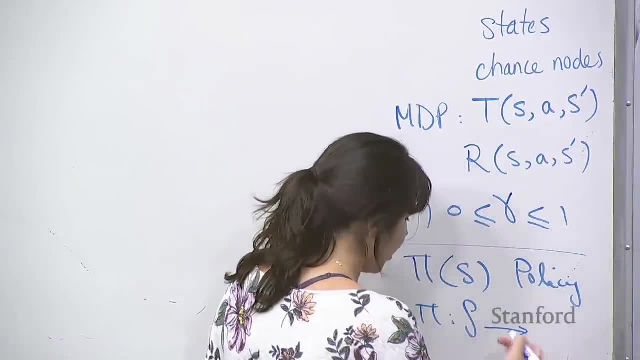 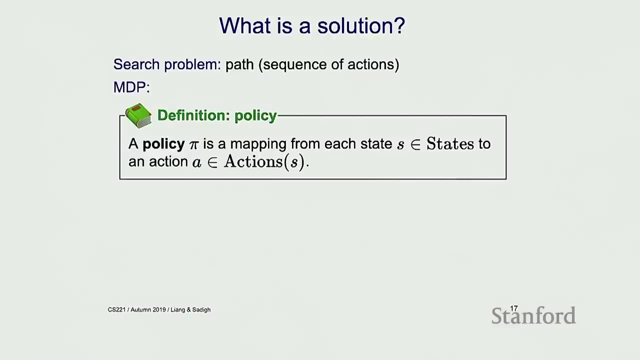 So it takes any state and it tells me: what is the po- what is the potential action that I would get? uh, for that state? Okay, So so a policy is a function. It's a mapping from each state S in the set of all possible states. 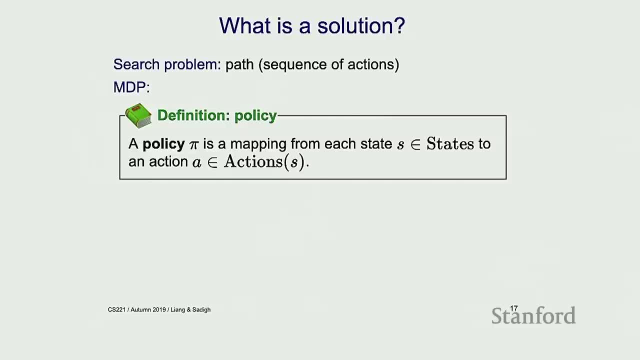 to to an action in the set of all possible actions. Okay, So in the case of a volcano crossing like I, can have something like this: I can be in state 1, 1 and then a policy of that state could be going south. 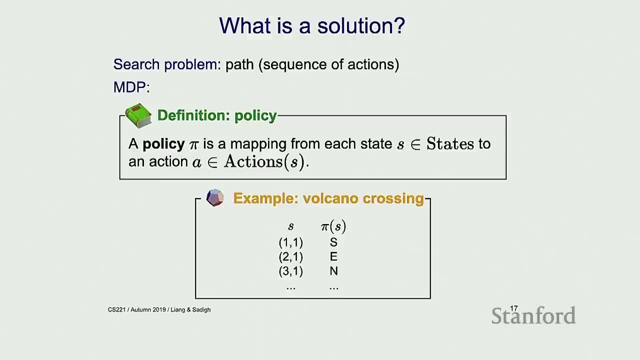 Okay, Or I can be in state 2, 1 and a policy for that state is east. If, if this was a search problem, I would just give a path. I would just say: go south, then, then go to go east and go north, right. 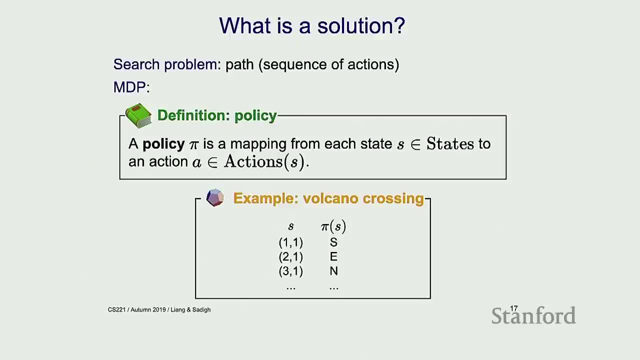 So, so that would be my solution, But, but again, like, if I decide that, well, the policy at 1, 1 is to go south, there is no reason for you to end up at south, right, Because this thing, this thing is probabilistic. 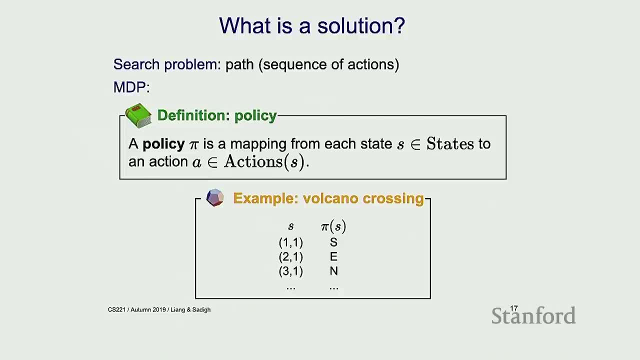 So so the best thing I can do is for every state, just tell you what is the best thing you can do for that particular state, And- and that's why we are defining a policy as opposed to get giving like a full path- Okay, 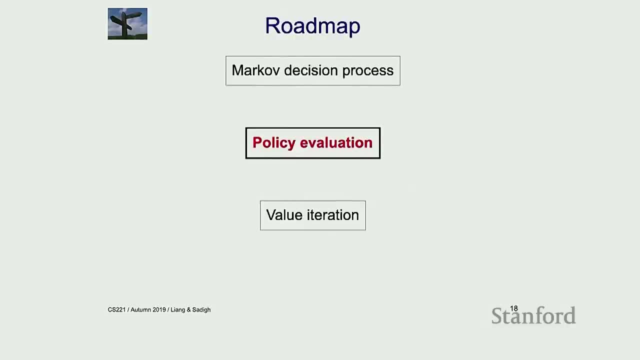 All right. So policy is the thing we are looking for, And- and ideally I would like to find this best policy. that would just give me the right solution. But in order to get there, I wanna spend a little bit of time talking about how good a policy would be. 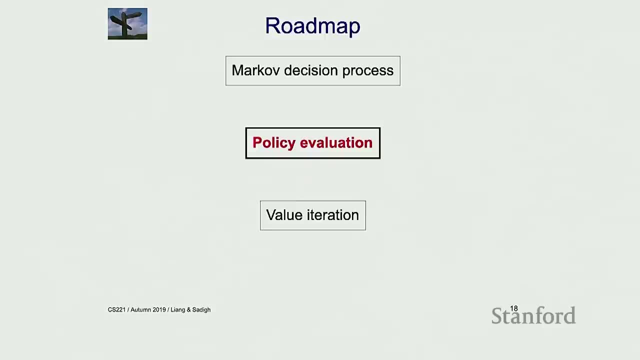 So and that's kind of this idea of evaluating a policy. So so in this middle section I don't wanna try to find a policy. I I just assume you give me a policy and I can evaluate it and tell you how good that is. 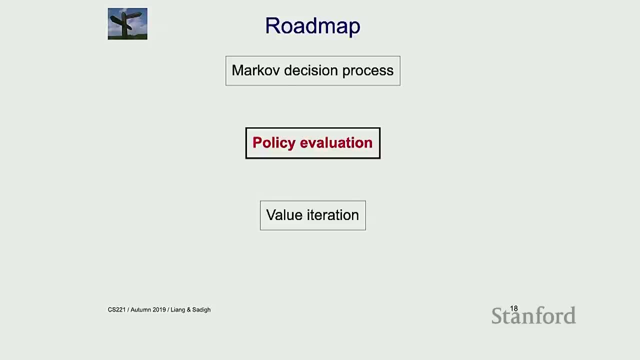 So so that's the plan for the middle section. Okay, All right, Everyone happy with it? So so, so far, all I've done is I've defined an MDP, which is very similar to a search problem. It's just probabilistic, Okay. 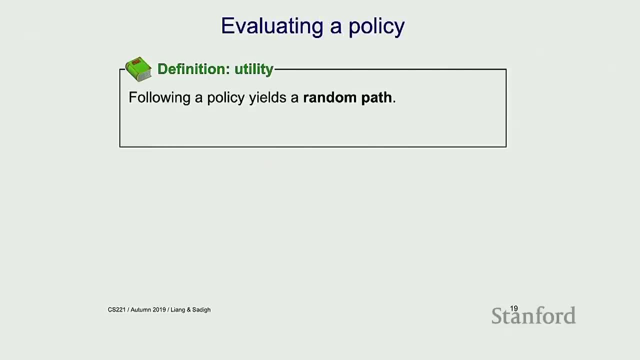 So so how would we evaluate a policy? Okay, So if you give me a policy which basically tells me I'd every state S takes some action, then that policy is going to generate a random path. right, I can get multiple random paths because nature behaves differently and the world is uncertain. 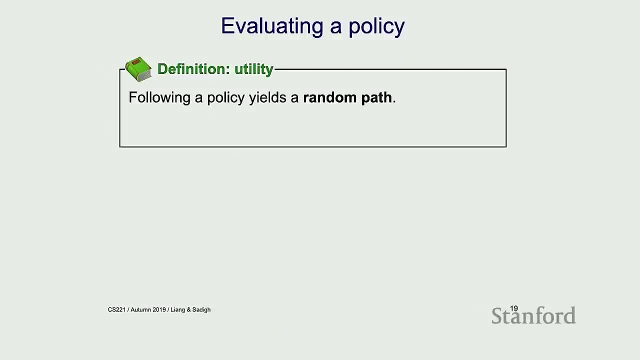 So I might get a bunch of random paths, and then those are all random variables. uh, random paths, sorry, And and then, and then, for each one of those random paths I can, I can define a utility. So so what is a utility? 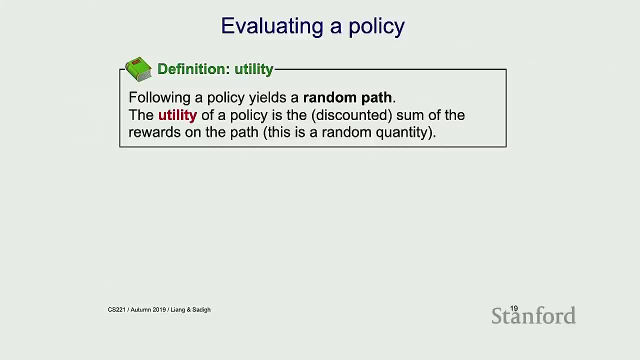 Utility is just going to be the sum of rewards, that I'm going to get over that path And I'm calling it as as the discounted sum of the rewards. Remember that discount, We'll talk about that, But but it can't. we can discount the future. 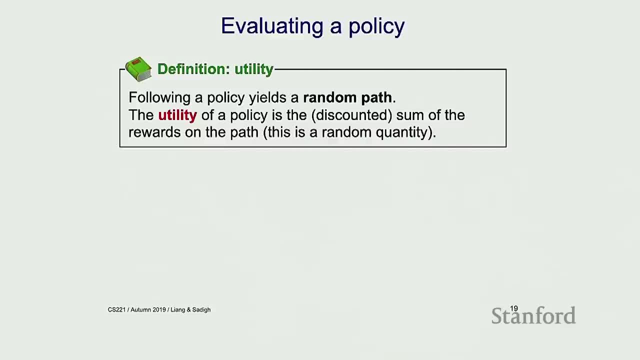 But, but for now, just assume it's just a sum of rewards on that path. Okay, So a uti- the utility that we are going to get is also going to be a random variable, right? Because if, if you think about a policy, 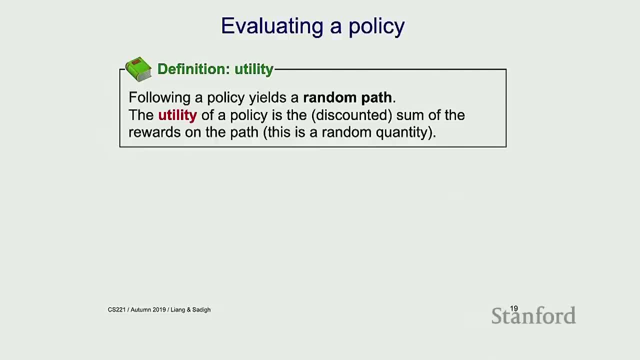 a policy is going to generate a bunch of random paths and and utility is just going to be the sum of rewards of each one of those. So it's a random variable. So so, if you remember this example right, So I can. 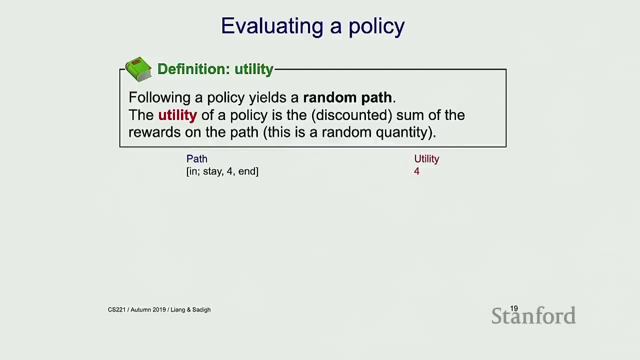 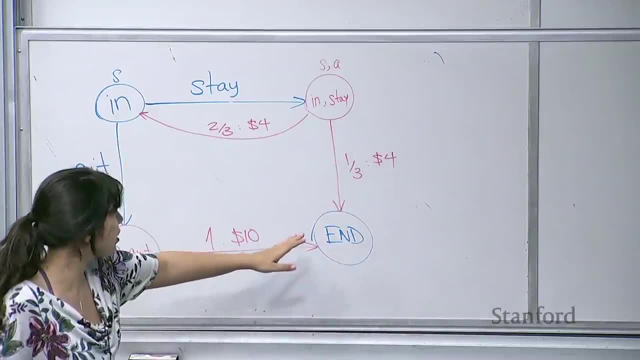 I can basically have a path that tells me start and end, and then stay, and then that ends right. So so this is one random path. And for this particular random path, well, what is the utility I'm gonna get? 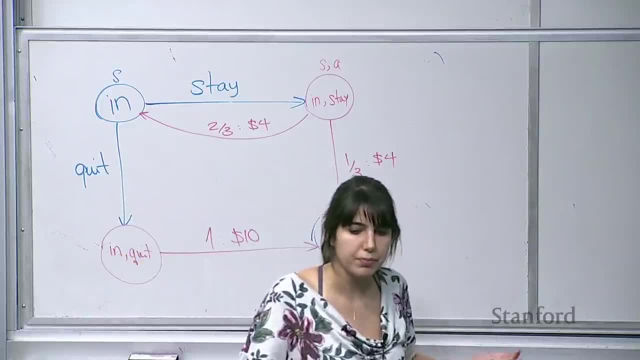 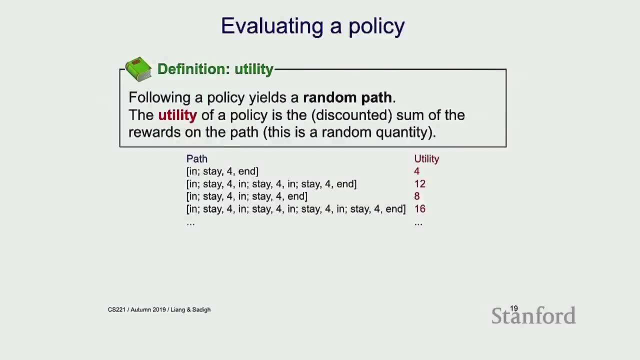 I'm just gonna get $4.. That's one possible thing that can happen If my, if my um policy is to, let's say, stay like there is no reason for for the game to end right here, right? 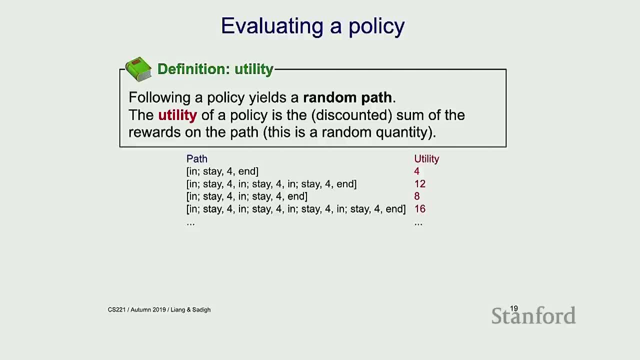 Like I can have a lot of different types of random paths. I can have a situation where I'm staying three times and then after that ending the game, and utility of that is 12.. We can have this situation where we have stay. 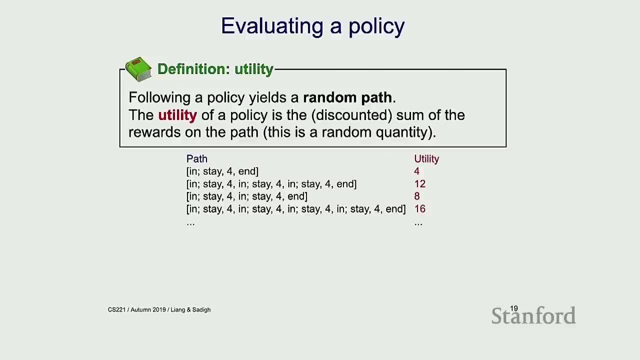 stay and end. that's the situation we saw. like you get a, you get a utility of eight, and so on. So so you're getting all these utilities for all these random paths. So so these utilities are also going to be just random variables, okay. 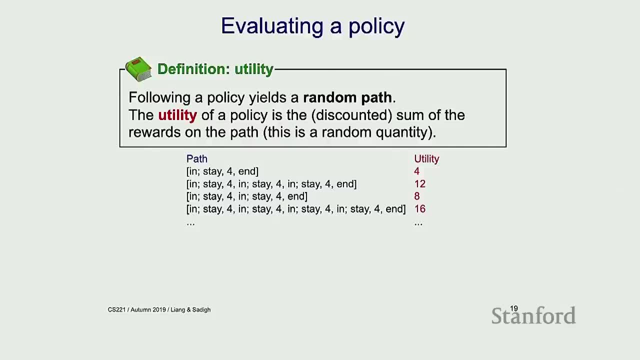 So I can't really play around with the utility. That's not telling me anything. Oh, it's telling me something, but it's a random variable. I can't optimize that. So instead we need to define something that we can actually play around with. 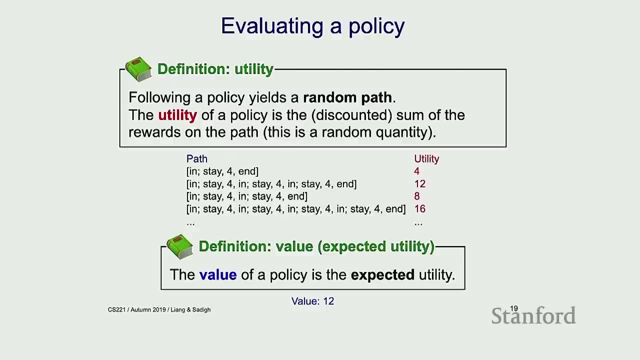 and then that is this idea of a value which is just an expected utility. So so the value of a policy is the expected utility of that policy, And then that's not a random variable anymore, that's actually like a number and I can- I can compute that number. 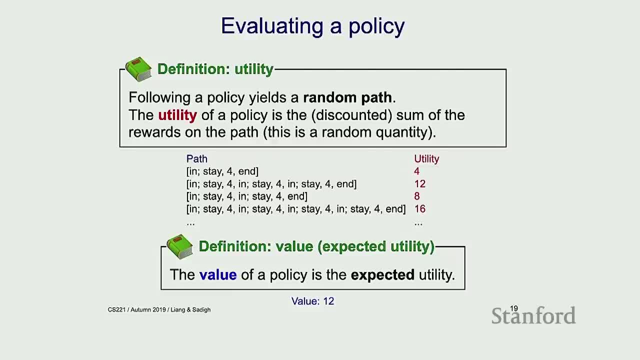 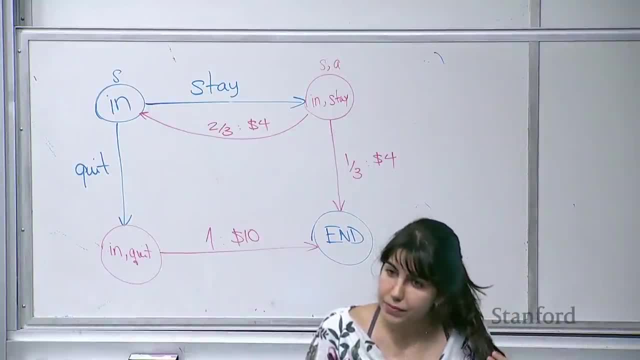 I can compute that number for every state and then just play around with value. okay, Is that policy mean defined for all possible states or a particular state For all possible? so? so the question is yes. so when you say a value of policy, 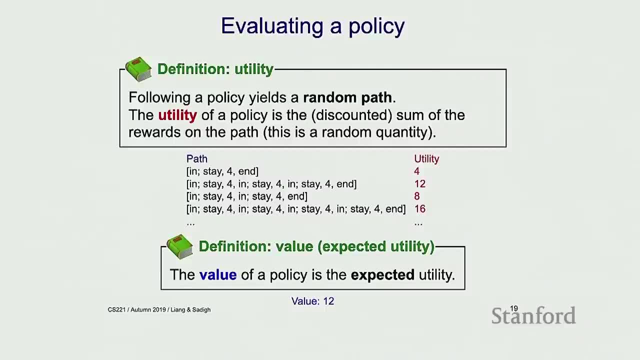 is the policy? basically telling me: um, is a policy basically telling me: uh, what is a strategy for all possible states? Well, um, you're defining policy as a function of state, right, So and value the same thing is a function of state. 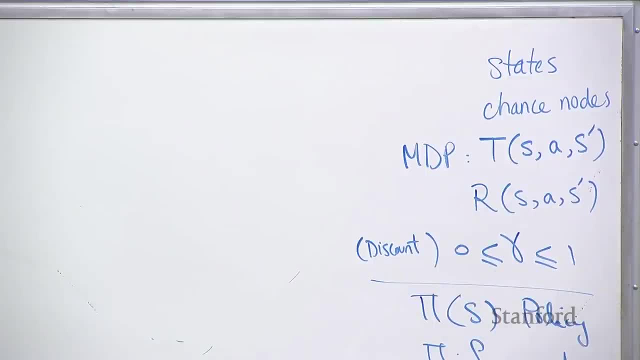 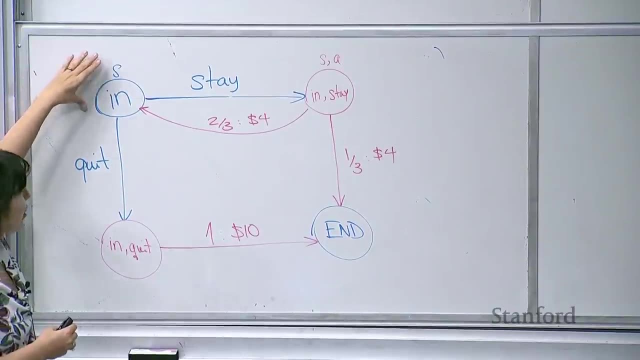 I might ask: what is the value of being an in? So the value of being an in is is, uh, an following and following policy state. is is going to be the the value of fo- following policy state. um, and following policy state. 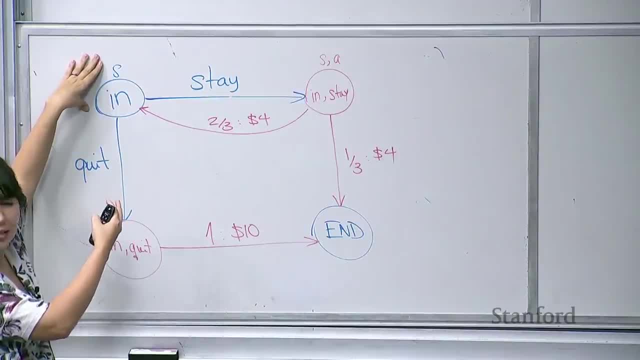 stay from this particular state, which is the expected utility of that, which is, which is basically that 12 value there. I could ask it about any other state too, So I can be in any other state and then say, well, what's the value of that? 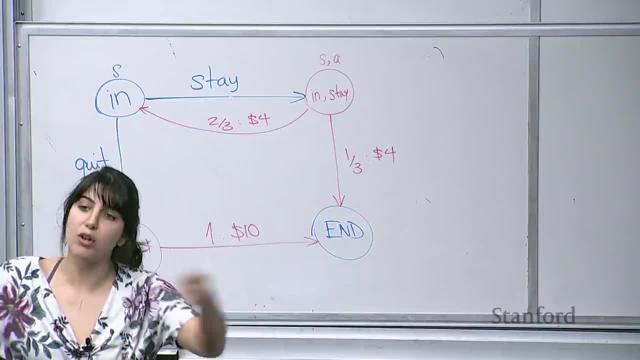 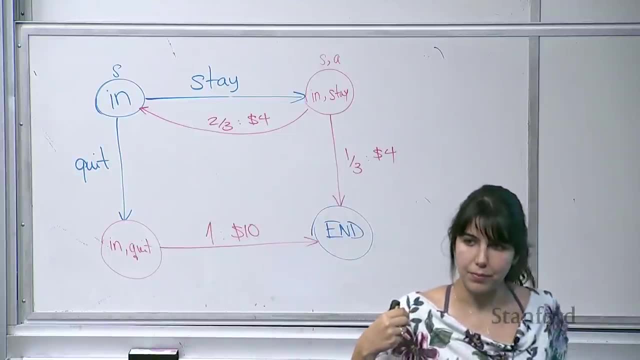 And and when we do value iteration and we actually need to compute this value for all states to kind of have an idea of how to get from one state to another state. But What is this with respect specifically to being in state in? Yeah, 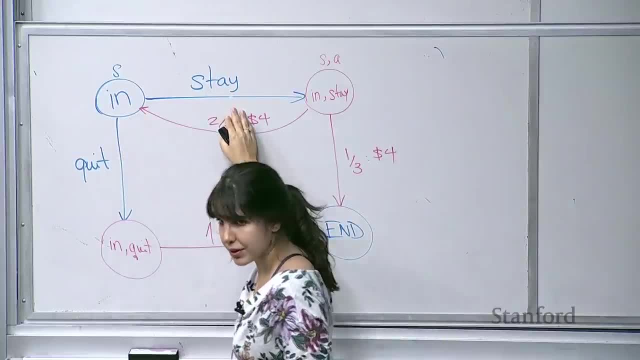 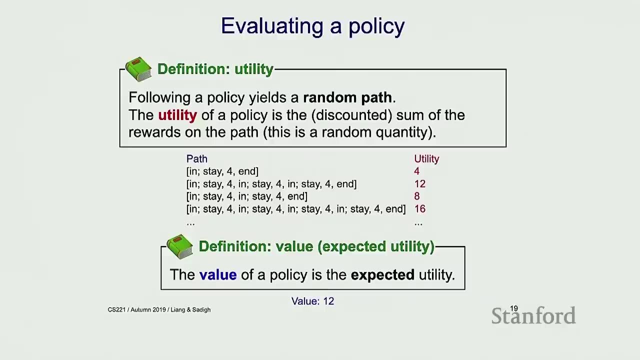 And the policy given your state in taking the action. state Yes, Okay, Yeah, And that is that is what. 12 is Okay And and 12, like we kind of empirically have seen it's 12, but we haven't like shown how to get 12 yet. 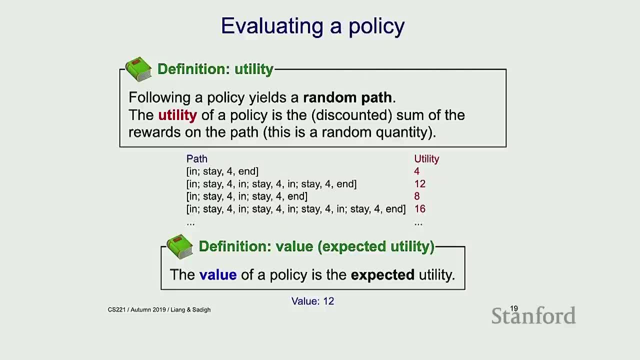 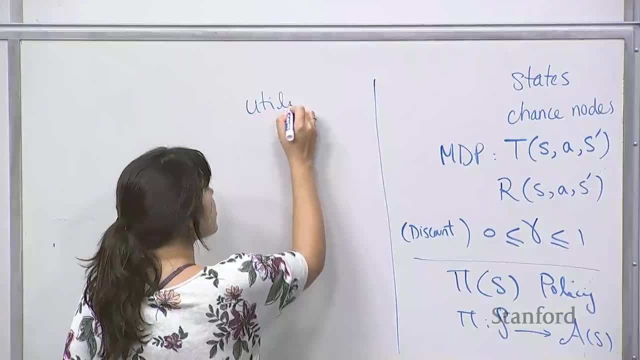 Okay, All right. So, um, actually, let me write these in my list of things. So we talked about the policy. What else did we talk about? We talked about utility. So what is utility? Utility, we said it's sum of rewards. 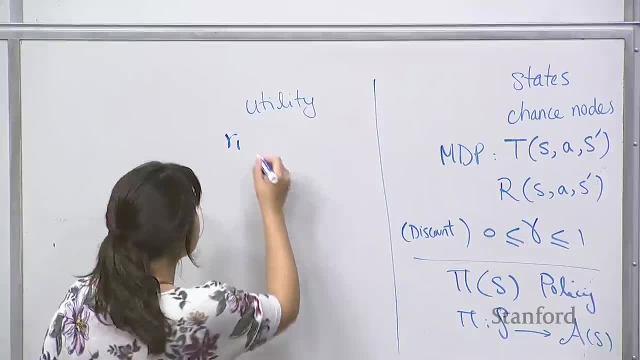 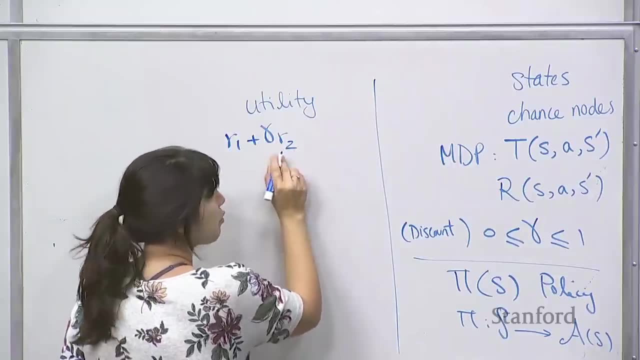 So if I get like reward one, then I get reward two. It's a discounted sum of rewards, So I'm gonna use this gamma, which is that discount that I'll talk about in a little bit- times reward two plus gamma, squared times reward three, and so on. 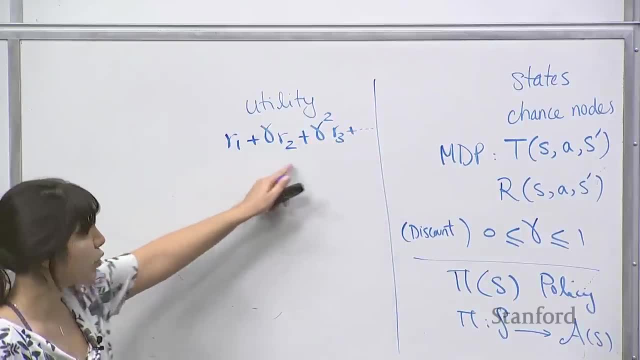 So utility is you give me a random path and I just sum up the rewards of that. Imagine, if gamma is one, I'm just summing up the rewards. If gamma is not one, I'm summing. I'm looking at this discounted sum. 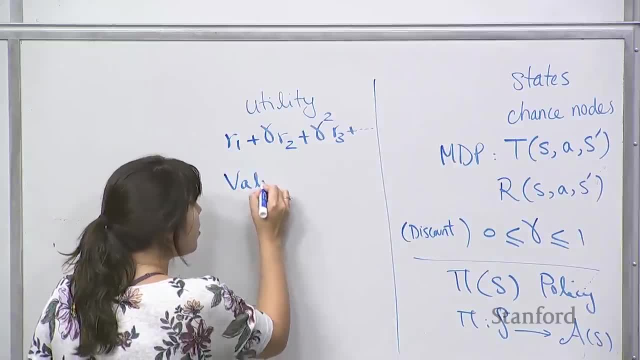 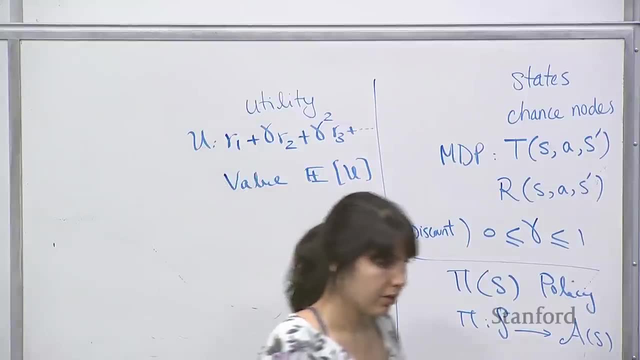 Okay So. so that is utility, But value. so this is utility, Value is just the expected utility. Okay, So you give me a bunch of a random path. I can compute their utilities. I can just sum them up and average them. 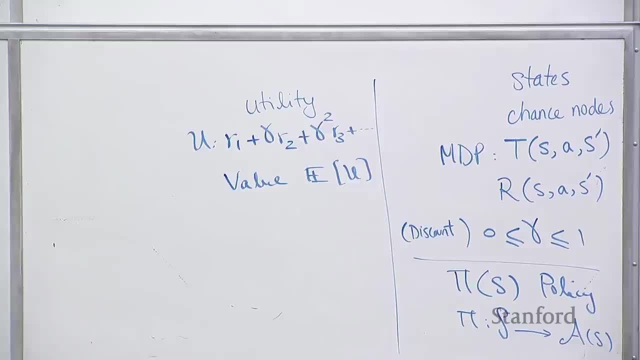 and that gives me value. That's a very good question. We'll get back to that, So so. so, in general, in in, in. okay if. if it is acyclic, it is fine, But if you have a cyclic graph, 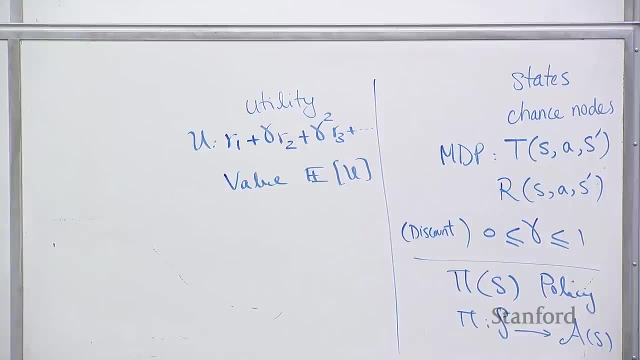 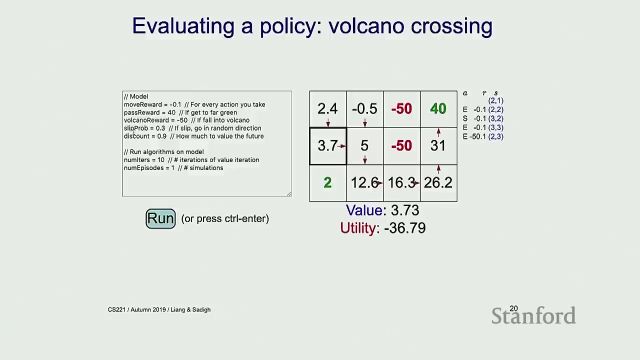 you want your gamma to be less than one, And we'll talk about that when we get to the convergence of of these algorithms. All right, Okay, All right, So. so let's go to the this particular volcano crossing example. 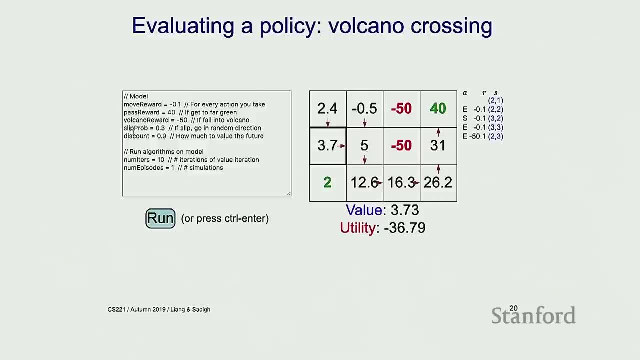 So in this case, like I can run this game and every time I run it I'm gonna get a different utility because, like I'm gonna end up in some random path, some of them end up in the volcano. that's pretty bad right. 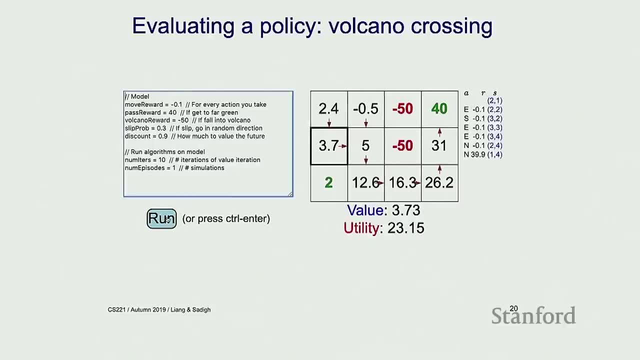 So I get different utility values, utilities, But the value which is the expected utility, is not changing really, it's just around 3.7, which is just the average of these utilities. So I can keep running this, getting these different utilities, but 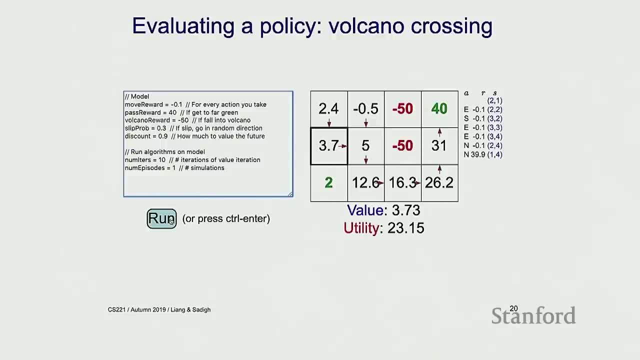 but value? is this one number, that that I can, I can talk about And and that's the value of this particular state, And that tells me, like what would be the best policy that I can take and what's the best amount of utility that I can. 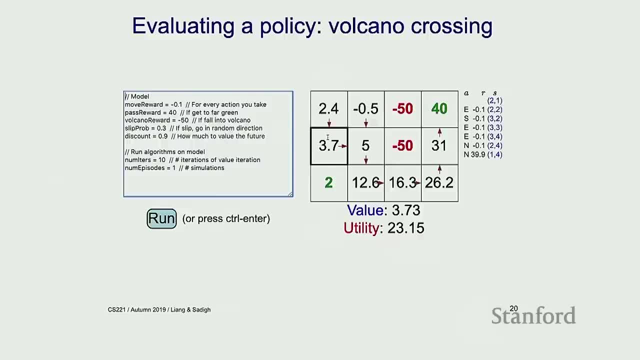 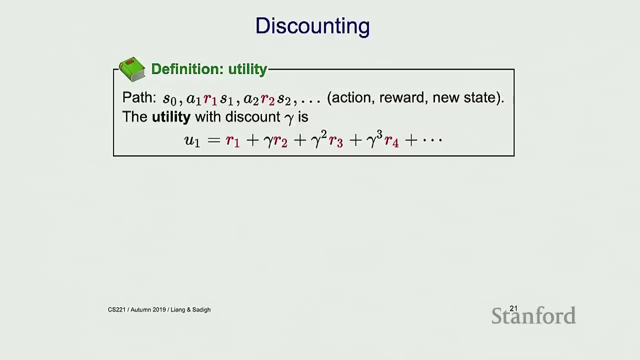 get from an expectation from that state. Okay, All right. So we've been talking about this utility. I've actually written that already on the board. So utility is going to be a discounted sum of rewards. And then we have been talking about this discount factor. 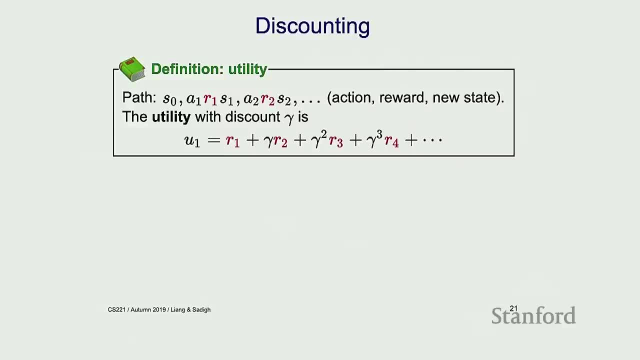 And the idea of the discount factor is: I might like care about the future differently from how much I care about now. So so, for example, if if you give me $4 today and you give me $4 tomorrow, like if that $4 tomorrow is the same kind of amount and has the same value to me as 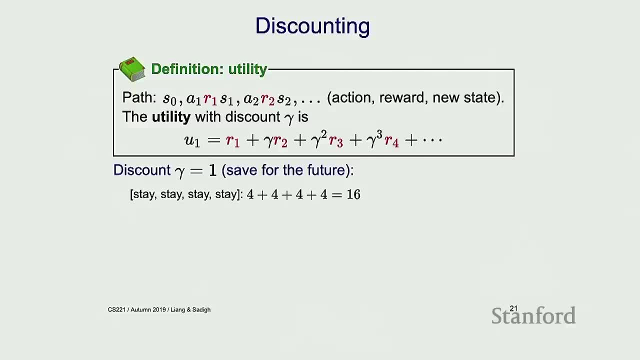 as today then then I might. it's kind of the same idea of having a discount counter of one, count discount of of one, So you're saving for the future. The values of things in the future is the same amount. 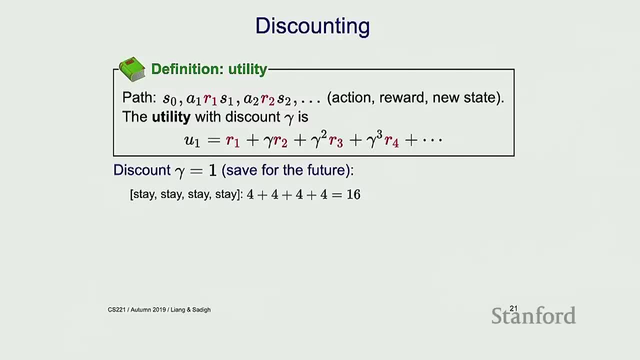 If you give me $4 now, if you give me $4 10 years from now, it's going to be $4.. I care about it like the $4 amount and I can just add things up, But it could also be the case. 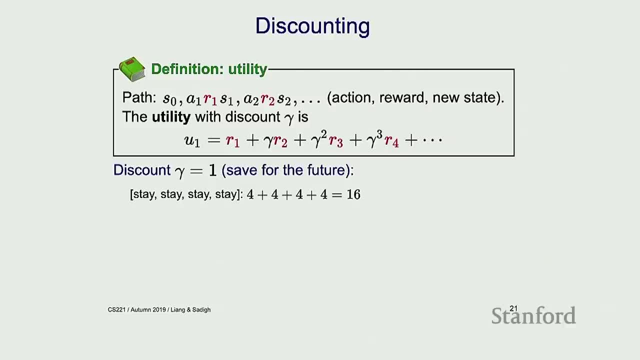 like you might be in a situation in a particular MDP where you don't care about the future as much. Maybe you give me $4 10 years from now and that's that doesn't like I don't have any value for that. 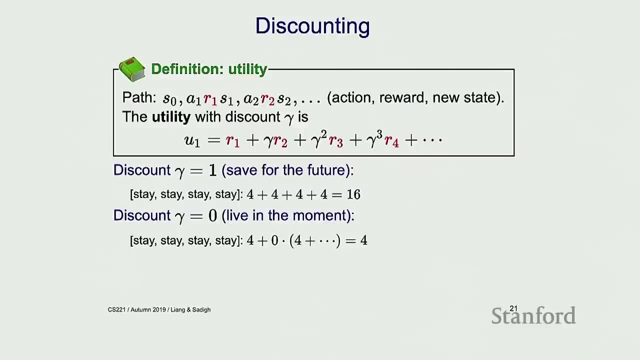 So, uh. so then, if that is the case and you just want to live in the moment and you don't care about the values you're going to get in the future, then that's kind of the other extreme, when, when this, this gamma. 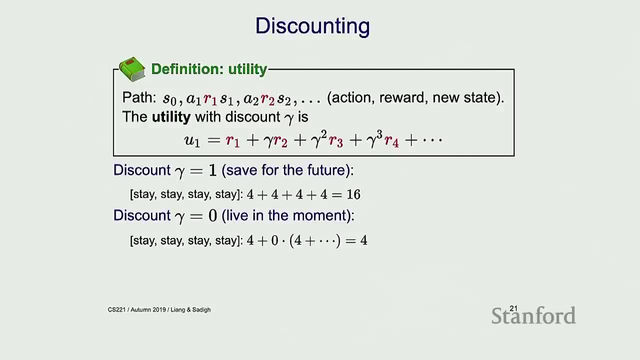 this discount is equal to zero. So so that is a situation that if I get $4 in the future that they don't like value, like they don't have any value to me, they're just like are zero to me. So so I only care about right now living in the moment. 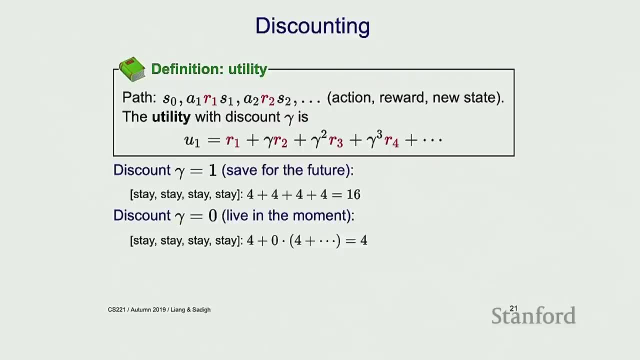 what is the amount I'm going to get? And and in reality, you're like somewhere in between, right, Like we are not just this case where we are living in a moment. we're also not this case that that everything is just the same amounts like right now or in the future. 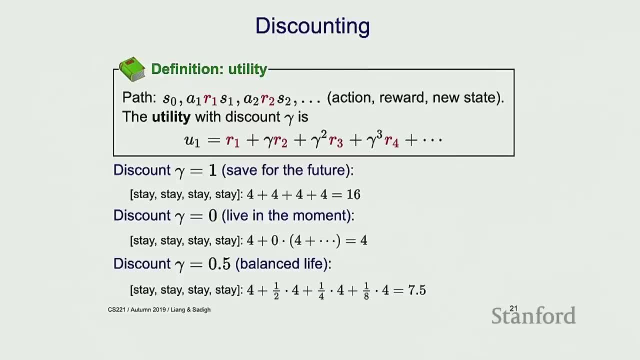 And and like in balanced life is a setting where we have some discount factor. It's it's not zero, it's not one. It actually discounts values in the future, because future maybe doesn't have the same value as now, But, um, but we still value things in the future. 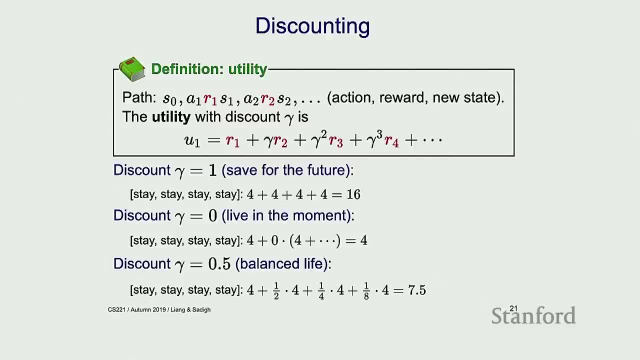 like $4, is still something in the future And- and that's where we pick, like a gamma that's between zero and one. So so that is kind of a design choice: like, depending on what problem you're in, you might want to choose a different gamma Question. 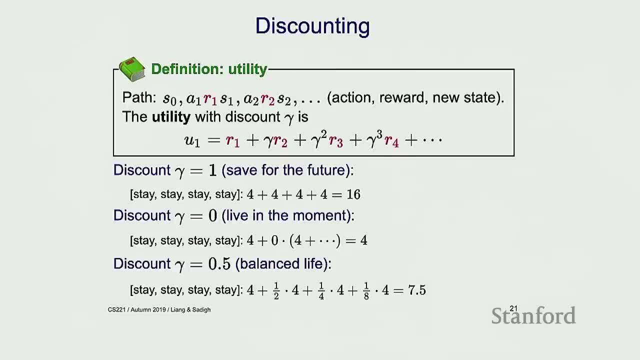 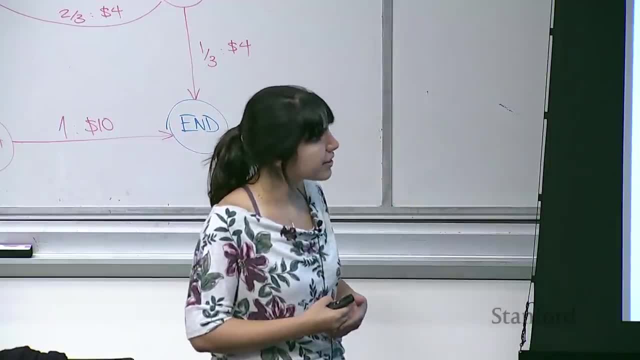 So is discounting usually like that? Is it a assessment of risk, or is there like a different way where you can assess how much risk you want to take? Um, you could, you could think of it as an ass- it's not really an assessment of risk in that way. 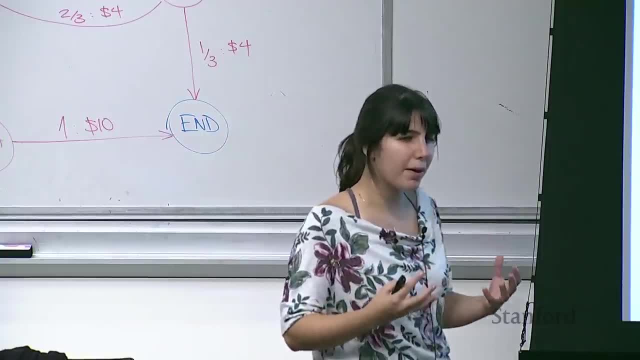 It depends on the problem, right, It depends on, like, in a particular problem, I do want to get values in the future. I have like some sort of long-term like goal that I want to get to and I care about the future. 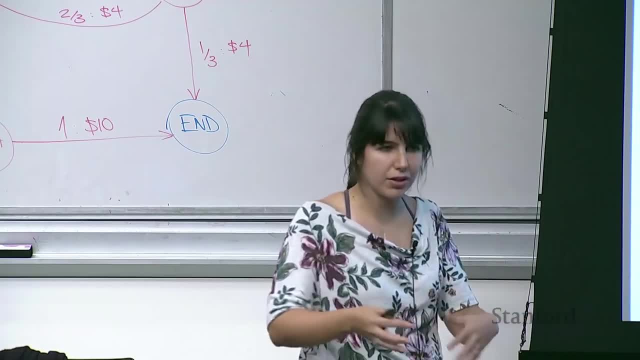 Like it, it depends, like if you're solving a game versus you're solving, like I don't know what, what a mobi-, like a robot, manipulation problem, Like it might just be very different, like discount factors that you would use. 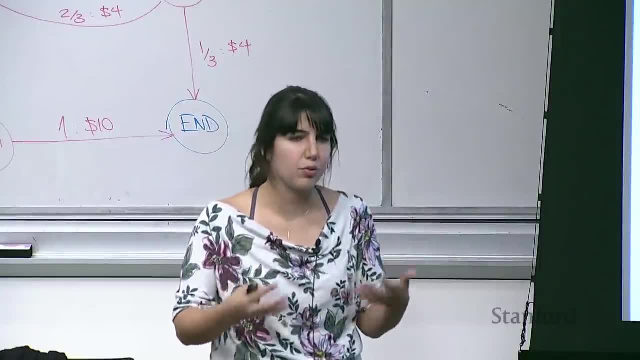 For a lot of examples we would use in this class, we would just choose a gamma that's close to one Like, like usually. like for for a lot of problems that we end up dealing with, gamma is like 0.9,. 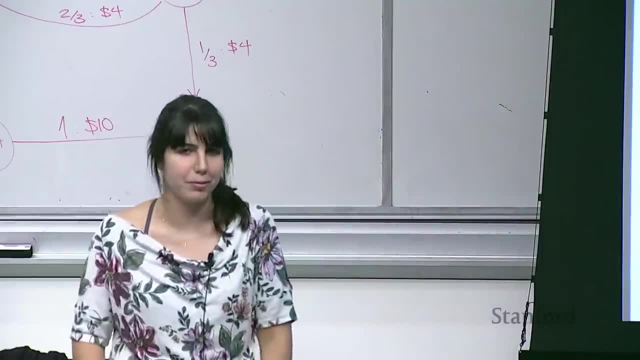 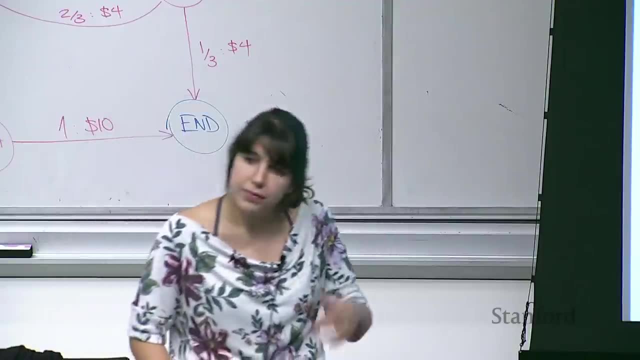 that's like the usual. okay, Like for usual problems. like you might have a very different problem where we don't care about the future, So so then we just drop it. yes, A quick question: Is gamma a hyperparameter that needs to be tuned? 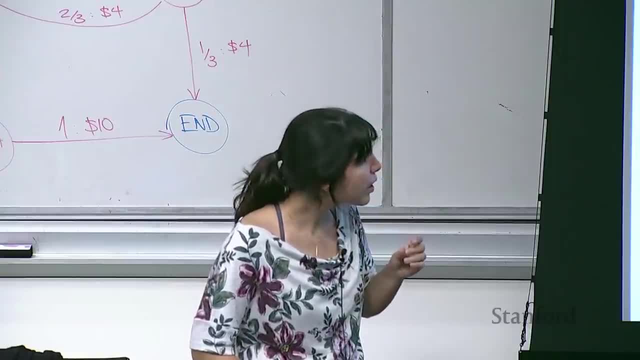 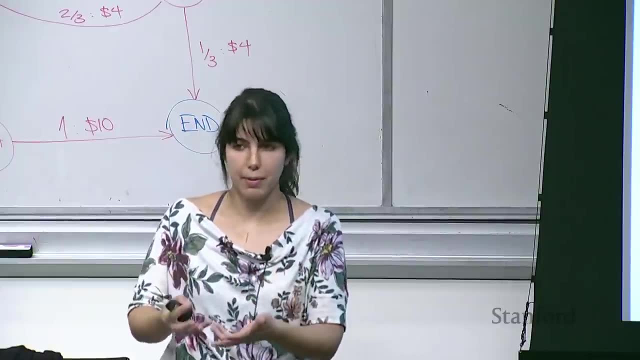 And is a gamma of zero the same as a greedy algorithm Gamma? okay, so so that's a good question. So is gamma a hyperparameter that you need to tune? I would say gamma is a design choice. It's not a hyperparameter necessarily in that sense that. 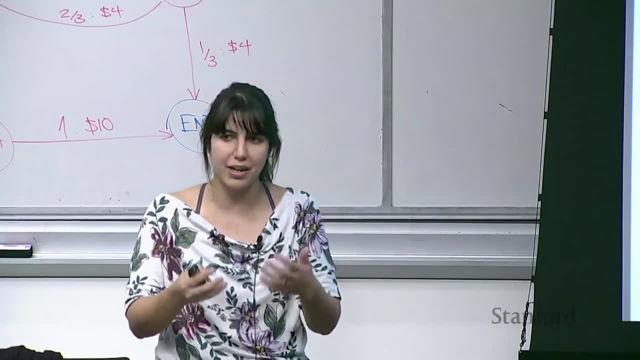 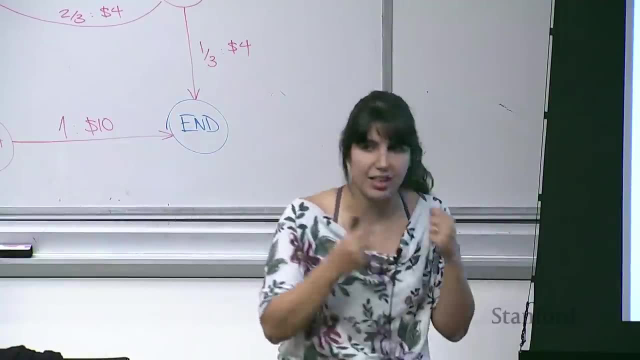 oh, I'll pick the right gamma that will do the right thing. You would want to pick a gamma that kind of works well with your problem statement And and gamma of zero is kind of yeah, greedy, Like you're picking, like what is the best thing right now. 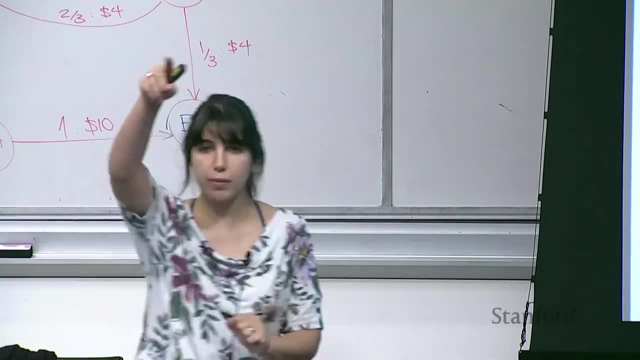 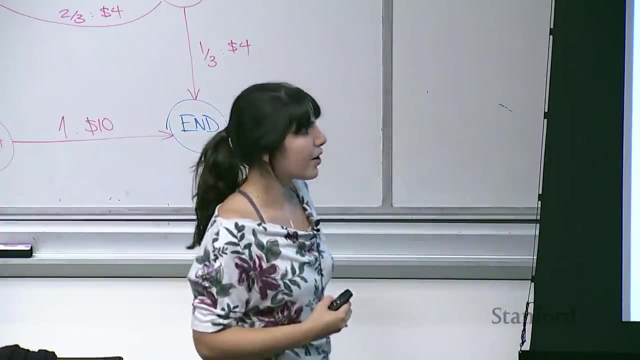 and I just don't care about the future. ever Question back here: Does the gamma violate the Markov property? because, like this kind of memory of like what your state is, It doesn't violate the Markov property. It's just a discount of like. it's about the reward. 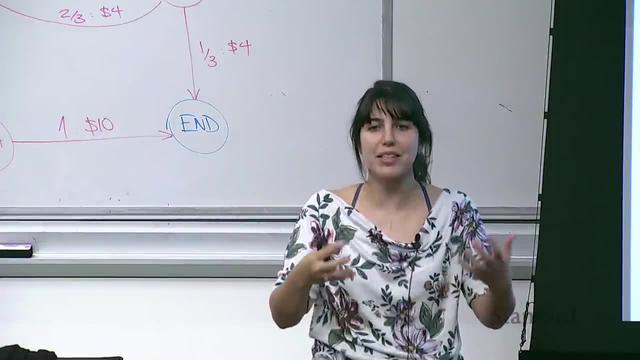 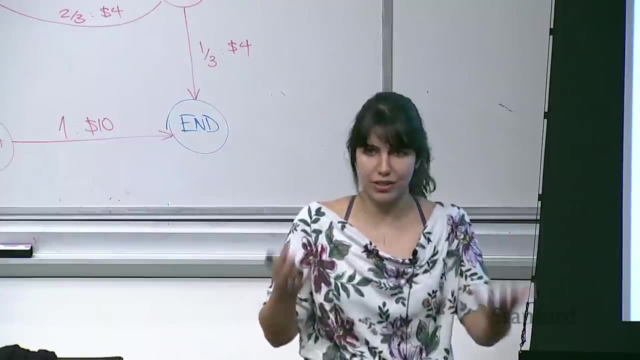 It's not about how this state affects the next state. It it's basically affects how much reward you're gonna get, or how much do you value reward in the future. It doesn't. it doesn't actually like. it's still a Markov decision process. 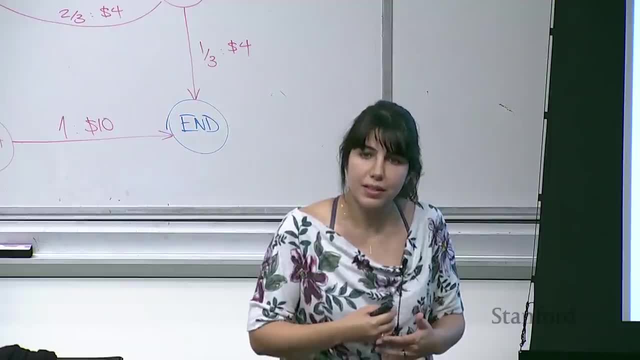 Markov is like the states and like your possible actions are memoryless, but the rewards can have some- What you're getting, what the re- it's affecting the reward? yeah, But it's Markov, because, yeah, if I'm in state S and I take action, A. 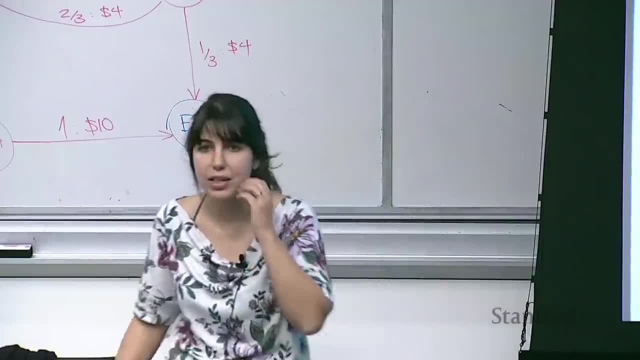 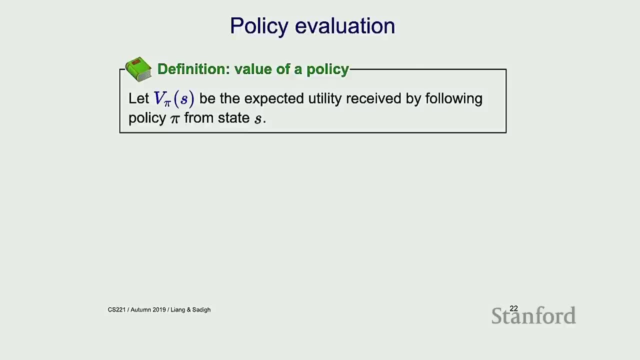 I'm gonna end up in S prime and that doesn't depend on like gamma, All right, So okay. So so in this section we've been talking about this idea of someone comes in and gives me the policy. So the policy is pi. 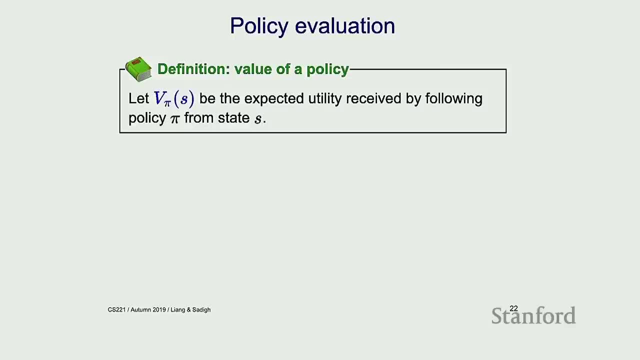 And what I wanna do is I wanna figure out what's the value of that policy. And again, value is just expected utility, okay, So v pi of S is just expected utility received by following this policy. pi from state S okay So, so I'm not doing anything fancy. 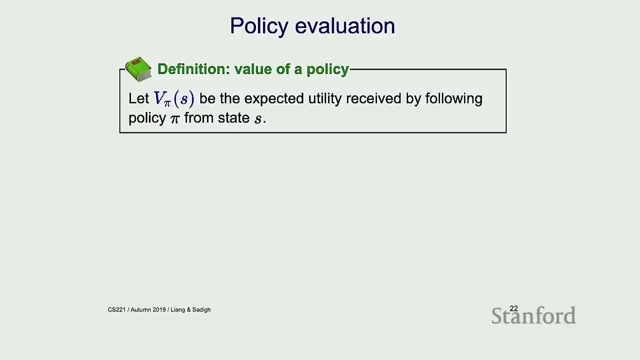 I'm not even trying to figure out what pi is. All I wanna do is I wanna just evaluate. If you tell me this is pi, how good is that? what's the value of that? okay, So, so that's what a value function is. 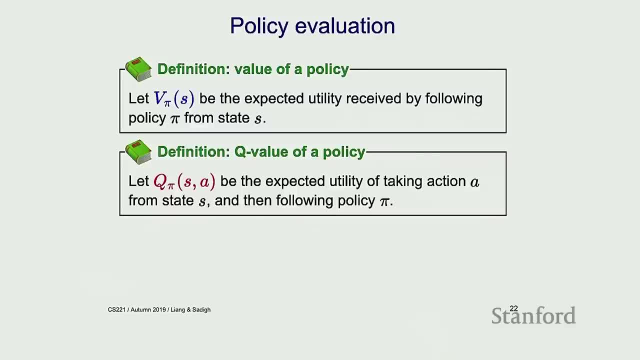 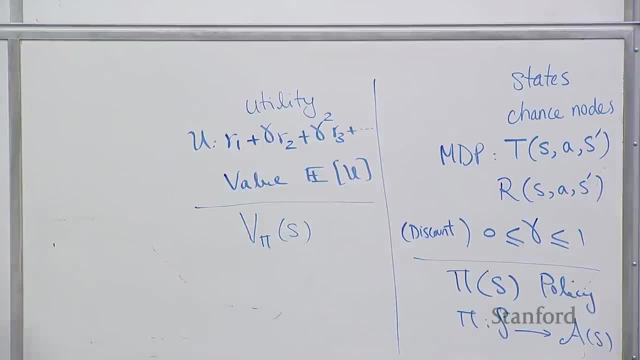 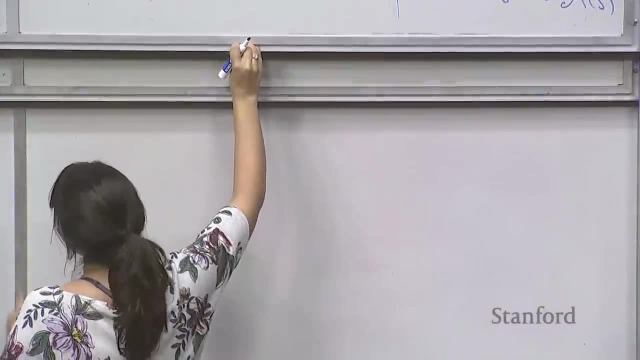 So value of a policy is: is v pi of S? okay, That's expected utility of starting in some state. Um, let me put this here and then I'm gonna move these up. Um, yeah, oops, Yeah, So v pi is. 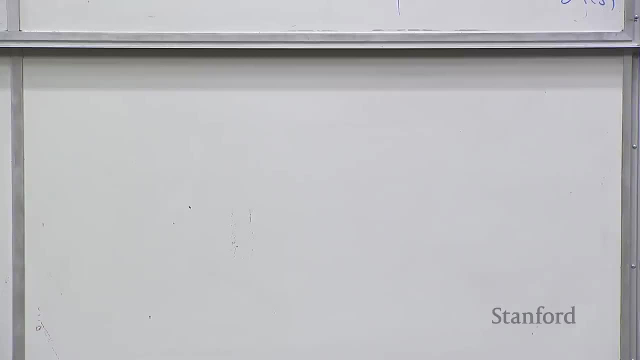 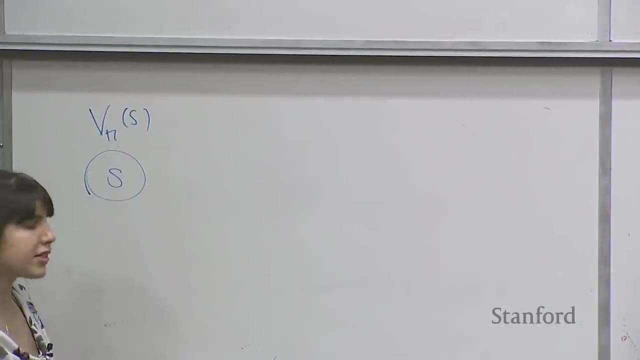 is the value of the expected utility of me starting in some state S. okay, And state S has value of pi of S. And if someone tells me that well, you're following policy pi, then I already know from state S the action I'm gonna take is pi of S. 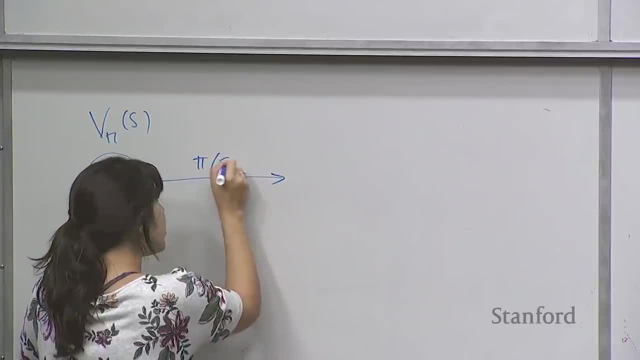 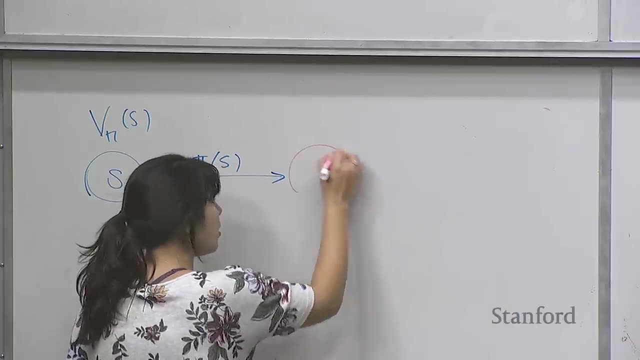 So that's very clear. So I'll take pi of S. And if I take pi of S, well I'm gonna end up in some chance note. okay, And that chance note is is a state action note, It's going to be S And the action. 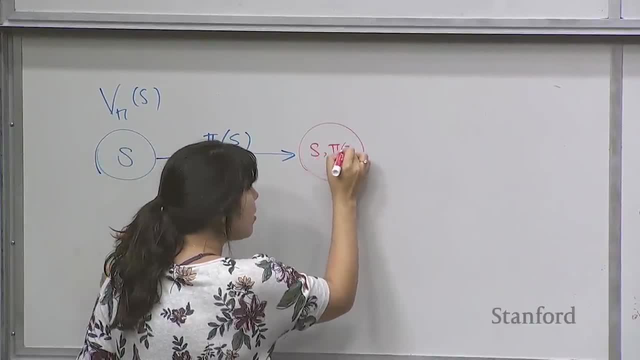 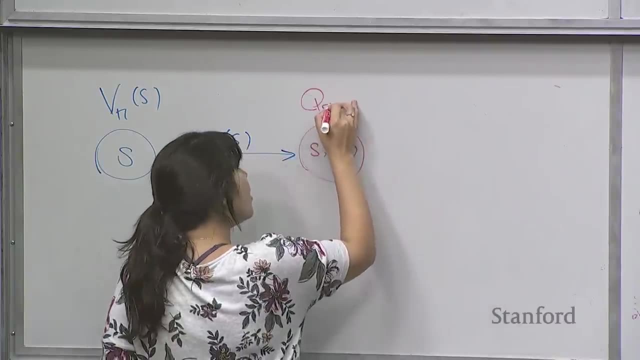 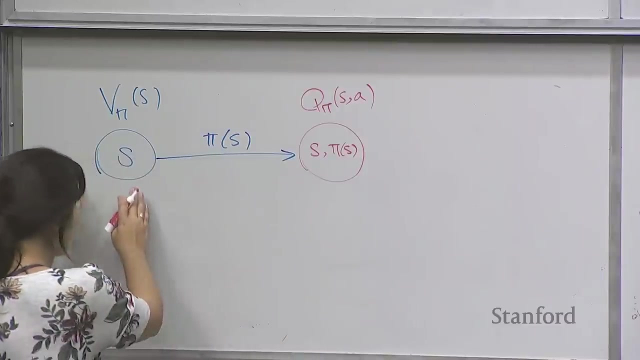 I've decided the action is pi of S, okay, And I've defined this new function, this q function, q, pi of S A, which is just the expected utility from the chance note okay. So so we've talked about value. 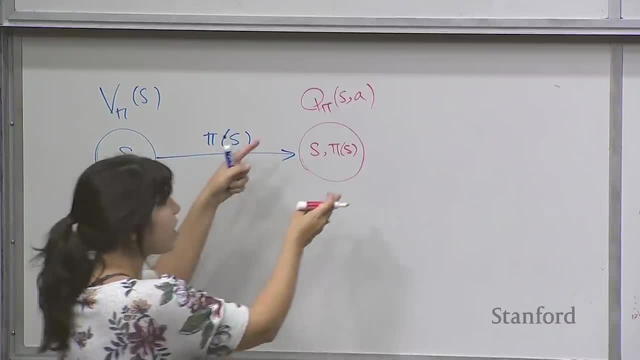 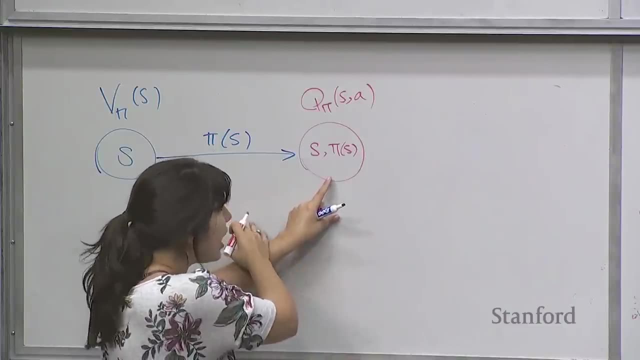 Value is expected utility from my actual state. I'm gonna talk about q values as expected utilities from the chance notes. So after you have committed that, you, you, you have taken action A and then you're following policy pi, then what is the expected utility from that point on? okay, 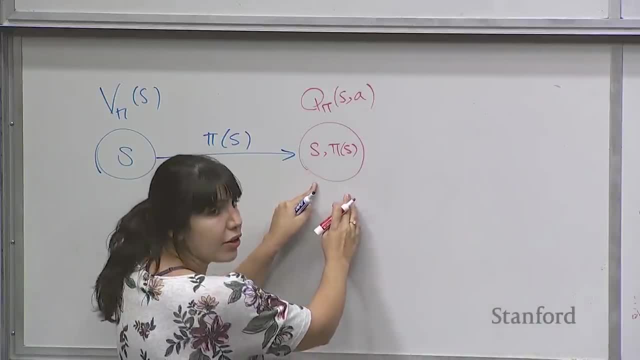 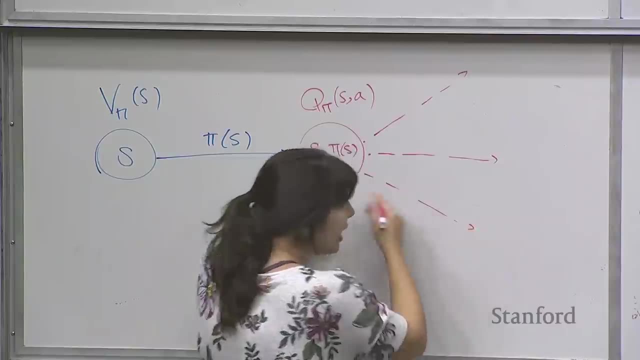 And well, what is the expected utility from this point on? We are in the chance note So many things that can happen, because I have like nature is going to play and roles die and anything can happen And they're gonna happen with transition. S A S prime. 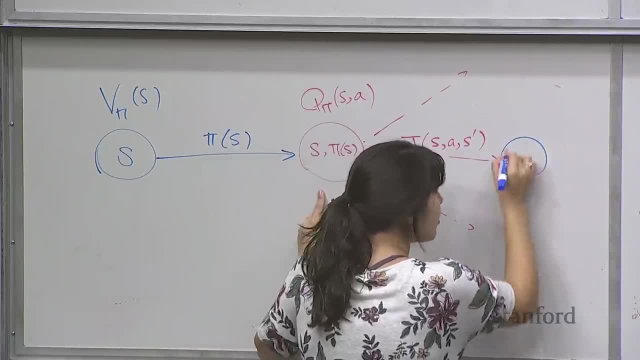 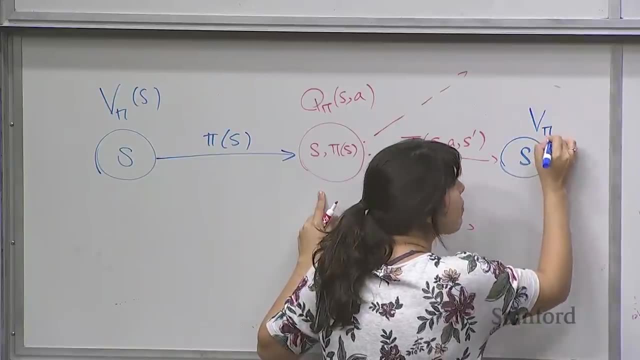 And with that transition probability I'm going to end up in a new state. I'm gonna call that S prime And the value of that state- again expected utility of that state- is v pi of S prime. okay, All right, So okay. 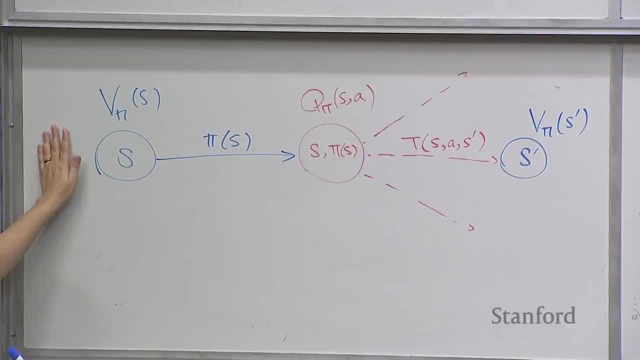 So what are these actually equal to? So I've just defined value as expected utility, q, value as expected utility from a chance. note What. what are they actually equal to? Okay, So I'm gonna write a recurrent that we're gonna use for the rest of the class. 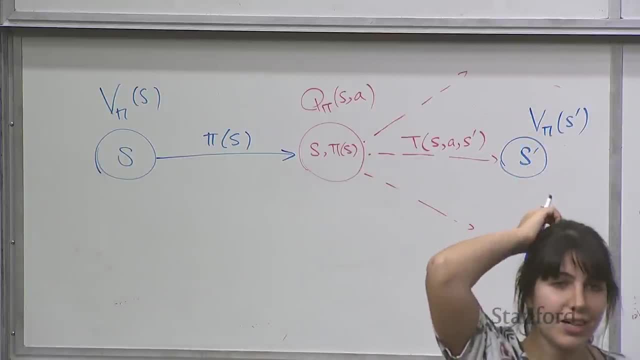 So pay attention for five seconds. There's a question there. I understand how, like semantically, uh v, pi, v pi are different, but in like actual, like number, like expected value, how are they different? So they're, both of them are expected value. 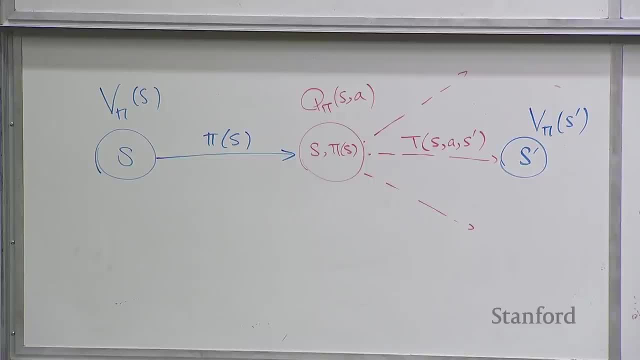 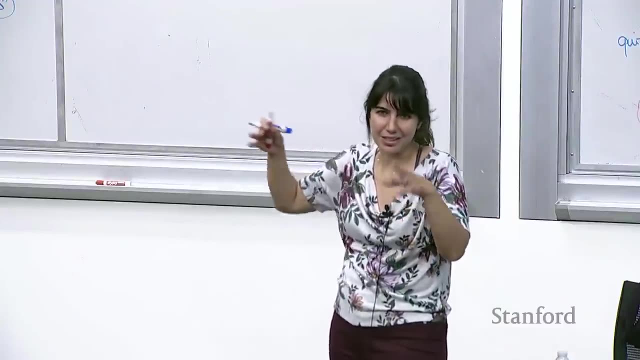 Yeah, So it's just. one is just a function of state. The other one you have committed to one action And the reason I'm defining both of them is to just writing. my recurrence is gonna be a little bit easier, uh, because I have this state action notes and I can talk about them. 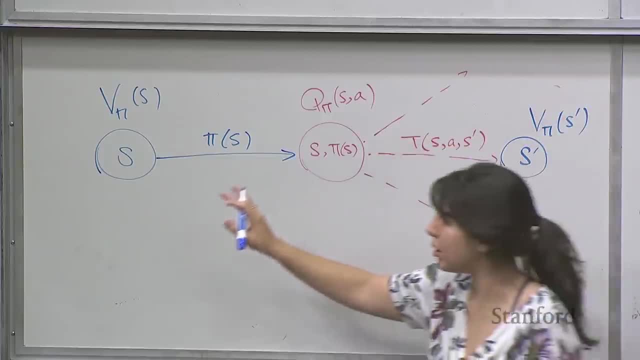 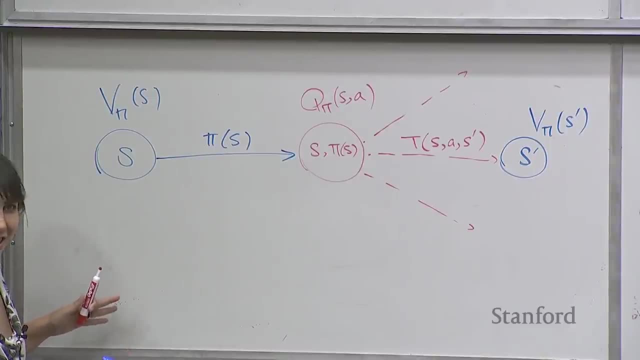 And I can talk about how like I get branching from these state action notes. okay, All right, So I'm gonna write a recurrence. It's not hard, but it's kind of the basis of the next like n lectures, So pay attention. 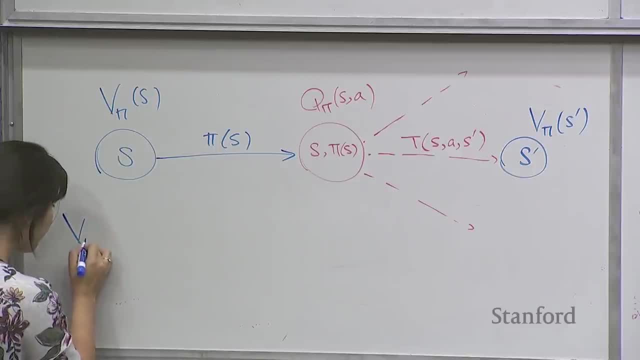 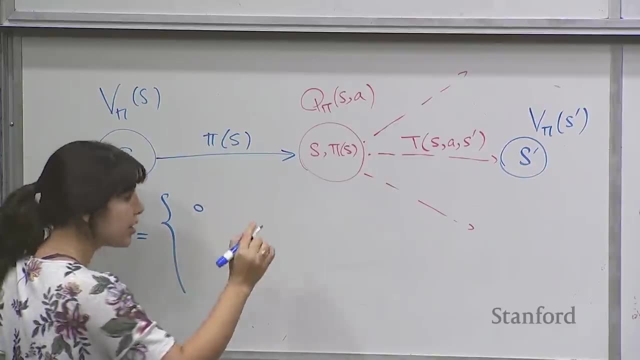 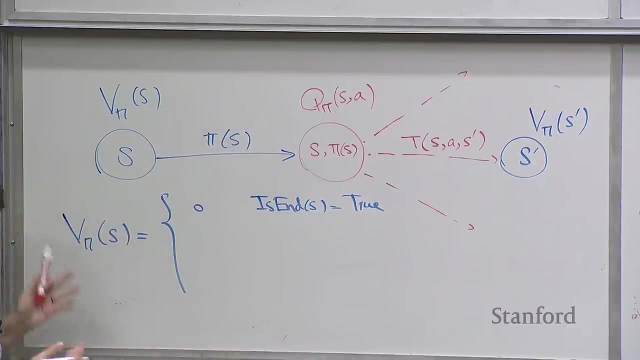 So, uh, all right, So v pi of s. what is that equal to? Well, that is going to be equal to 0 if I'm in an n state. So if is n of s is equal to true, then there is no expected utility. that's equal to 0.. 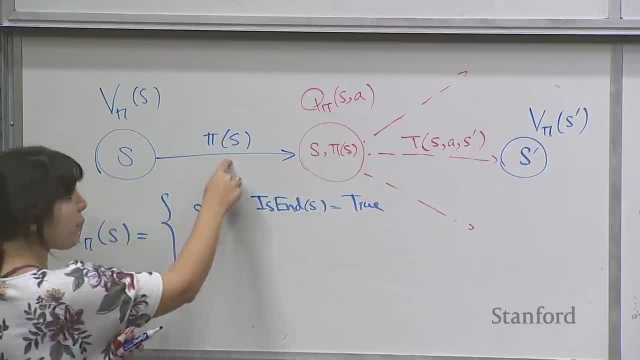 That's a easy case Otherwise. well, I took policy pi s. Someone told me take policy pi s, So value is just equal to q, right? So so in this case, v pi of s, if someone comes and gives me policy pi. 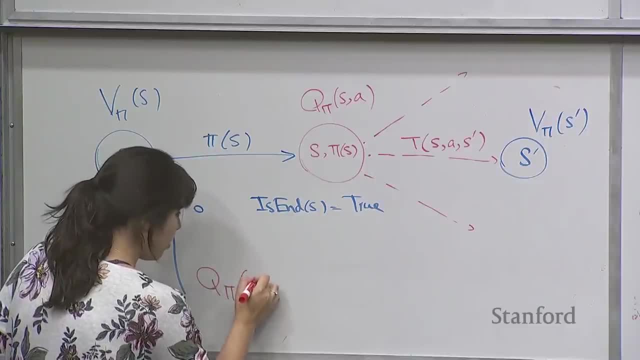 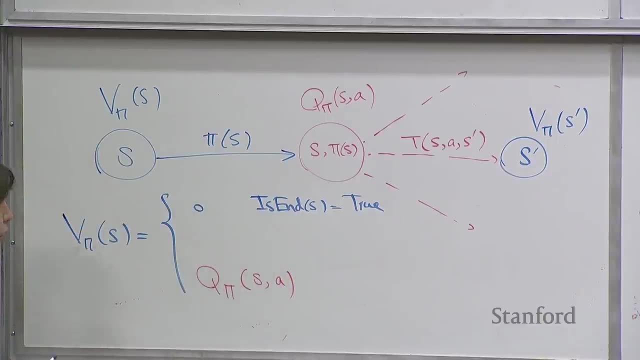 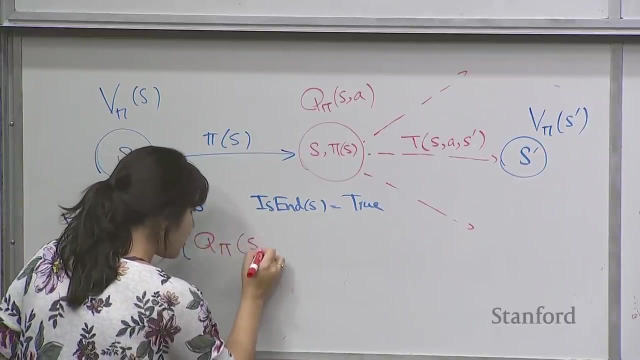 is just equal to q pi of s a. Okay, These two are just equal to each other. So the next question one might ask is actually: let me write these a little closer so I'll have some space. Yeah, So this is equal to q pi of s a. 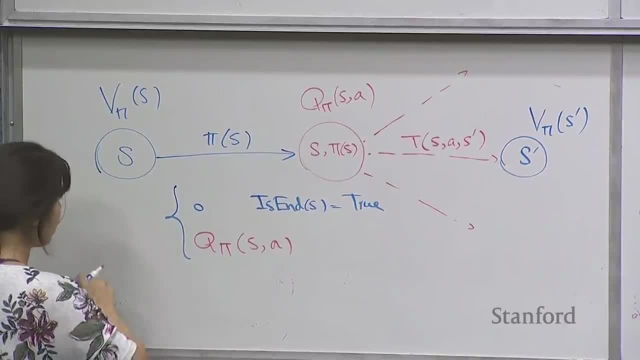 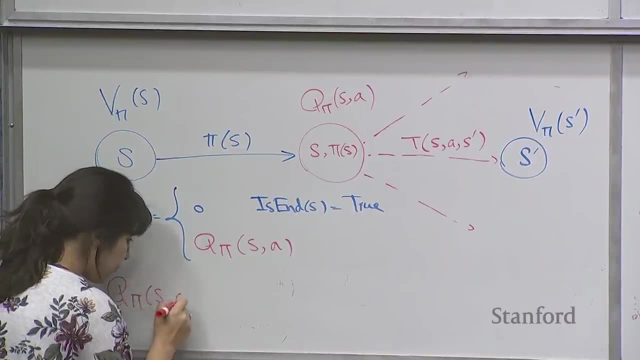 Okay, So so what is that equal to? What is q pi of s a equal to? So this is v pi of s. So now I just want to know what is q value, q pi of s a? What is that equal to? 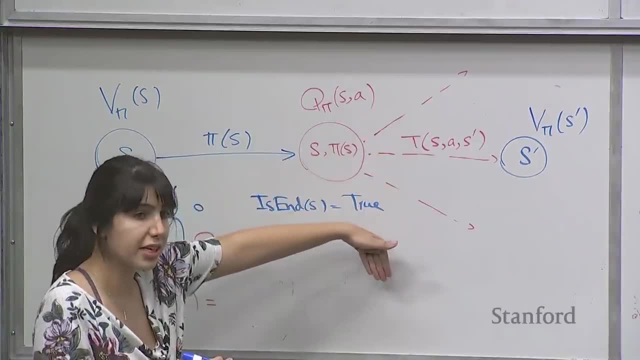 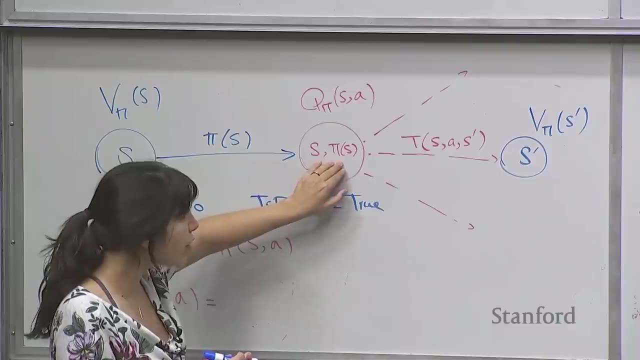 Okay. So if I'm right here, then there are a bunch of different things that can happen, right, And I can end up in these different s prime. So if I'm looking for the expected utility, then I'm looking for the probability of me ending up in this state. 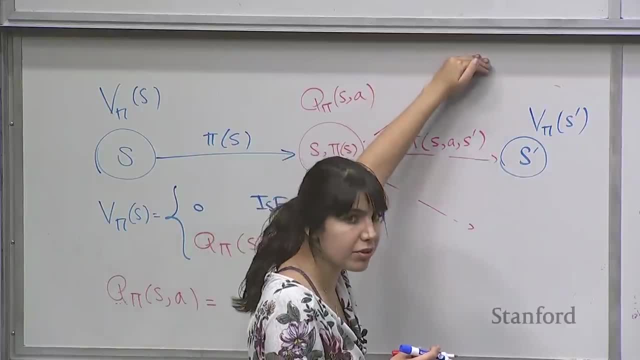 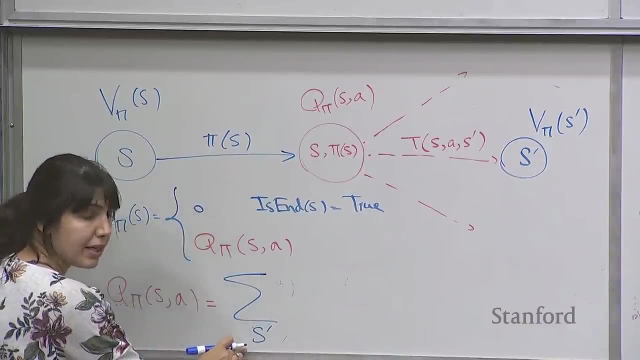 times the utility of this state, plus the probability of me ending up in a new state times the utility of that. So so that is just equal to sum over all possible s primes that I can end up at of transition probabilities of s a. 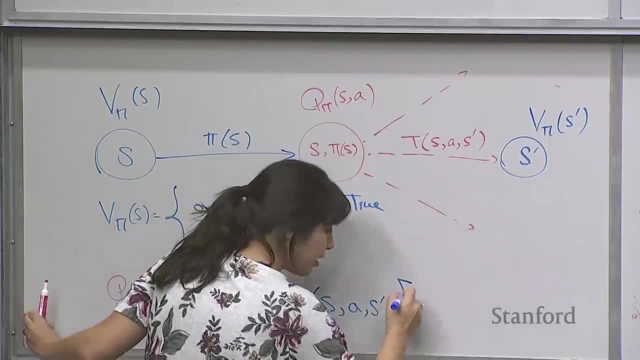 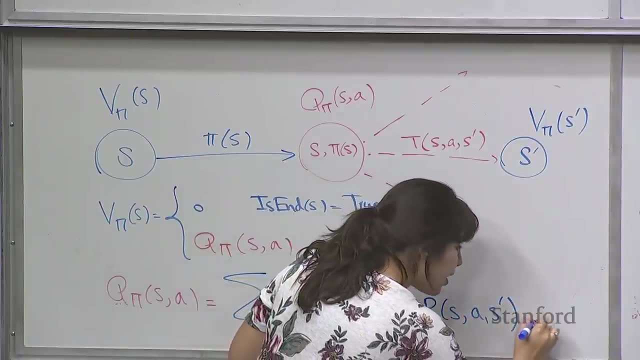 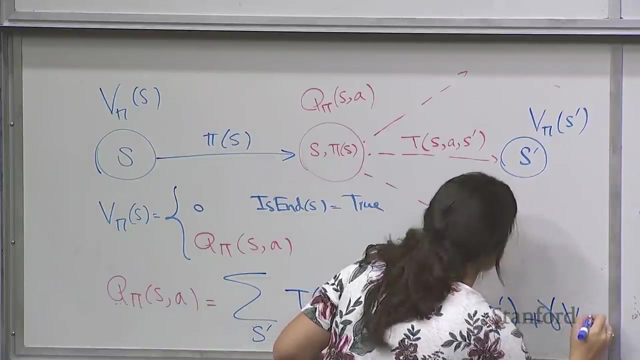 s prime transition probability of ending up in a new state times the immediate reward that I'm gonna get, reward of s a s prime plus the value here. but I care about the discounted value, So I'm gonna add gamma v pi of s prime. 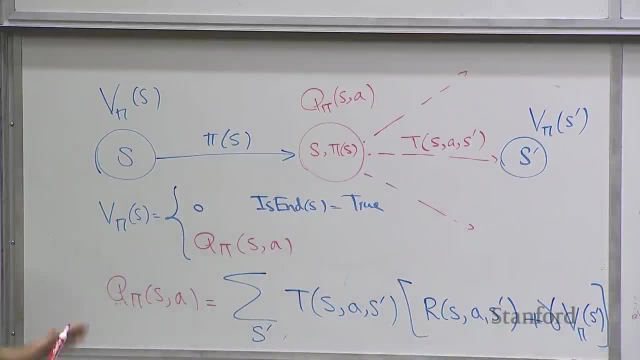 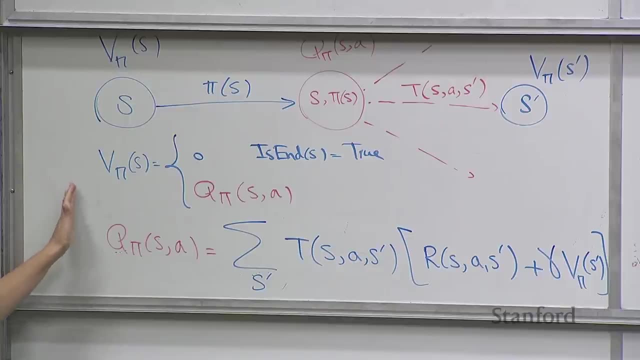 because I've been talking about this. this next state: Okay, Does this? does everyone see this? Okay, So this is the recurrence that we are doing in policy evaluation. Again, remember, someone came and gave me policy pi, So I'm writing this policy pi here. 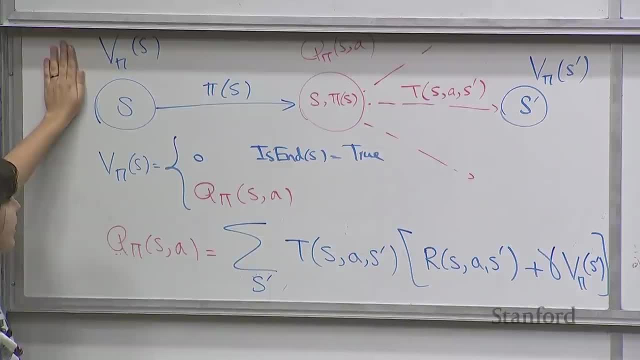 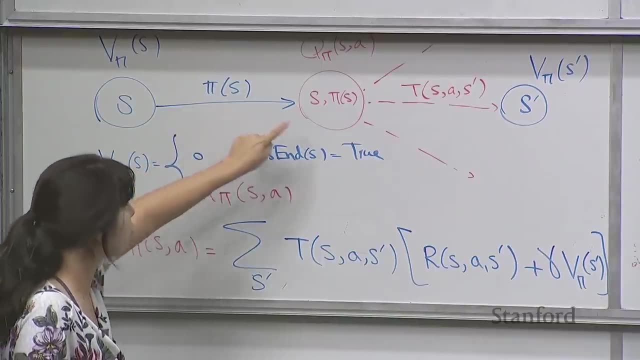 Someone gave me policy pi. I just wanna know how good policy pi is. I can do that by computing v pi. What is v pi equal to? Someone told me it's you're following policy pi, so it's gotta be equal to just q pi. 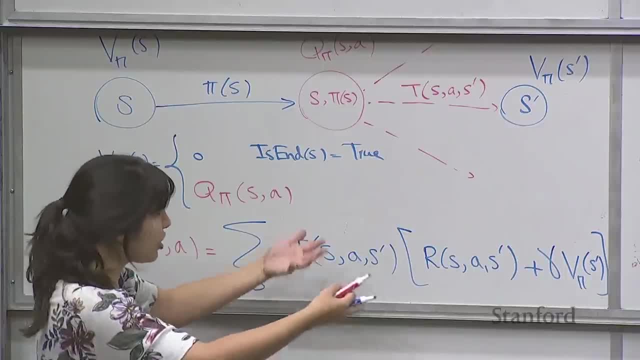 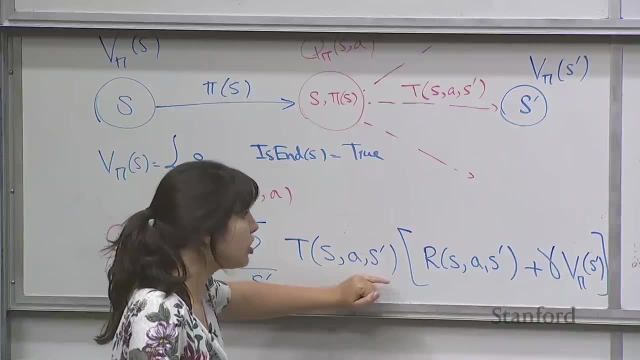 What is q pi equal to? It's just sum of all the like, the, the expectation of all the places that I can end up at. that sum over s primes, transition probabilities of ending up in s prime times, the reward, the total reward we are getting. 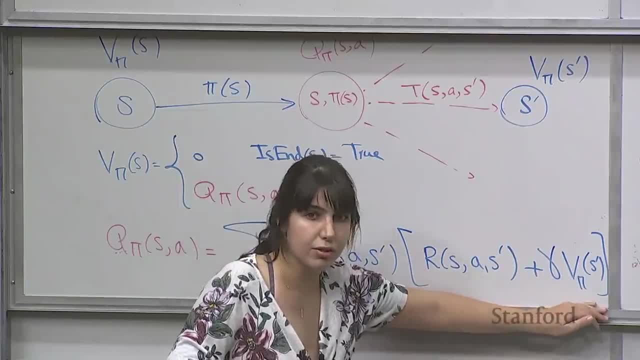 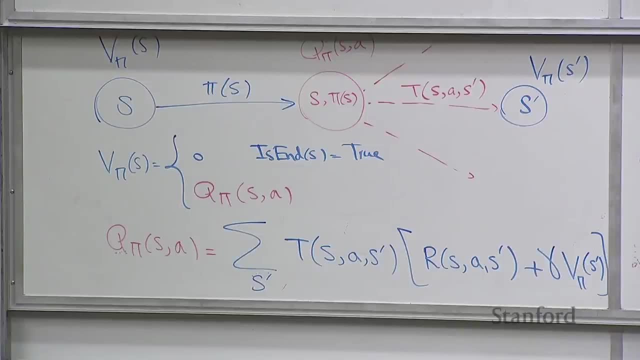 which is the immediate reward, plus discounting in my future. Okay, For the q values, and then, following policy pi, starting from s prime. Uh-huh, Yes, Yeah, yeah, yeah, yeah, Starting from s prime, All right. 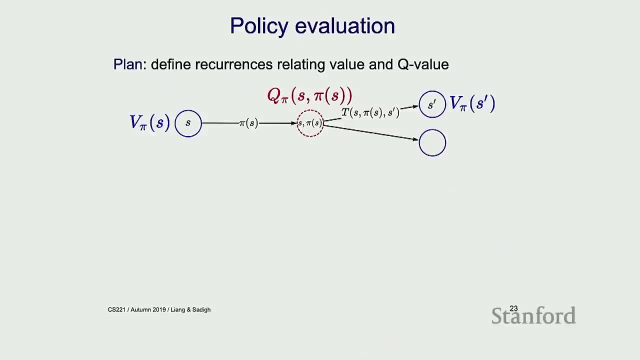 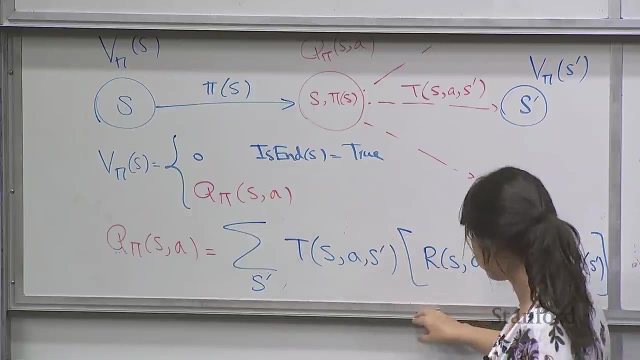 So okay, So far, so good. So so that is how I can evaluate this policy, right? So so I have these two recurrences. If I have these two recurrences, I can just replace this guy here, And let's imagine we are in the case. 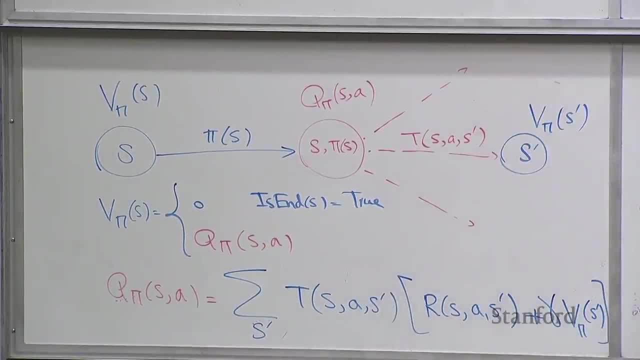 maybe I can use a different color up here. um in here, Okay, I'm just replacing. I'm just replacing this guy right here. I don't know if it's worth writing it. Imagine we are not in an end state. 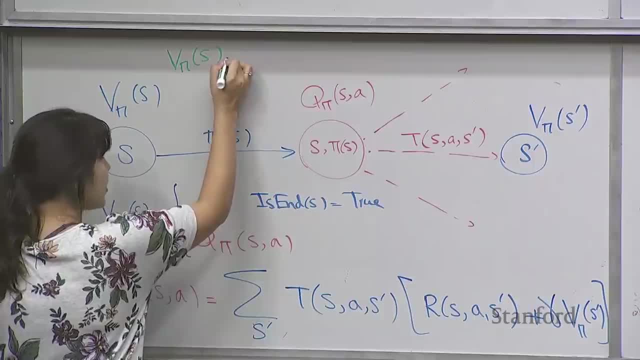 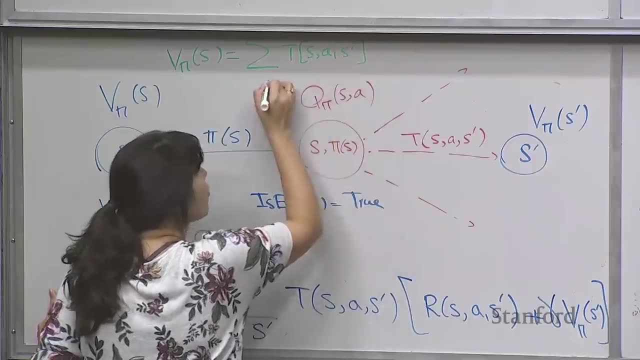 If you're not in an end state, then v pi of s. well, what is that equal to? That is just equal to sum of transition probabilities: s a s prime over s primes times. immediate reward that I'm gonna get. 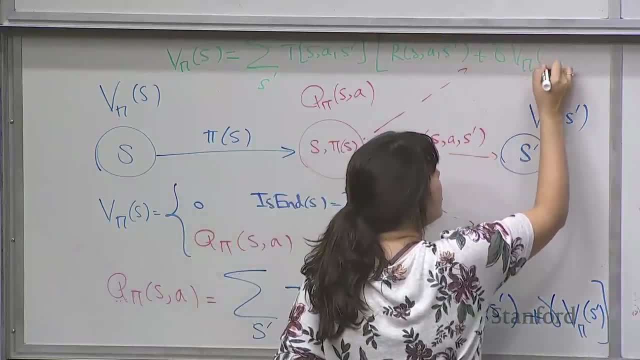 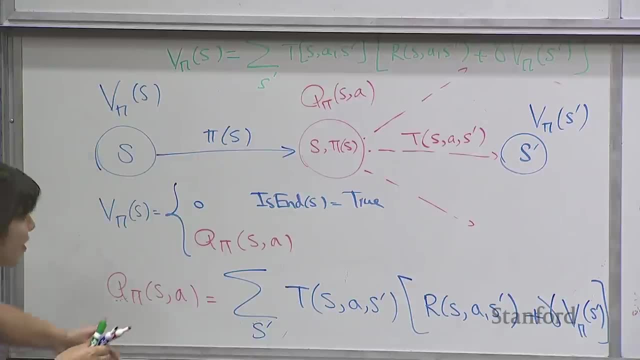 plus discounting v pi of s prime. Okay, So this is kind of the recurrence that I have. I, I, I literally just combine these two and wrote it in green: Okay, If you're not in an end state. So if you're not in an end state. 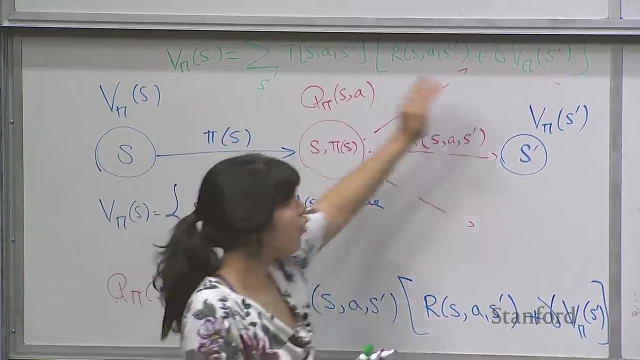 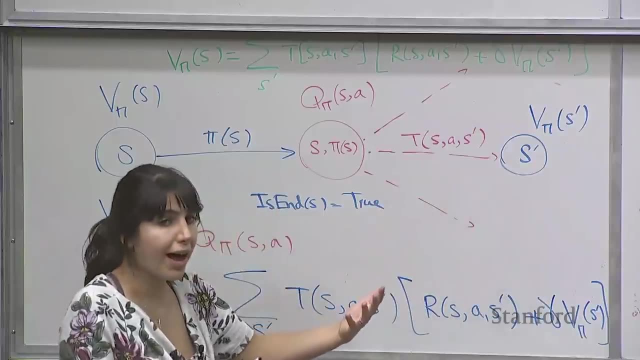 this is the recurrence I have. I have v pi here, I have v pi on this side too, So that is nice And and that is kind of the, the place where I can compute v pi. Maybe I can do it iteratively. 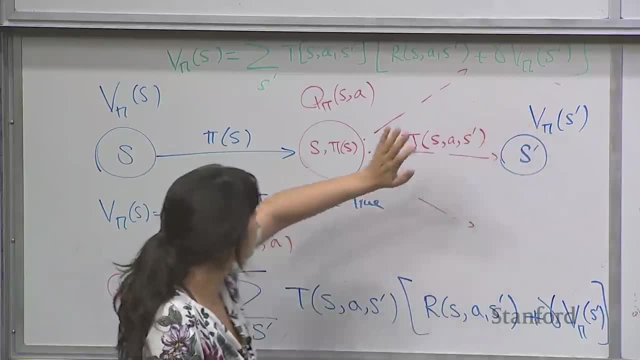 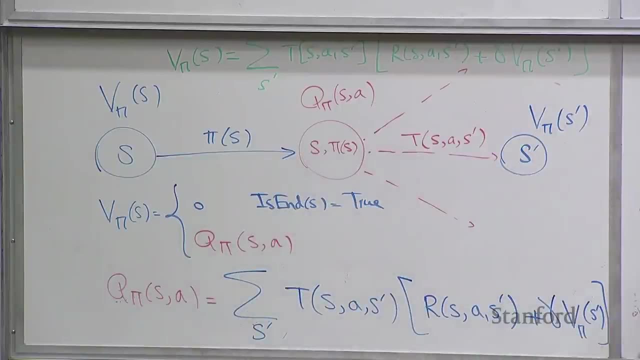 or maybe I can actually find a closed-form solution for some problems, But that is basically what I'm gonna do. I have v pi as a function that depends on v pi of s prime and I can just solve for this v pi Okay, And that allows me to evaluate um. 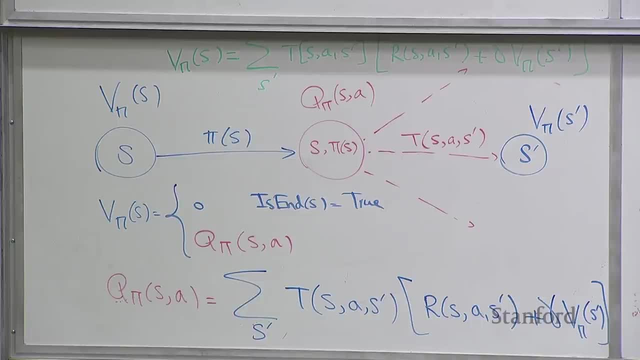 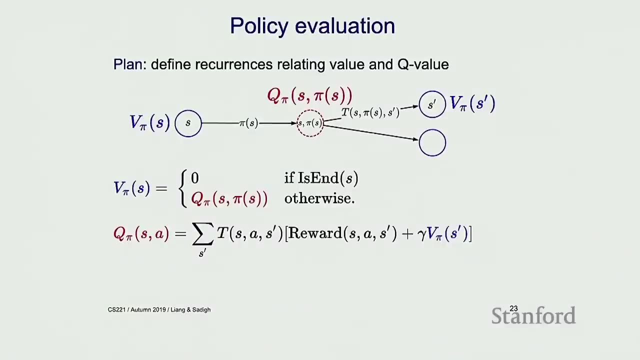 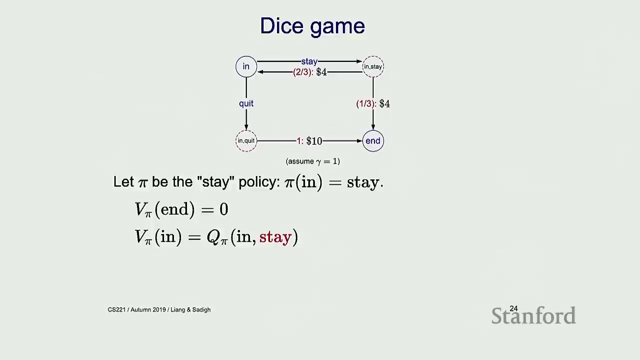 to evaluate policy pi. I haven't figured out a new policy. All I have done is evaluating what's the value of pi. Okay, All right, Okay, So let's go back to this example. So let's say that someone comes in and tells me: 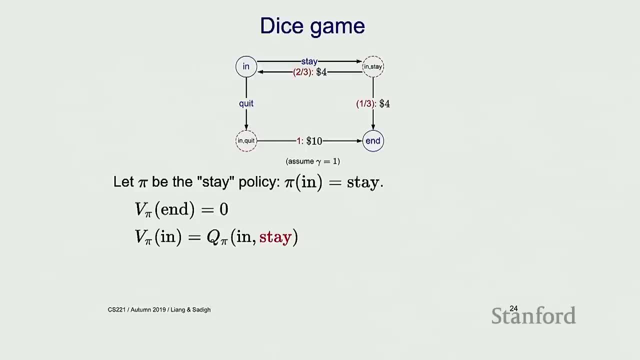 well, the policy you gotta follow is is stay. So my policy is is to stay. Okay, I wanna know. I wanna just evaluate that. I wanna do policy evaluation. When you're doing policy evaluation, you gotta compute that v? pi for all states. 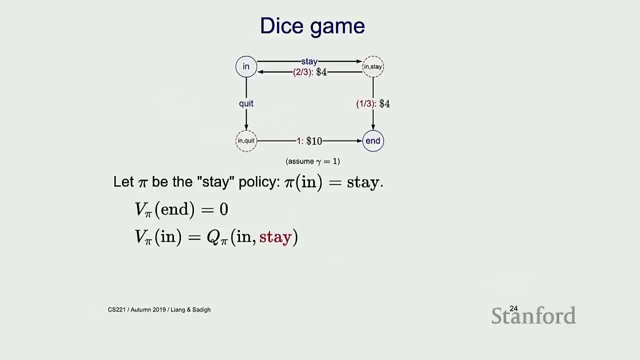 So let's start with v pi of n. Well, that is equal to 0, because we know v pi at n state is just equal to 0.. Now I wanna know what's v pi of of n Okay State n. What is that equal to? 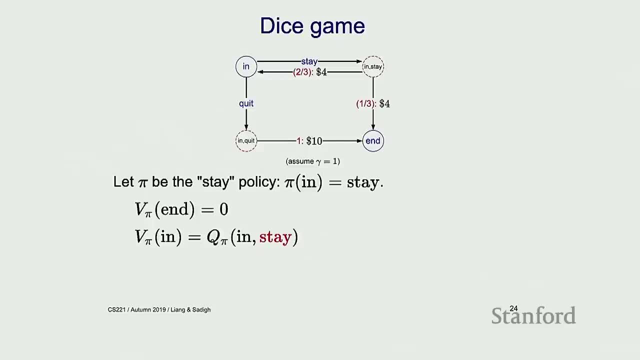 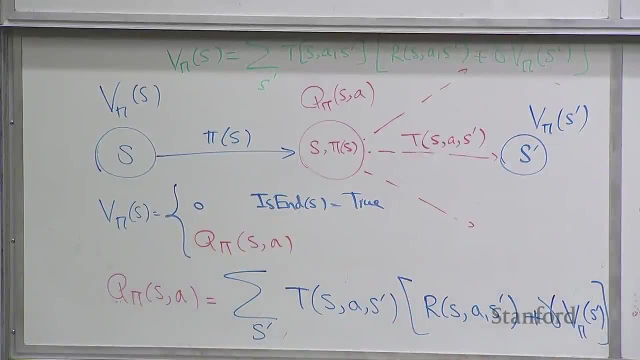 That's just equal to q pi of n, and stay right, V pi is just equal to q pi of n and stay, So I'm gonna replace that. That's just equal to one-third. Okay, So I'm gonna replace that. That's just equal to one-third. 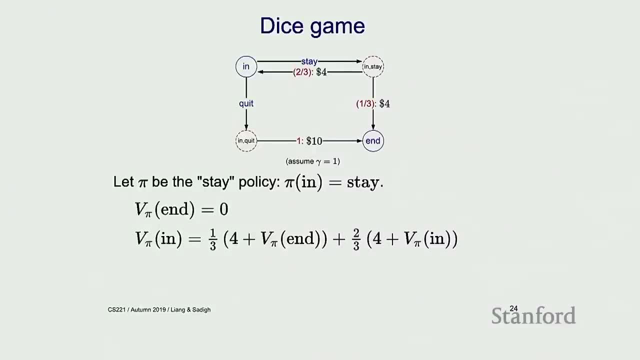 Two-thirds times immediate reward, which is four plus value of the next state I'm gonna end up at, which is n in this case, plus two-thirds times the immediate reward I'm gonna get, which is $4, plus value of the state I'm gonna end up at, which is n. 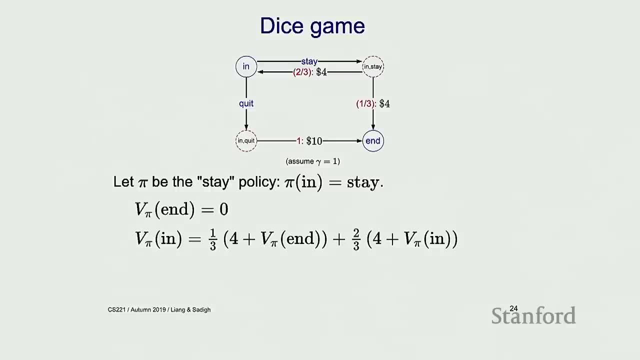 Okay, So. so that is just that sum that we have there. All right, V pi of n is 0.. So let me just put that 0 there. I'm gonna put 0 there. I only have one state here too, right. 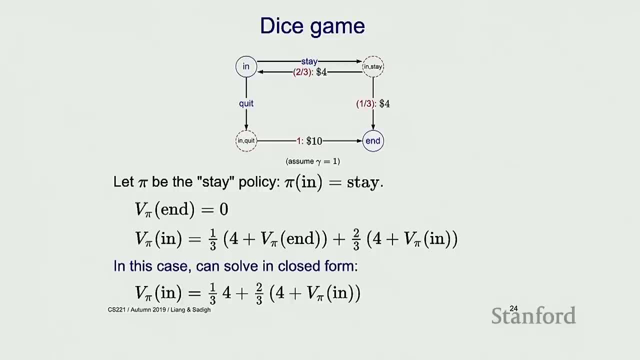 So I just have this as a function of this one state, n. So I have an an equation. I can find the closed-form solution of V pi of n. I'm just gonna move things around a little bit and then I'll find out that V pi of n is just equal to 12.. 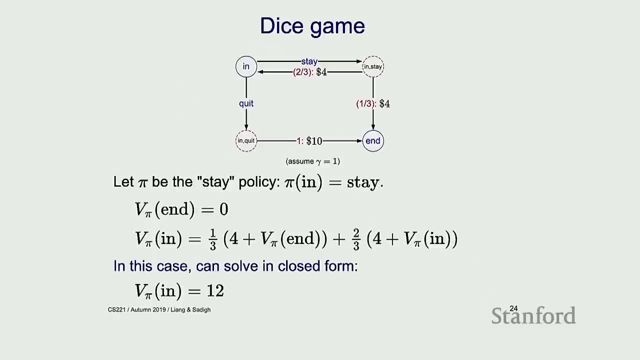 So so that's how you get that 12 that I've been talking about. So so you just found that that if you tell me the policy to follow is stay, if that is the policy, then the value of that policy from state n is equal to 12.. 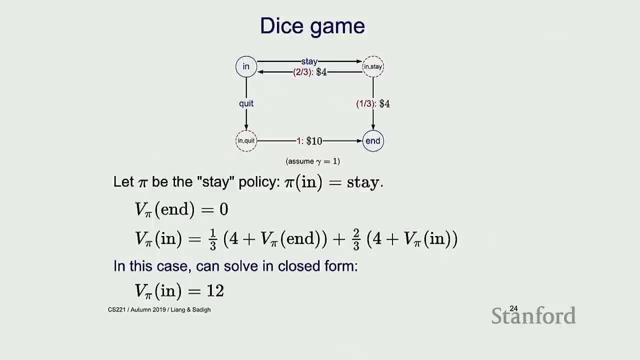 Do you think that some of you always choose the same policy? All right, Some of you always choose the same, Yeah, So so the policy is a function of state. I only have this one state that's interesting here, right, That that's one state is n. 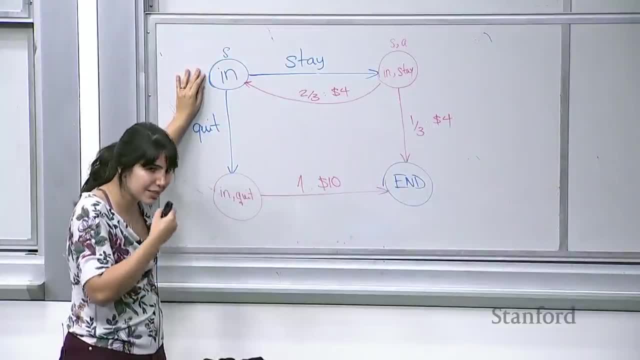 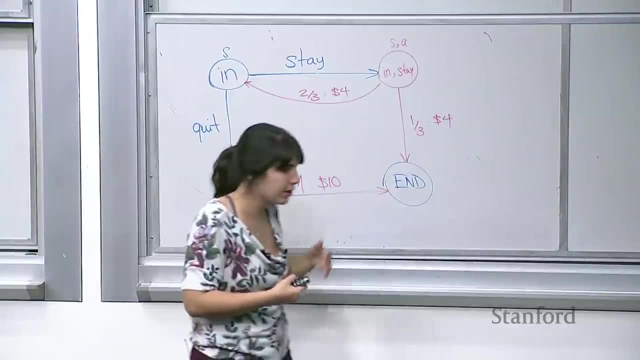 So I need to, when, when I define my policy, I need to kind of choose the same policy for, for, for, for that state right, My policy says: in n you, you gotta either stay or you gotta either quit, quit. 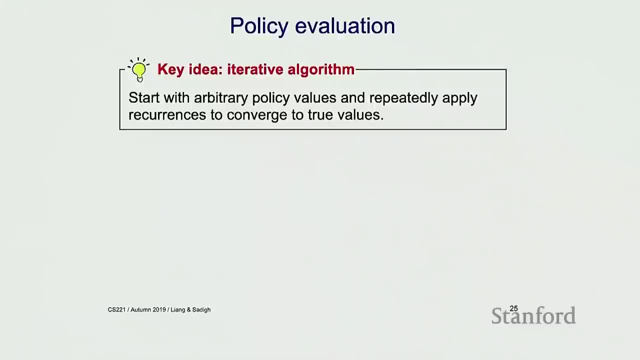 All right, So you can basically do the same thing using an iterative algorithm too. So so here, like in the previous example, it was kind of simple. I just solved the closed-form solution, But in in reality, like you might have different states and then it might be a little bit more complicated. 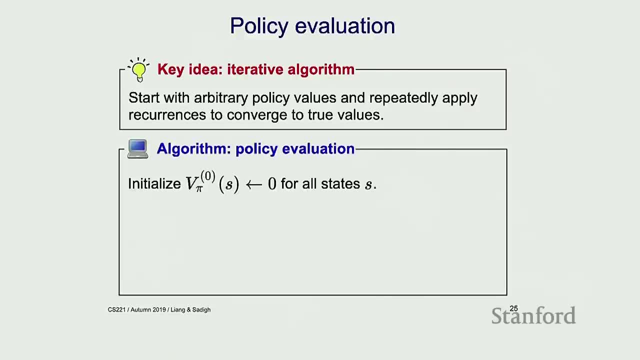 So we can actually have an iterative algorithm that allows us to find these v pies. So the way we do that is, we start with the values for all states to be equal to 0. And, and this 0 that I put here is the first iteration. 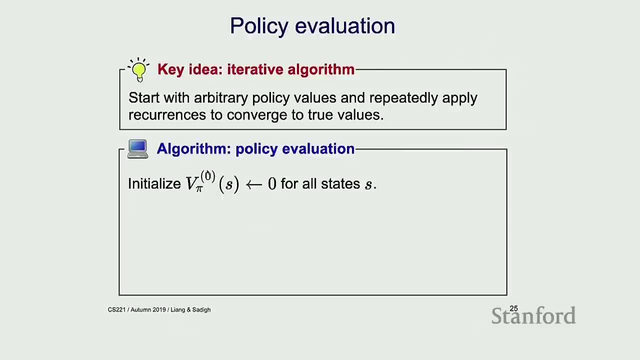 So so I'm going to count my iterations here. So so I'm gonna just initialize all the values for all states to just be equal to 0,. okay, Then I'm just gonna iterate for some number of time, whatever number I care, like I would like to. 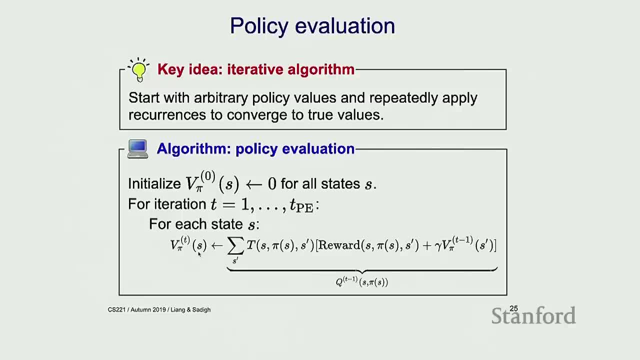 Then what I'm gonna do is, for every state- again, remember, the value needs to be computed for every state. So for every state, I'm gonna update my value by the same equation that I have on the board. okay, And the same equation depends on the value at the previous time step. 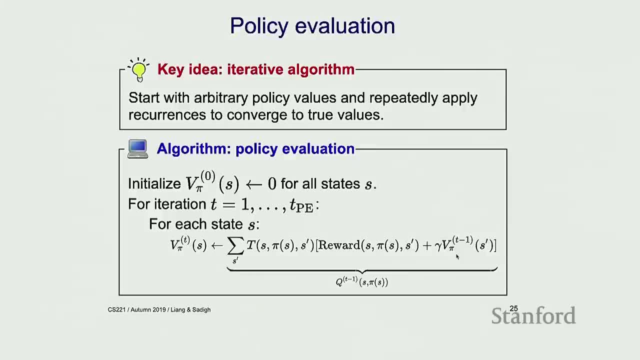 So this is just an iterative algorithm that allows me to compute new, old values based on previous values that I've had, And I started with, like everything, 0, and then I keep updating values of all states and they keep going. So basically that equation. 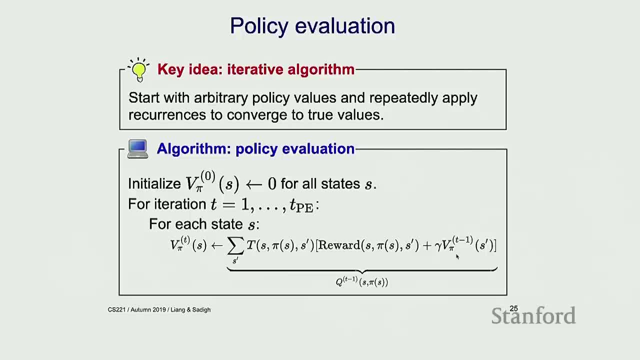 but think of it as like an iterative update every round. So you, you're done. you run this for multiple rounds. Every round you just update your value, okay, So like here is just a pictorially looking at it. Imagine you have like 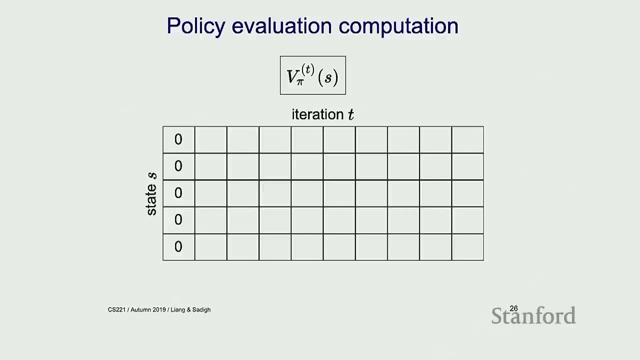 five states here. you initialize all of them to be equal to 0. The first round you're going to get some value, you're going to update it and then you're going to keep running this and then eventually you can kind of see that. 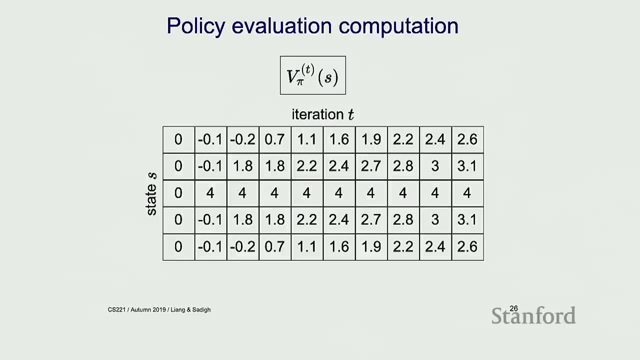 the last two columns are kind of close to each other and you have converged to the true value. So so again, someone comes and gives you the policy. You start with values equal to 0 for all the states and then you just update it based on your previous value. 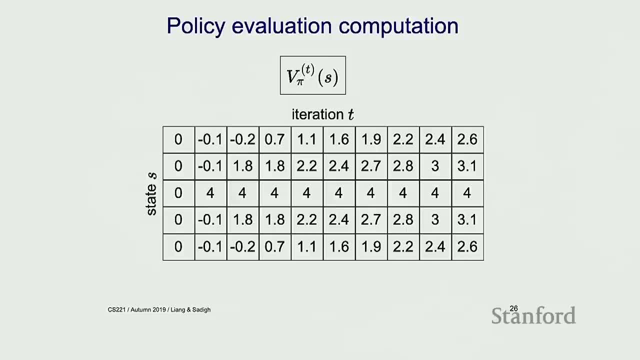 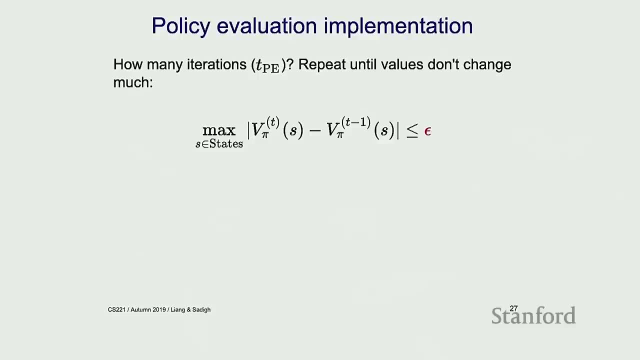 Okay, So how long should we run this? Well, we have a heuristic to to kind of figure out how long we should run this particular algorithm. Uh, one thing you can do is you can kind of keep track of the difference between your value at the previous time step versus this time step. 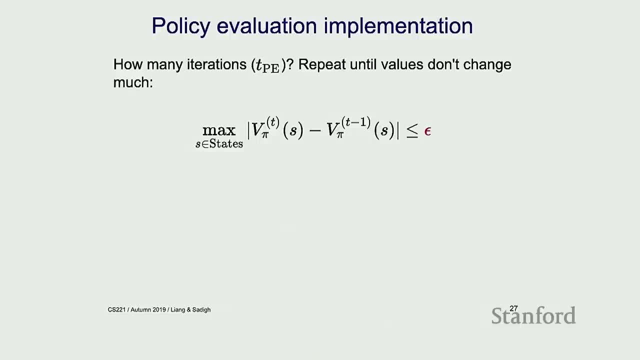 So. so if the difference is below some threshold, you can kind of call it, call it done and then say, well, I've, I've found the right values. And then in this case we are basically looking at the difference between value at iteration t. 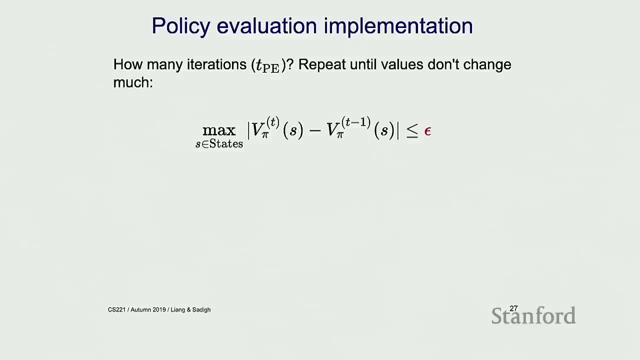 versus value at iteration t minus one, And then we are taking the max of that over all possible states because I want the values to be close for all states. Okay, Yes, Is this going to be the first one of these? Is this here? So? so I'm going to talk about the convergence. when we talk about 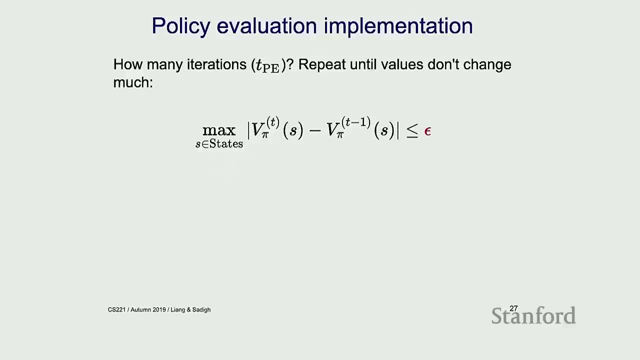 the gamma factor, and then the, the discount factor, and um, a-sequelicity, Um. also, how long you should run this to get these is also a difficult problem and it depends on the properties of your MDP. So if you have an ergodic, if you have an ergodic MDP, 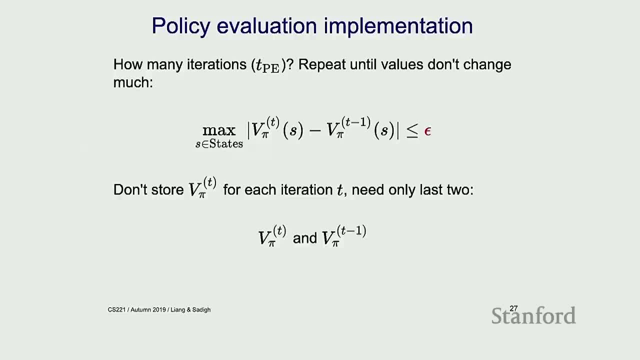 this is sh-. this should work Okay, But in general it's a hard problem to answer for general Markov decision pro- processes: Okay. And another thing to notice here is I'm not storing that whole table, Like the only thing I'm storing is. 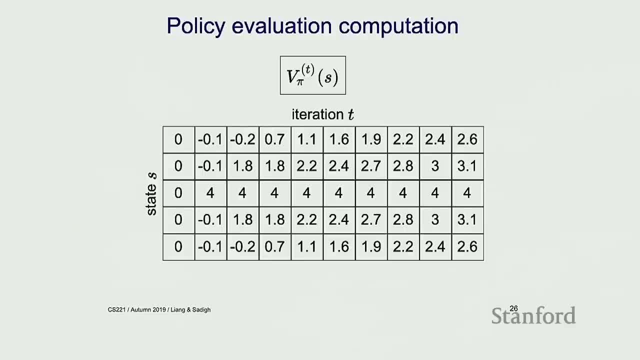 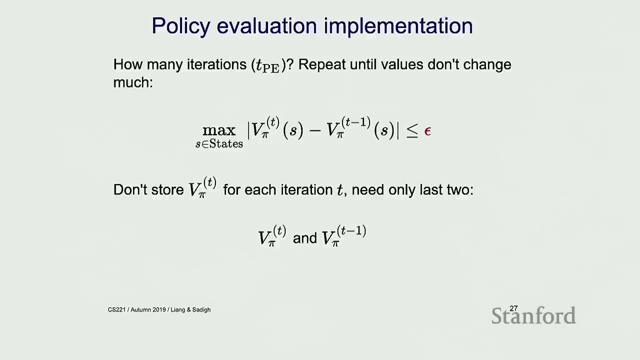 is the last two columns of this table, Because, because that's v pi at iteration t and v pi at iteration t minus one, Those are like the only things I'm storing, Because that allows me to compute if I've converged and that kind of allows me to keep going because I only need my previous value. 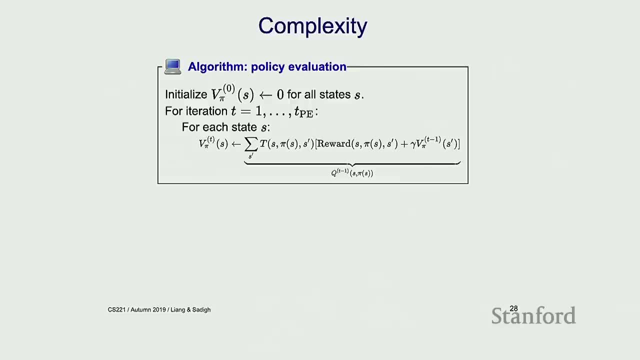 It's to update my new values Right In terms of complexity. well, this is gonna take order of t times s times s prime. Well, why is that? Because I'm iterating over t times steps and I'm iterating over all my states. 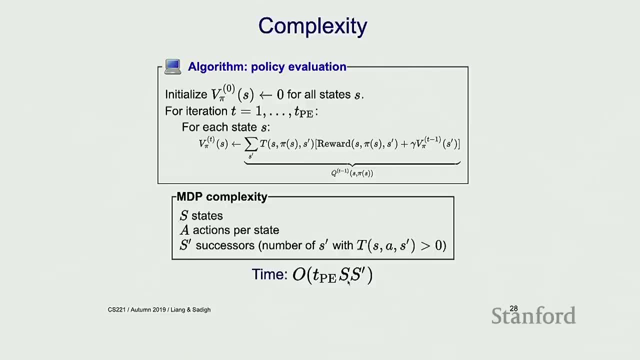 and I'm summing over all s primes, right. So so, because of that, that's a complexity I get, And one thing to notice here is it doesn't depend on actions, right, It doesn't depend on the size of actions. 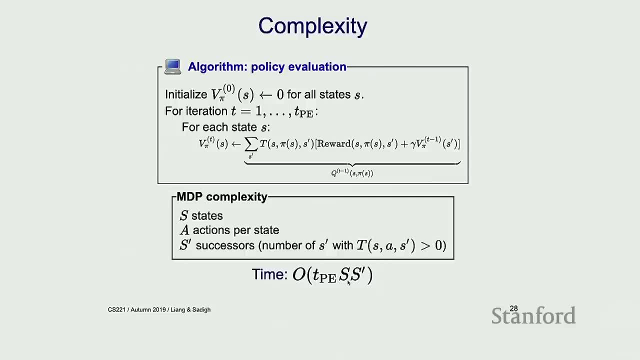 And the reason it doesn't depend on the size of actions is you have given me the policy. You're telling me follow this policy. So if you've given me the policy, then I don't really need to worry about like the number of actions I have. okay. 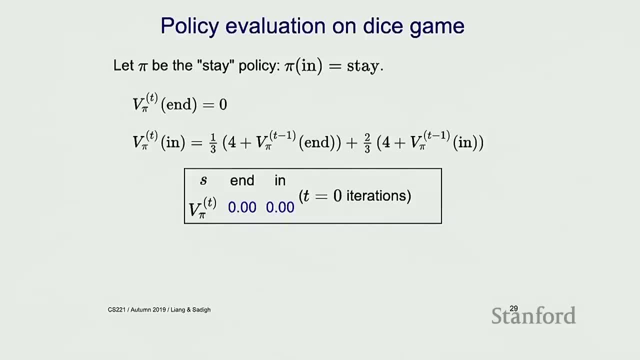 All right, Um, here is just another like like the same example that we have seen. So, at iteration t, equal to one, n is going to get four, n is going to get zero. At iteration two, it gets a slightly better value. 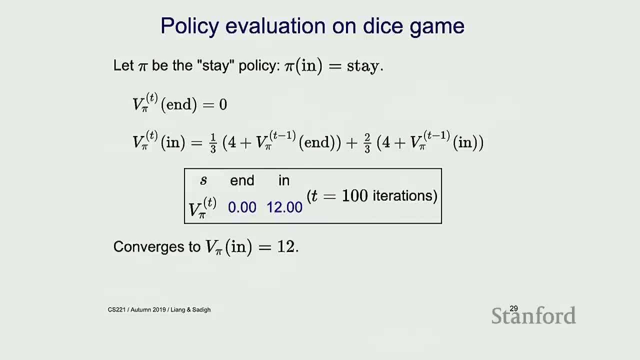 And then finally, like iteration, like 100, let's say we get the value 12.. And, and remember, for this particular example, like this example, we were able to solve it like: solve the closed form v v of uh v v of policy staying. 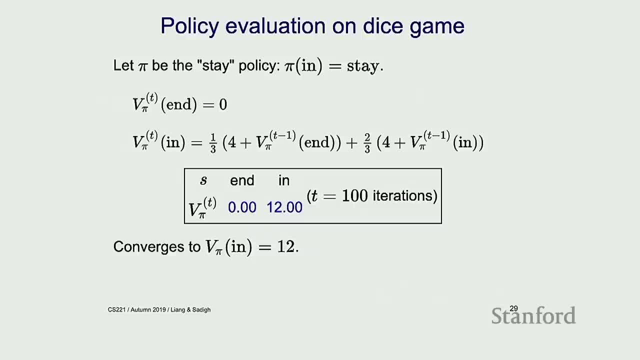 uh from state n, But uh, but you could also run the iterative algorithm and get the same value of 12.. Okay, Yes, The number of actions is just the size of s prime. right, The number of uh actions is the size of s prime. 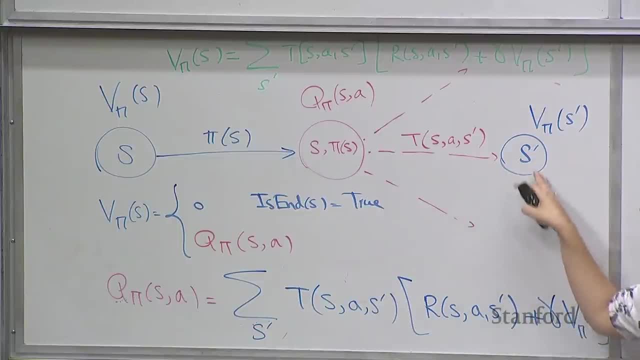 Uh, no, because the size of s you might end up in very different different states. This depends on your probabilities. Oh, okay, The size of s prime is actually the size of. like, the size of states is the same thing, right? 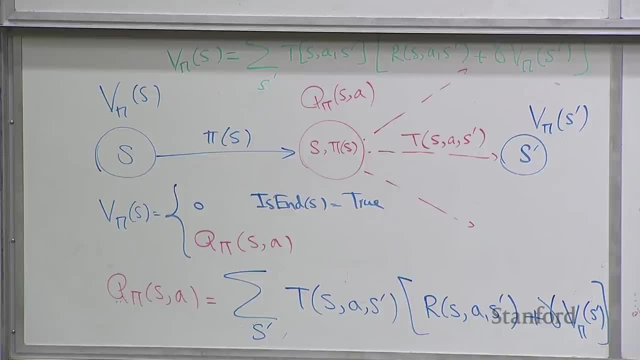 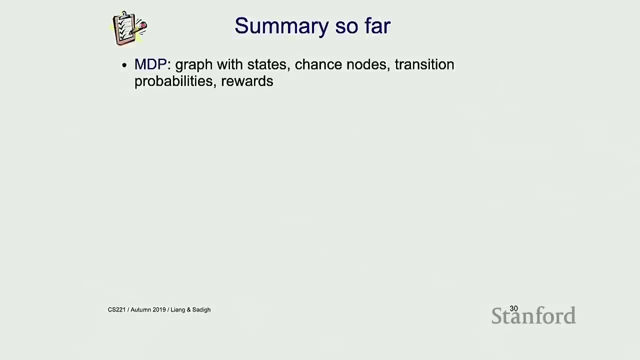 Like it's worst case scenario. you're going from every state to every state, So just imagine the size of s. Okay, All right. So summary: so far, where are we? So we have talked about MDPs. These are graphs with states and chance nodes and transition probabilities and rewards. 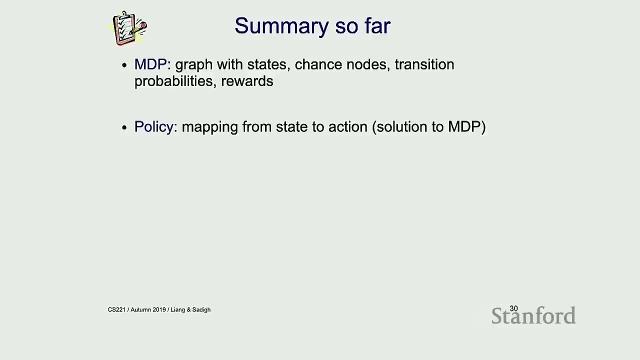 And we have talked about policy as the solution to an MDP, which is this function that takes a state and gives us an action. Okay, We talked about the value of a policy. So value of a policy is the expected utility of of that policy. 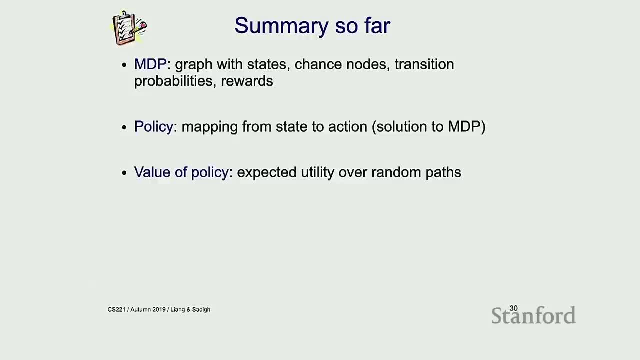 So. so if you talk about utility, like you, you have these random values for all these random paths that you're gonna get for every policy. The value of utility is just an expectation over all those random, random variables. And so far we've talked about this idea of 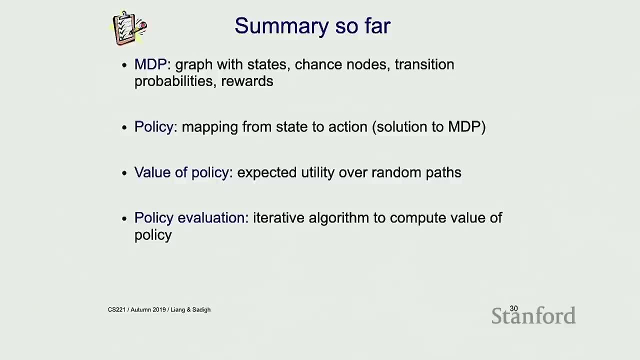 a policy evaluation, which is just an iterative algorithm to compute what's the value of a state if you give me some policy, Like, how good is that policy? What's the value I'm gonna get at every state? Okay, All right. So that has been all, assuming you give me the policy. 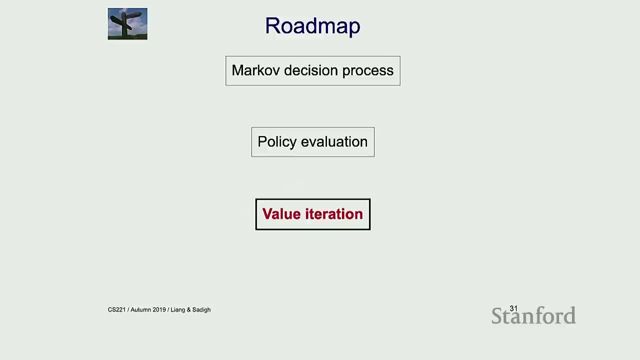 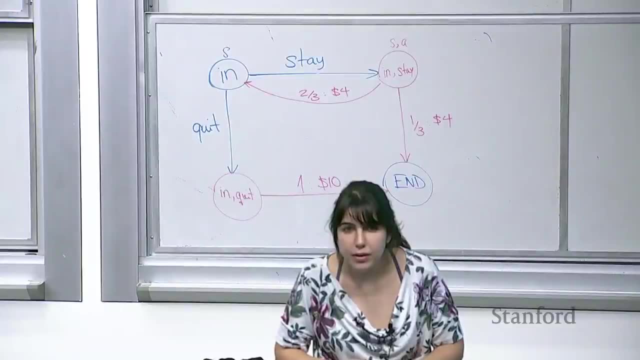 Now the thing I want to spend a little bit of time on is is figuring out how to find that policy. Um, is it possible that we learn new actions for a problem that's going to change the value of the policies? We learn new actions. 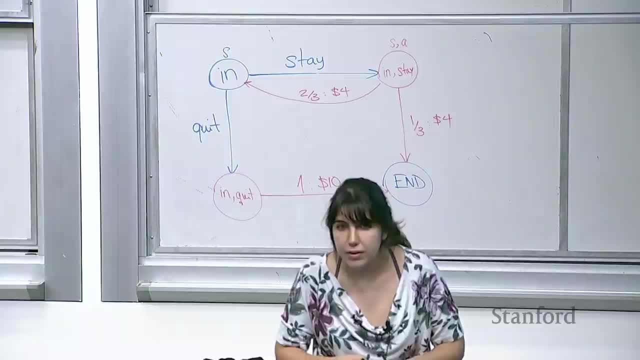 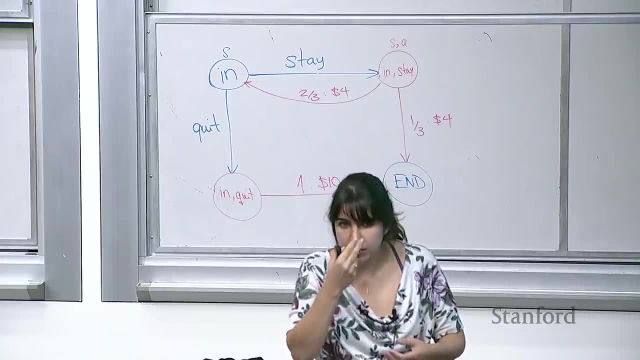 So, for example, here we only have a stay or quit, Like if we have a different problem, that we can learn another action like stay, quit or something um, um trade, Uh-huh. Is it going to change the value of the policies? 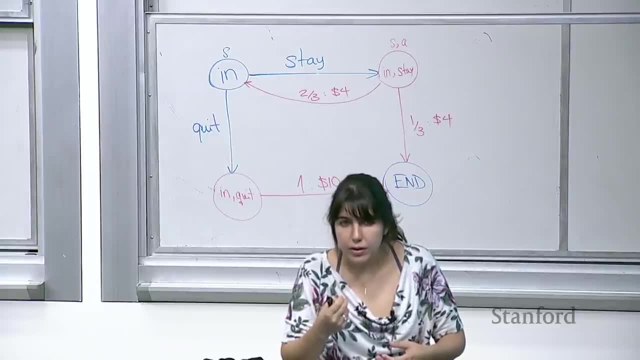 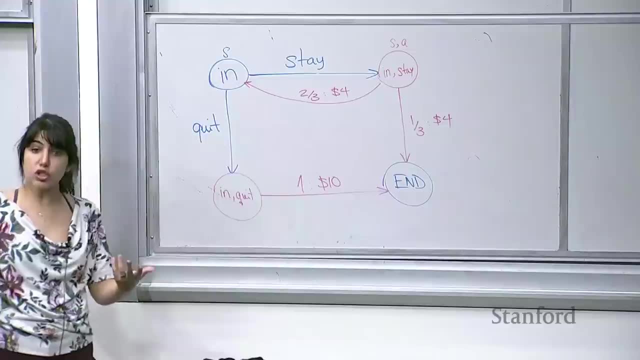 Because then we have a new action and then we need to update our policies. So in this case, so so so far, I'm assuming that the set of actions is fixed. I'm not like adding new actions right Like the way, even with search problems. 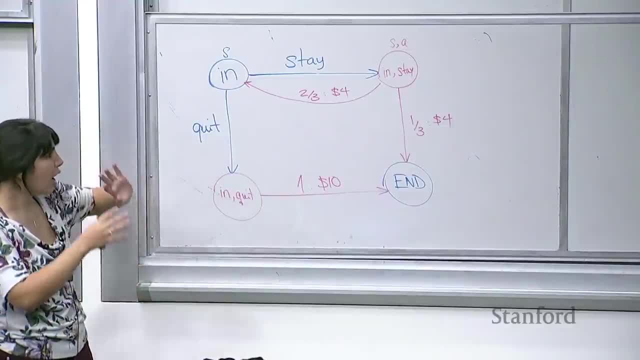 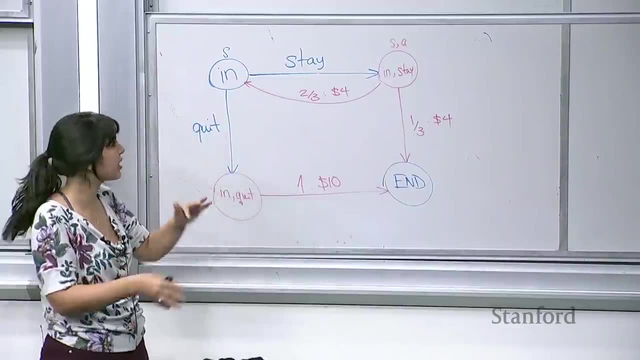 like the way we define search problems or the way we are defining MDPs, is, I'm say, like I'm starting with a setup where states are fixed, actions are fixed. I have stay and quit. Those are like the only actions I can take. 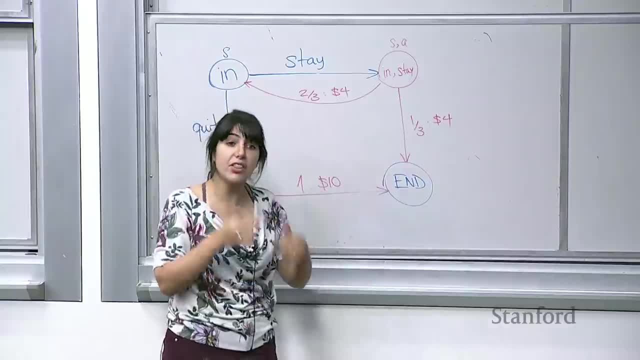 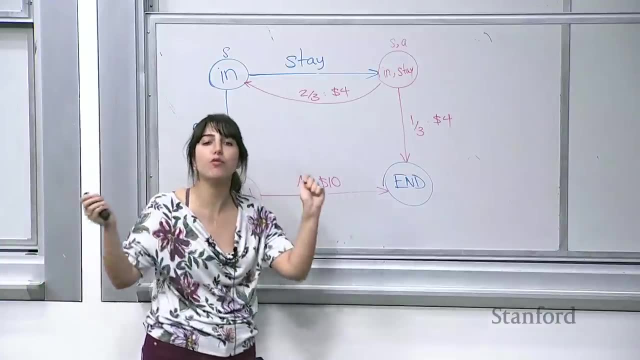 Uh, the reward is fixed. uh, transition probabilities are fixed. under that scenario, Then what is the pest-? the best policy I can take, And best policy, is just from those set of like already defined actions. okay, Um, next lecture we'll talk about unknown settings. 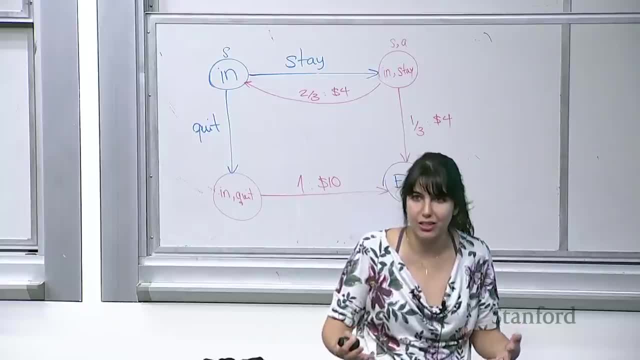 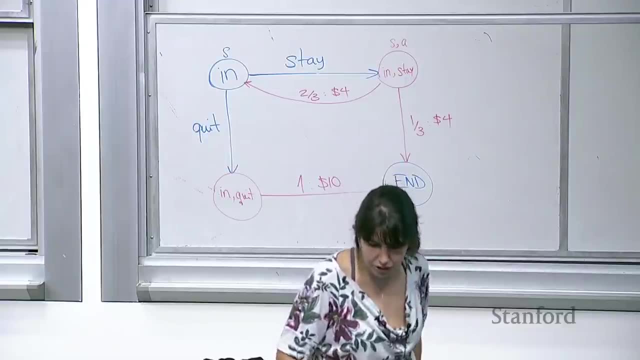 like when we have transition probabilities that are not known or reward functions that are not known and how we go about learning them, And that that would be the reinforcement learning lecture. So next lecture I might address some of this. Okay, All right, So let's talk about value iteration. 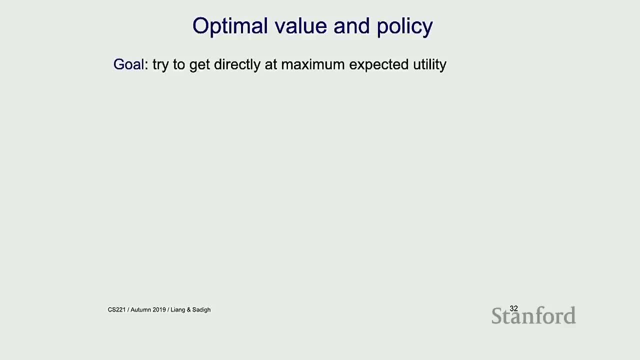 So so that was policy evaluation. So, like, that whole thing was policy evaluation. So now what I'd like to do is I wanna try to get the maximum expected utility and find the set of policies that gets me the maximum expected utility. okay, 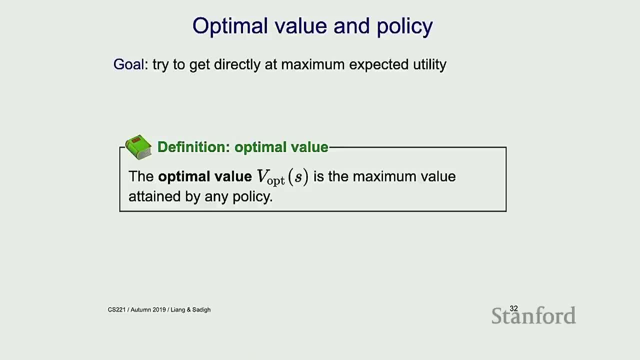 So to do that, I'm gonna define this thing that's called an optimal value. So instead of value of a particular policy, I just want to be Opt of S, which is the maximum value attained by any policy, So so you might have a bunch of different policies. 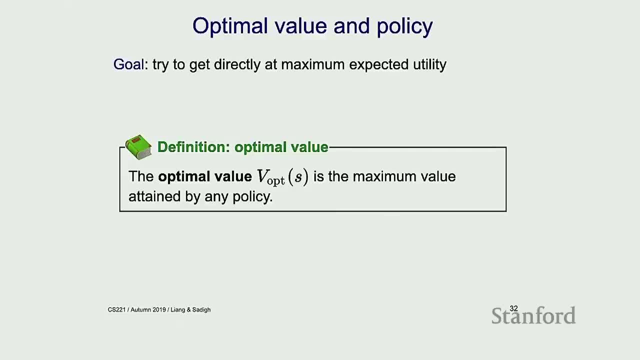 I just want that policy that maximizes the value- okay, So, and that is the Opt of S- okay So, um, so let me go back to this, to this example. So I'm gonna have this in parallel to this example of policy evaluation. 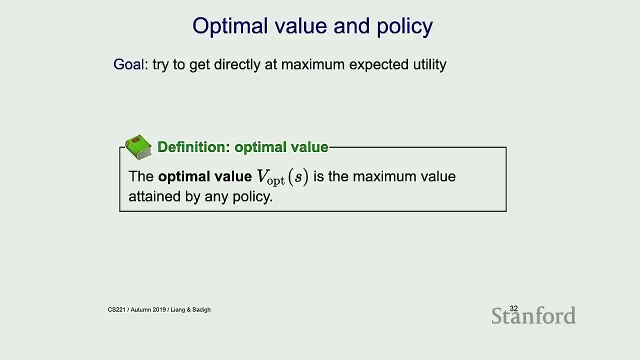 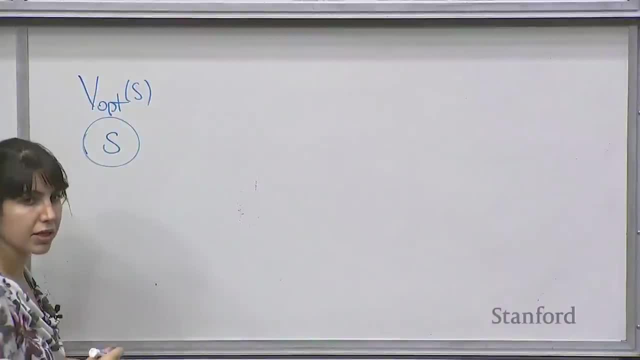 I wanna do value iteration- okay, So I'm gonna start from state S again. State S has V Opt of S. okay, So I'm gonna start from state S again- S. okay, that is what I'd like to find. 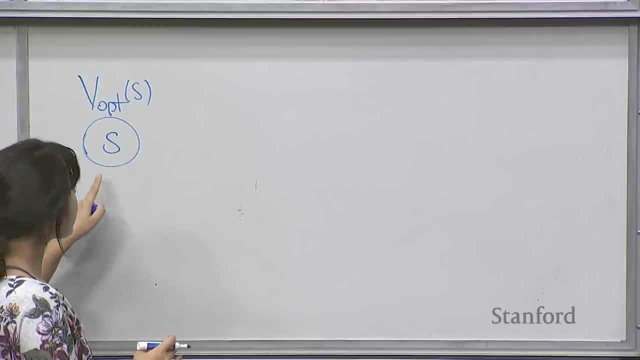 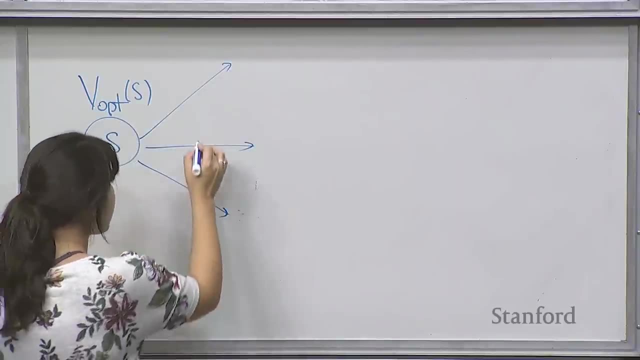 Here I had V Pi of S. If I'm looking for V Opt of S, then I can have multiple actions that can come out of here And I don't know which one to take. But like any of the- if I take any of them, 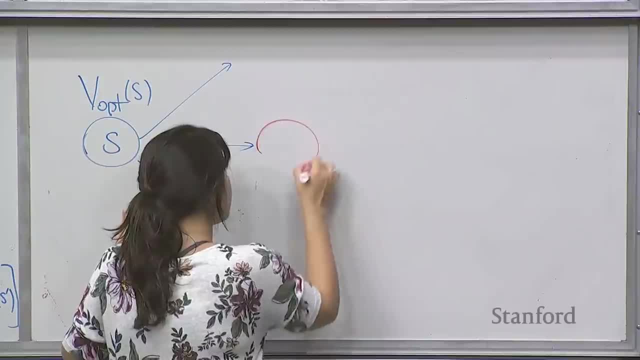 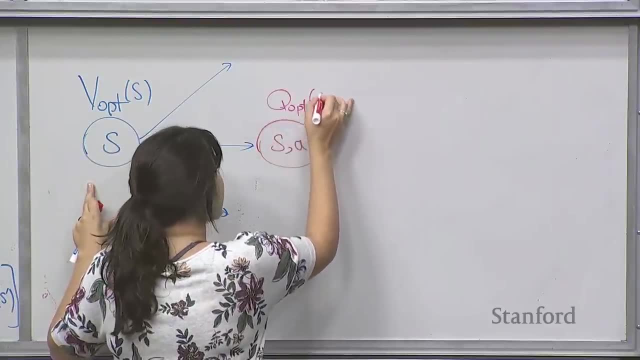 if I take this guy, that takes me to a chance node of S A. okay, And then I'm looking for qолоct of S A And from here it's actually pretty similar to what we had right here. So I'm in a chance node. 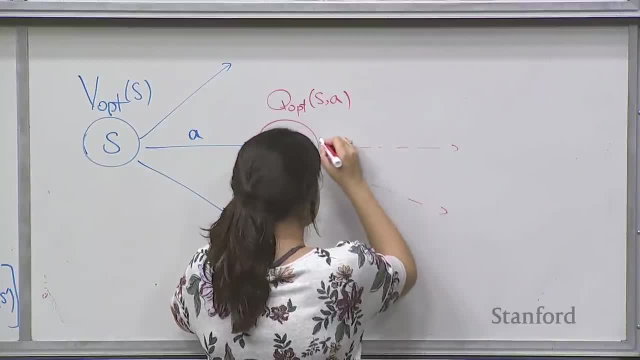 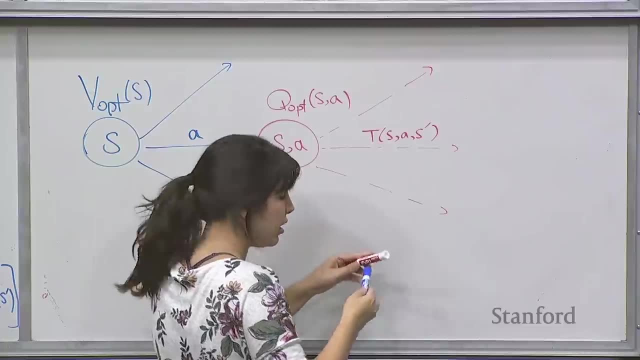 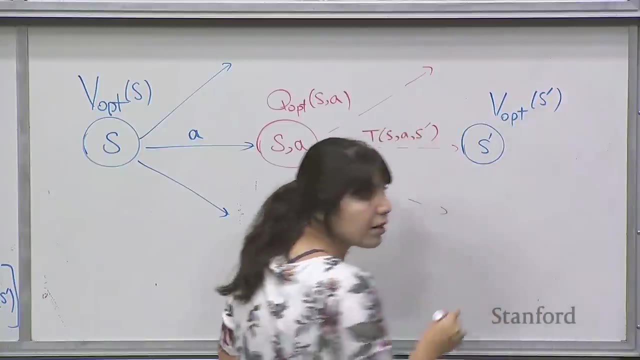 Anything can happen right. Nature plays and with some transition probability of S A S prime, I'm going to end up in some new state S prime And I care about V opt of that S prime. okay, So if I'm looking for this optimal policy, 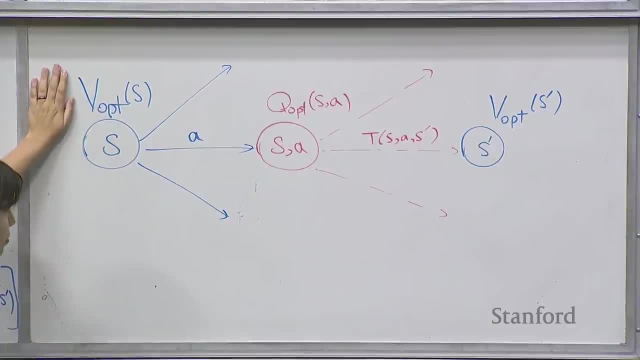 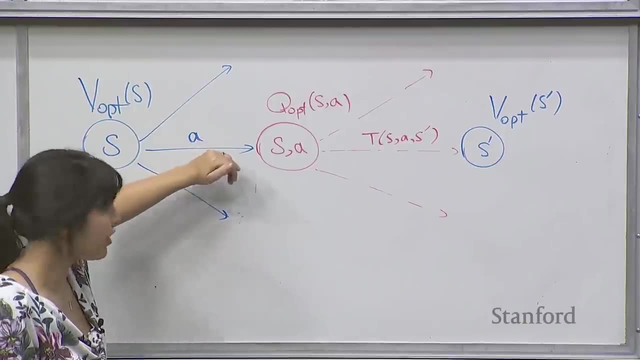 which comes from this optimal value, then I need to find V opt. And if I want to find V opt, well, that depends on what action I'm taking here. But let's say I take one of these, And if I take one of these, 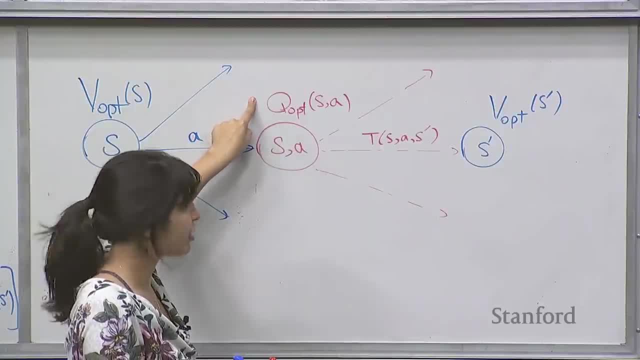 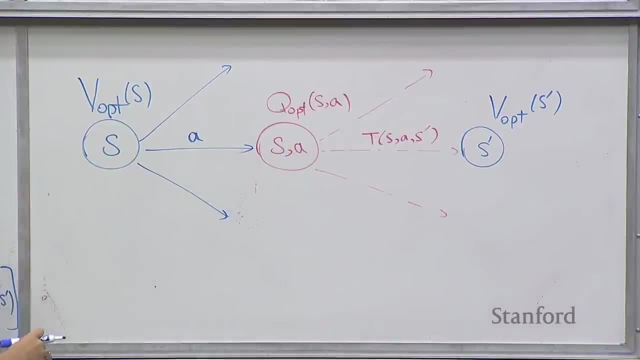 I end up in a chance node, I have Q opt of S A in that chance node And then from that point on, with whatever probabilities, I can end up in some S prime okay. So I want to write the recurrence for this guy. 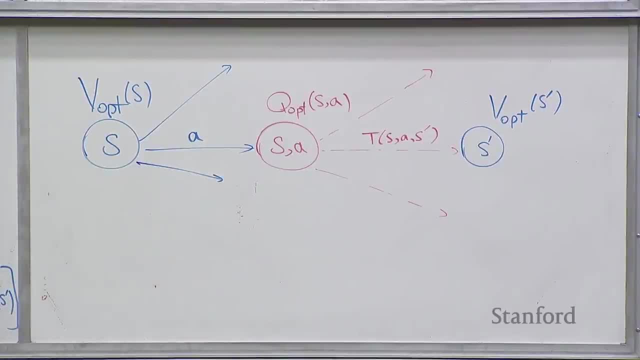 similar to the recurrence that we wrote here. It's gonna be actually very similar, So okay, so I'm going to start with Q, because that is easier. So what is Q? opt of S A That that just seems very similar to this previous case. 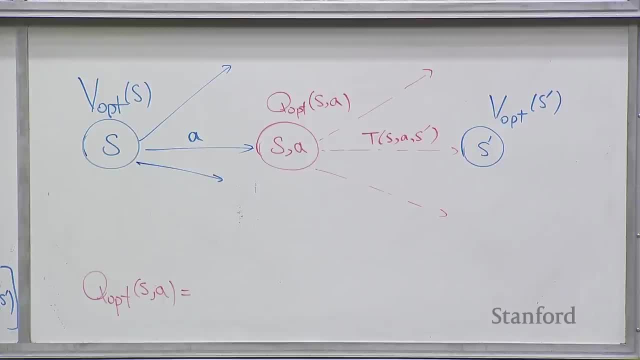 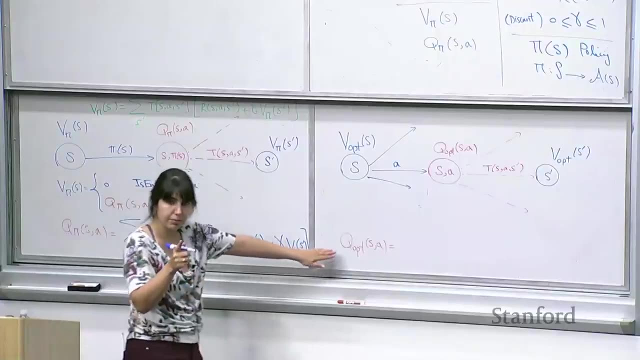 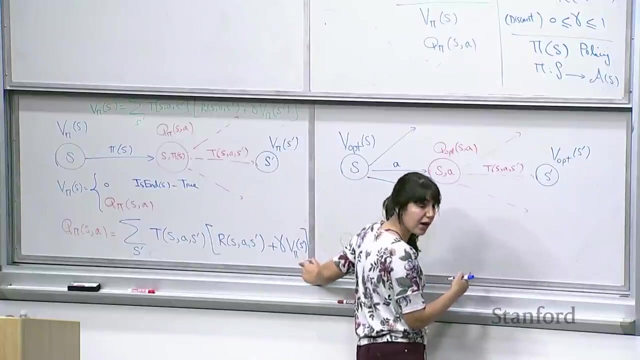 What is that equal to? What was Q pi? Q pi was just sum of transition probabilities, times, rewards, right? So so what is Q opt? Yeah, So so it would just be basically this equation, except for I'm gonna replace V pi with V opt. 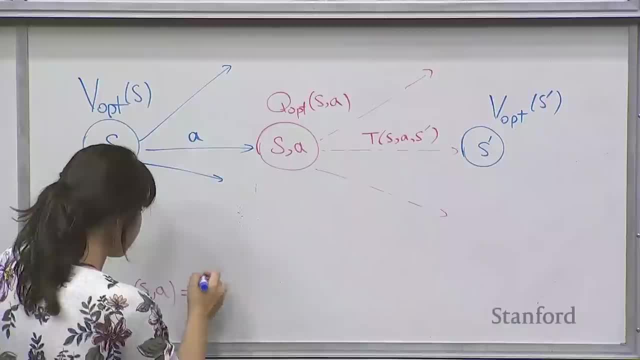 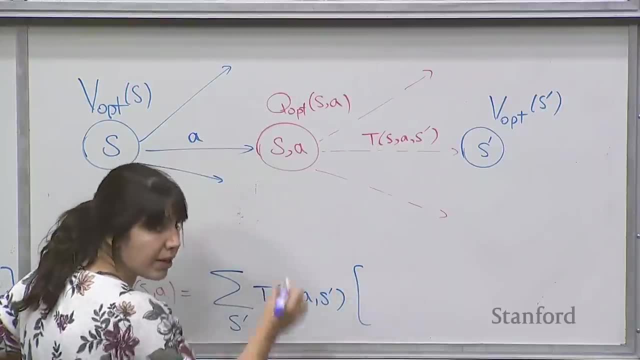 So so from Q opt I can end up anywhere like based on the transition probability. So I'm gonna sum up over S primes and all possible places that I can end up at. I'm gonna get an immediate reward, which is R S A S prime. 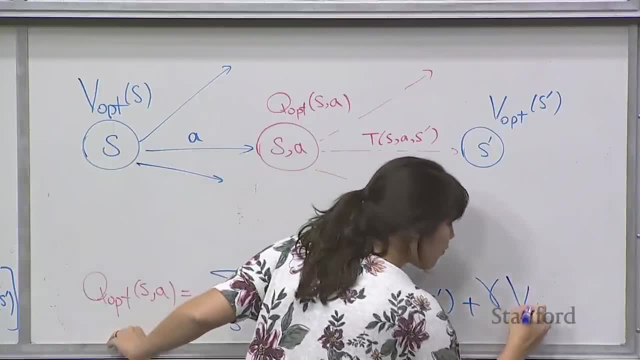 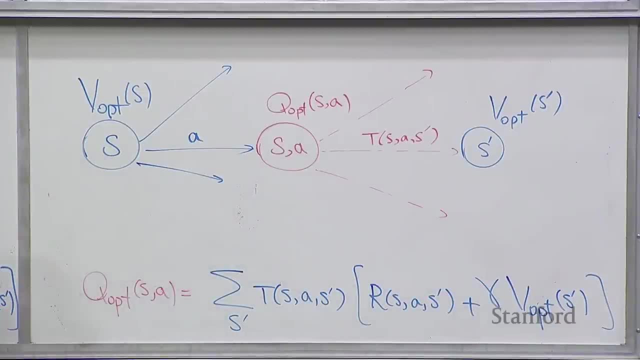 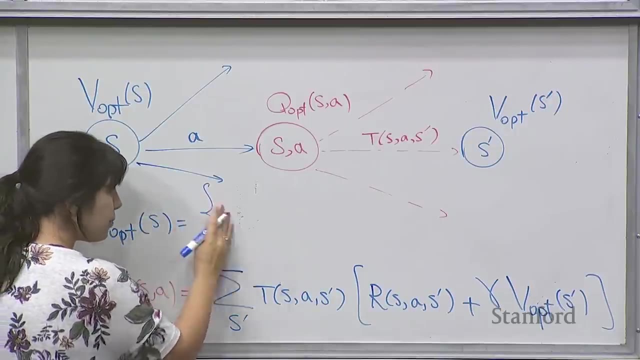 And I'm gonna discount the future. But the value of the future is V opt of S prime. okay, So so far, so good. that's Q opt. How about V opt? What is that equal to? Well, it's going to be equal to zero if you're in an n state. 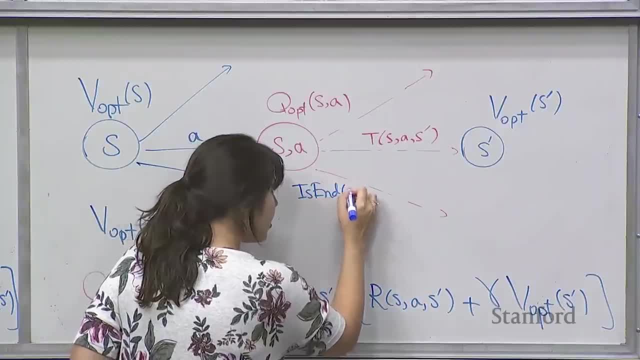 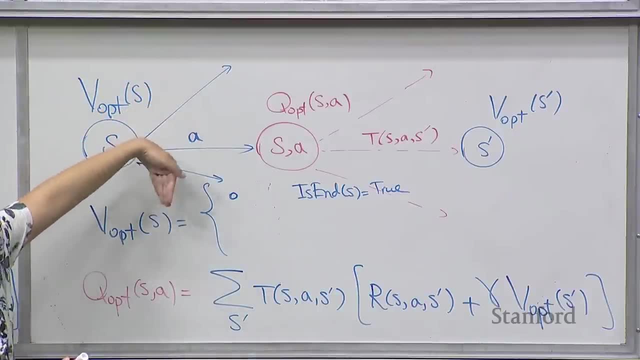 that's similar to before. So if this n of S is true, then then it is zero. Otherwise I have. I have a bunch of options here, right, I can take any of these actions and I can get any Q opt. 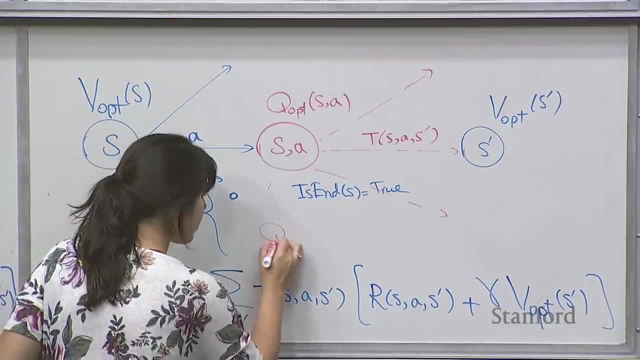 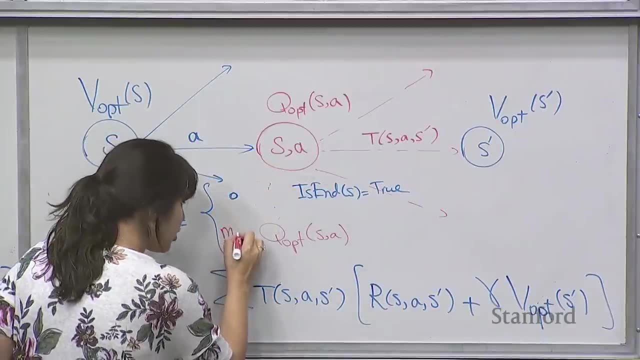 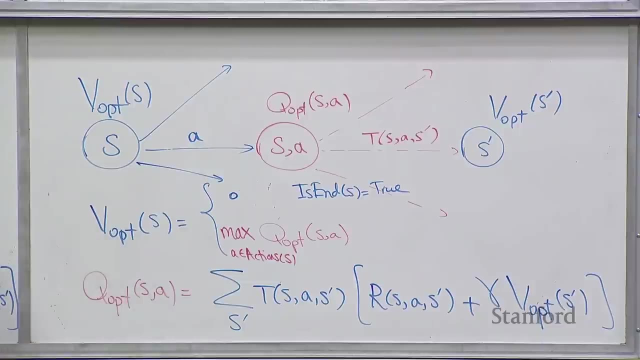 So which one should I pick? Which Q opt should I pick? The one that maximizes right, Like I'm? which action should I take? I should pick an action from the set of actions of that state that maximizes Q opt. 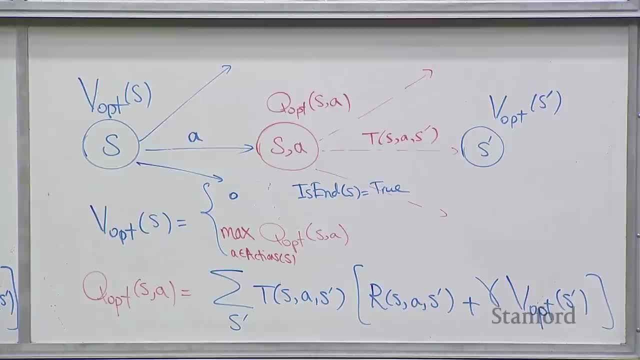 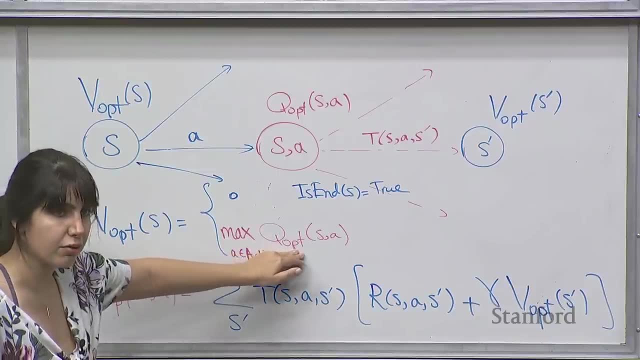 So so the only thing that has changed here is, before someone told me what the policy is, I just took the Q of that. Here I'm just picking the maximum value of Q And, and that actually tells me what action to pick. 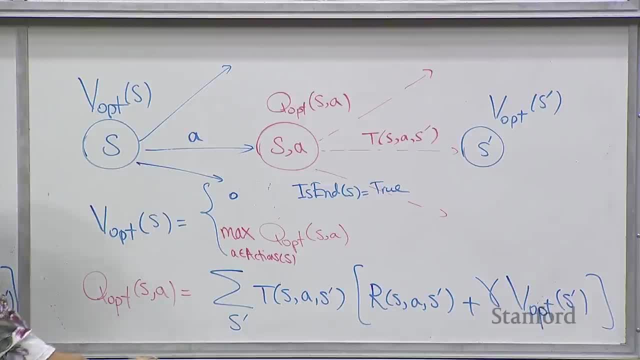 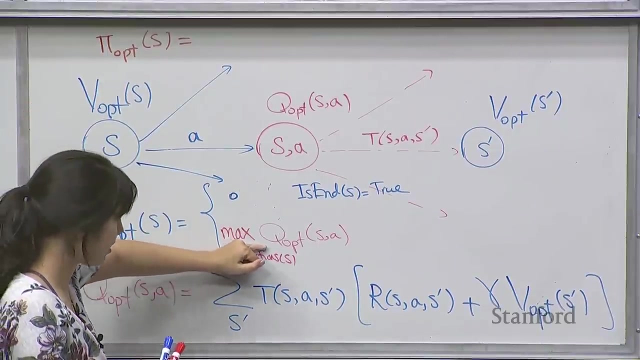 So what is the optimal policy? What should be the optimal policy? I'm gonna pa- call it pi, opt, Opt of S. What is that equal to? It's gotta be the thing that maximizes V, right, Which is the thing that maximizes this, this, this Q? 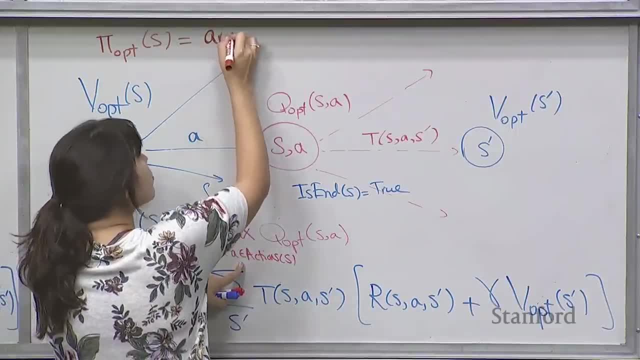 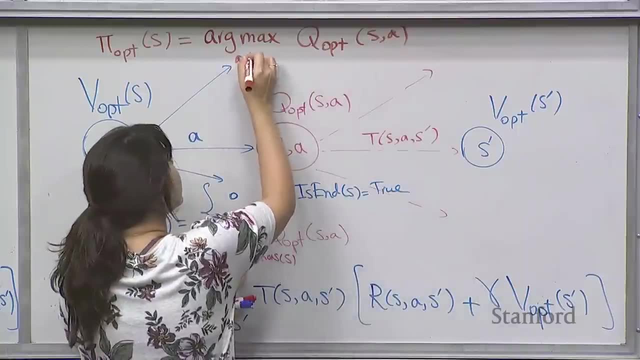 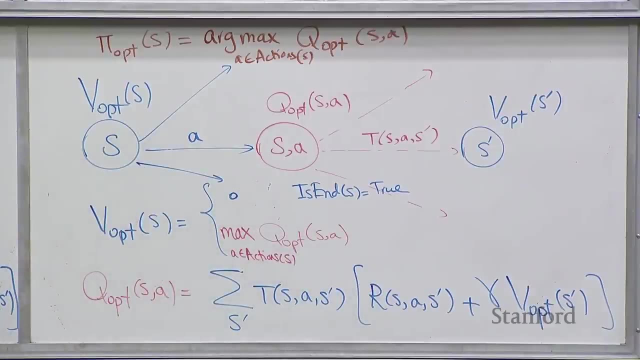 So, because that gives me the action, So it's going to be the argmax of Q opt of S and A, where A is in actions of S. Okay, All right. So this was policy evaluation. Someone gave me the policy. 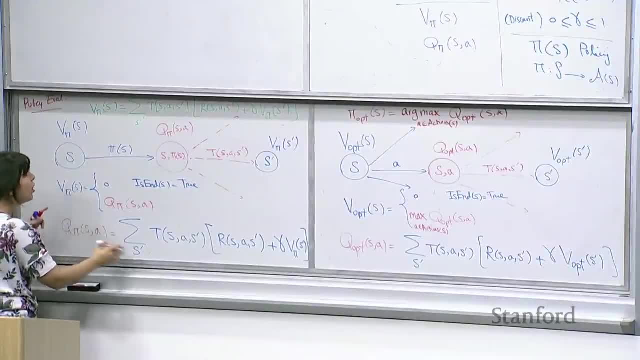 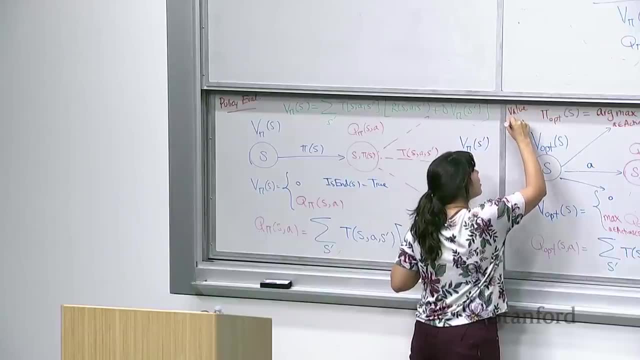 With that policy, I was able to compute V, I was able to compute Q, I was able to write this recurrence. Then I had an iterative algorithm to do things. This is called value iteration. This is to find the right policy iteration. 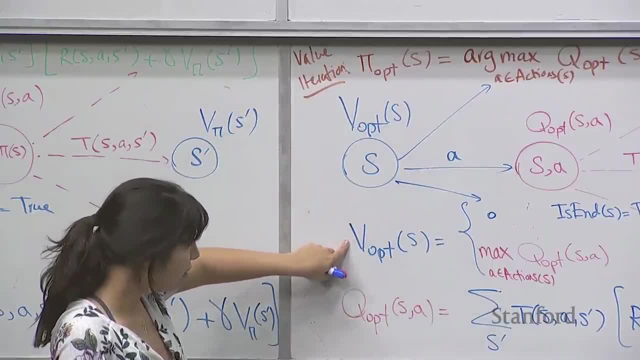 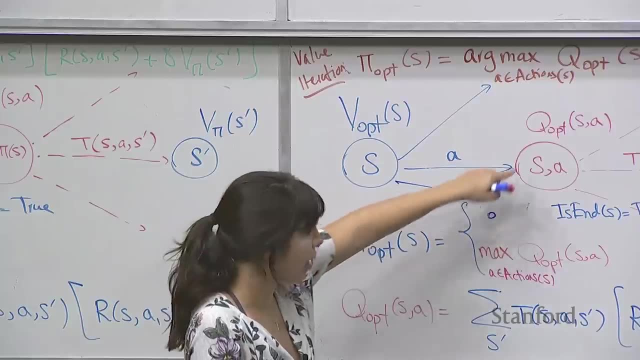 This is to find the policy. How do I do that? Well, I have a value that's for the optimal, optimal value that I can get, And it's going to be maximum over all possible actions I can take of the Q values. 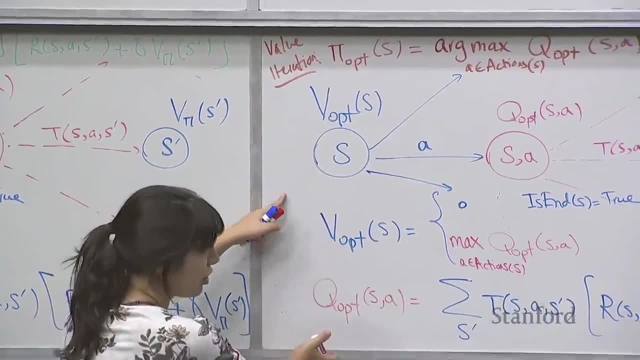 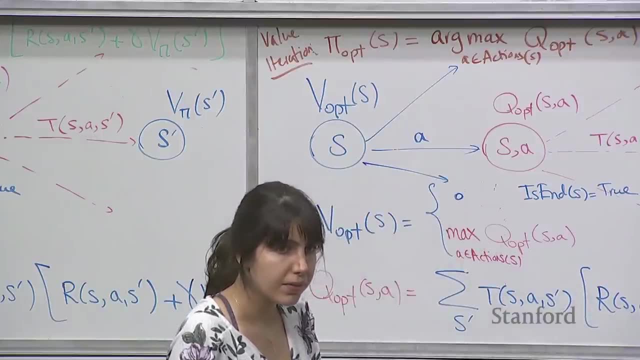 And Q values is similar to before, So I have this recurrence now, And then the optimal policy is just an argmax of Q. Oh yeah, So you could get two A's right. So the question is: yeah, like what if? 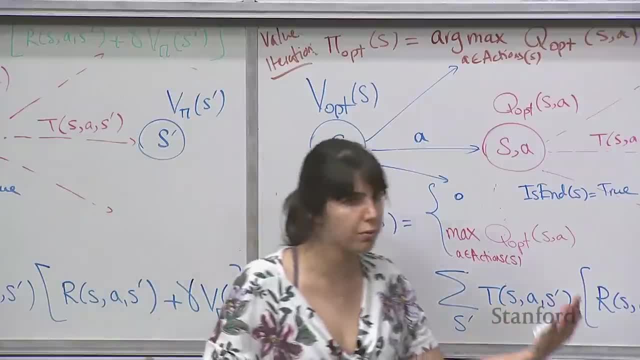 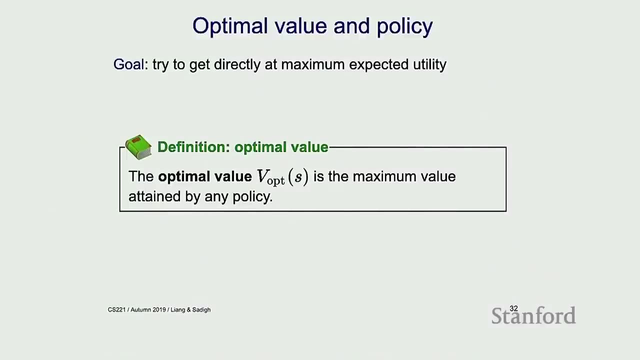 like I, I have two A's that give me the same thing. I can return any of them. It depends on your implementation of Max. So you can return any of them. How am I doing with this time? Ooh, we are five minutes over MDP1.. 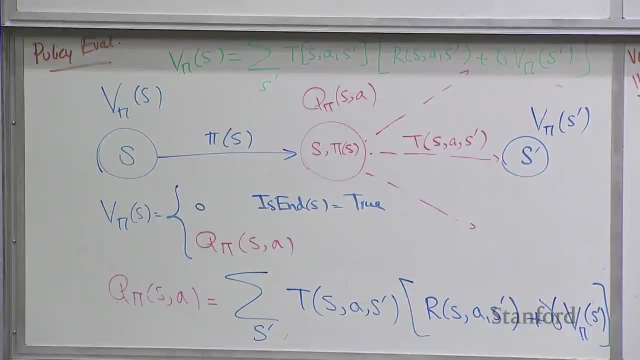 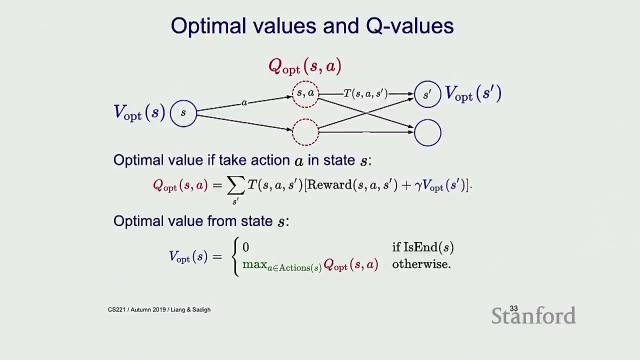 Okay, So uh, good news is, the slides are the same things that I have on the board, So so Qopt is just equal to the sum that we've talked about Vopt. I just add the max on top of Qopt. same story. 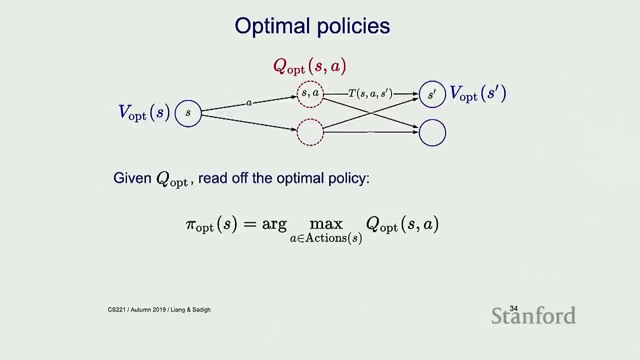 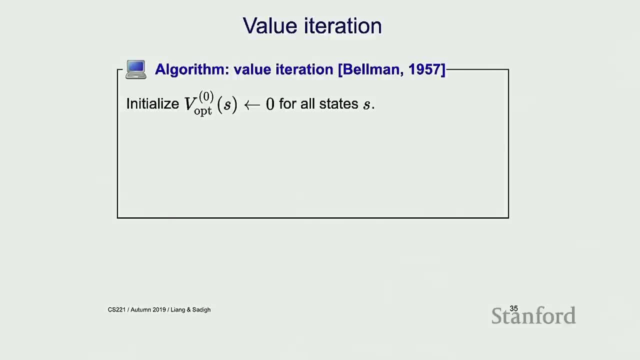 Okay, And then if I want the policy, then I just do the argmax of Qopt and that gives me the policy Right. I can have an again an iterative algorithm that does the same thing. It's actually quite similar to the iterative algorithm for policy evaluation. 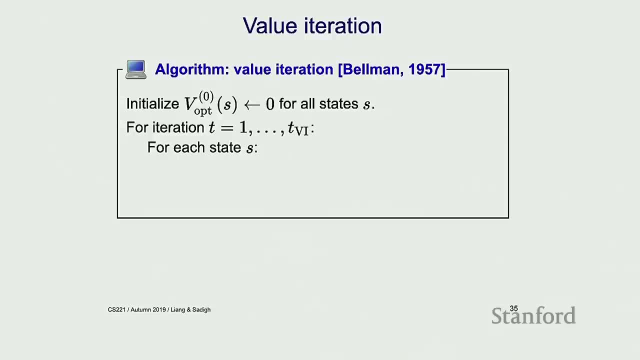 I just start setting everything to equal to zero. I iterate for some number of times, I go over all possible states And then I just update my value based on this new recurrence that has a max. Okay, So very similar to before. I just do this update. 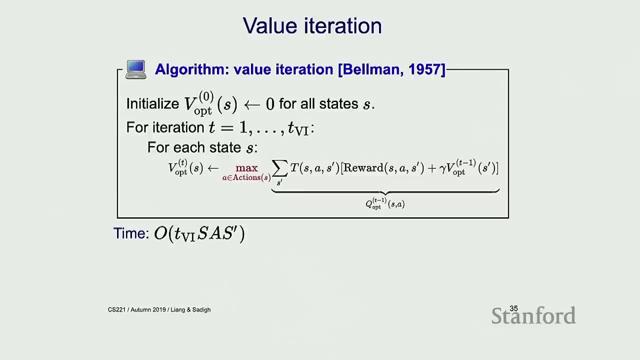 One thing is the time complexity is going to be order of T times S, times A times S prime, Because now I have this max value over all possible actions, So I'm actually iterating over all possible actions versus in policy evaluations I. I didn't have A because 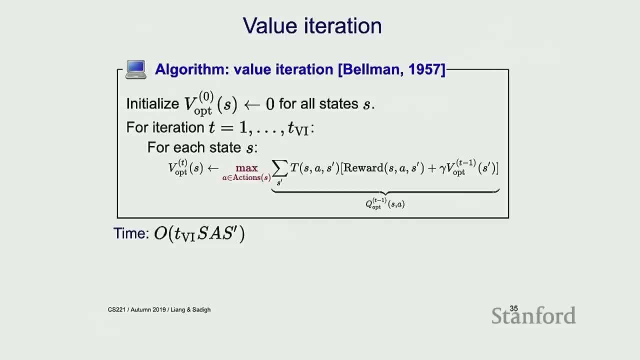 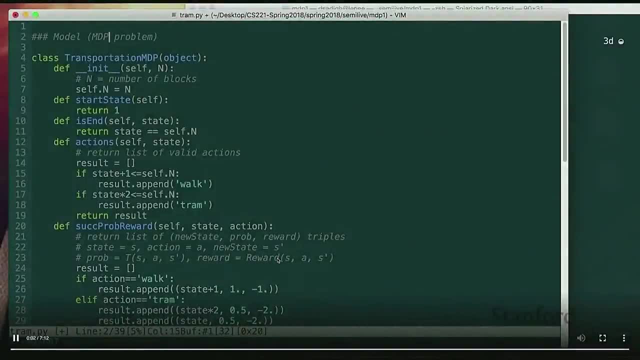 because someone would give me the policy. I didn't need to worry about this. All right, So. so let's look at coding this up real quick. Okay, So we have this MDP problem. We defined it. It was a tram problem. 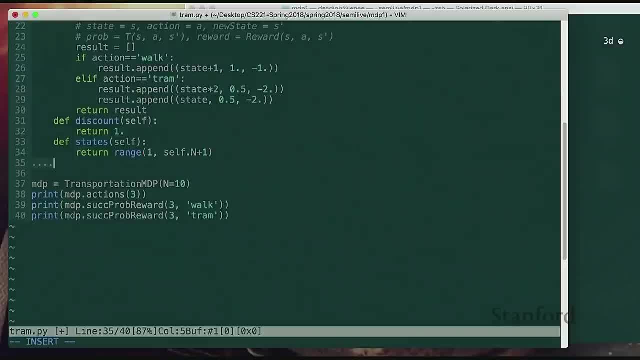 It was probabilistic, Everything about it was great. So now I just want to do an algorithm section, An inference section, where I code up value iteration And I can call up value iteration on on this MDP problem to get the best optimal policy. 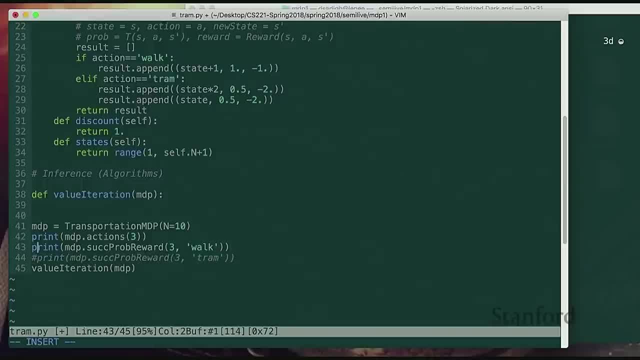 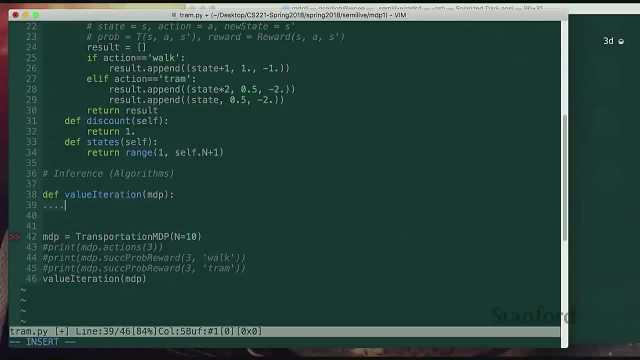 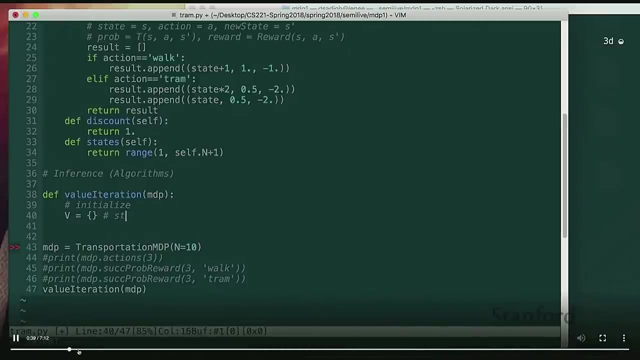 Okay, So I'm gonna call value iteration later. All right, So we initialize. So all the values are going to become. I might skip things to make this faster. So, uh, we're gonna initialize all the values to just 0, right. 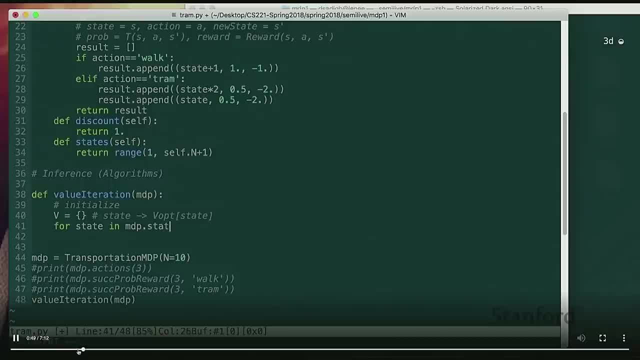 Because all these values are gonna be 0. So I defined a states function. So I, for all of those, the value is just going to be equal to 0. So let's initialize with that. Then you're just gonna iterate for some number of time. 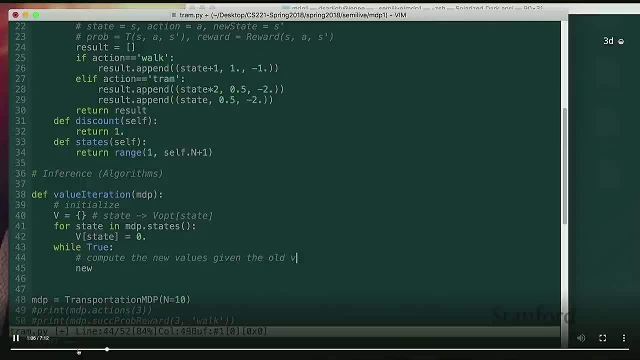 And what we wanna do is: you wanna compute this new value given old values. So it's an iterative algorithm. We have old values, We just update New values, New values based on them. So what should that be equal to? Okay, So we iterate over our states. 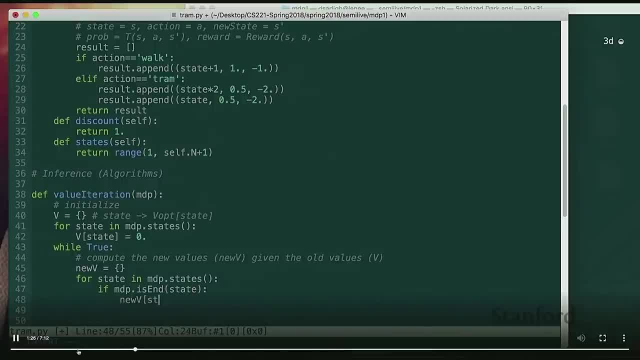 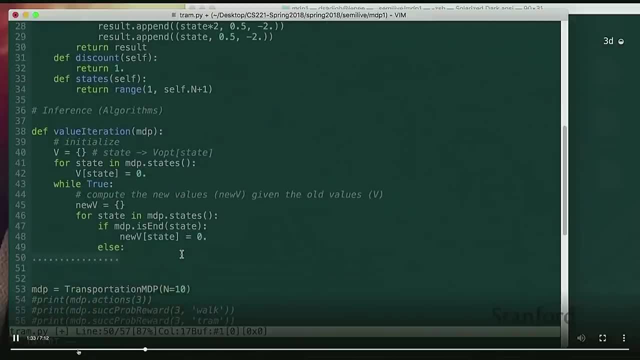 If you are in an end state, then what is value equal to 0, right? If you're not in an end state, then you're just gonna do that- iter- that that uh recurrence there. Okay, So new value of a state is going to be equal to max of what? 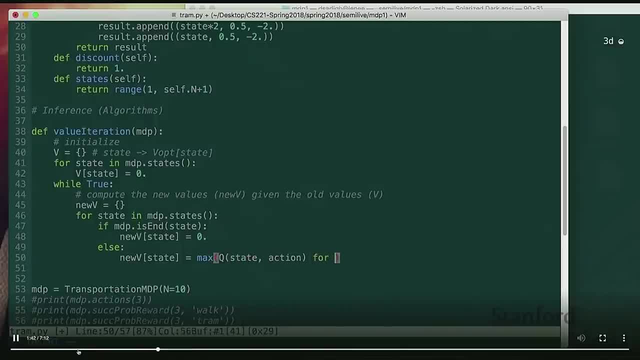 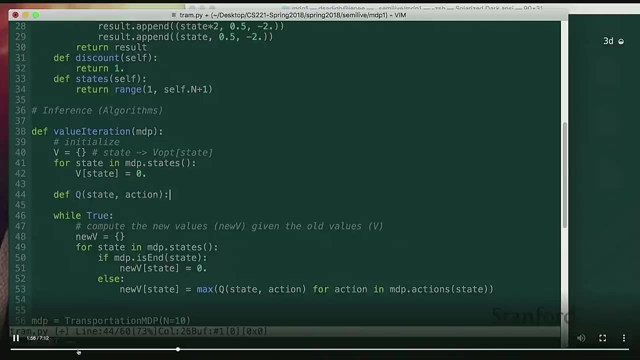 The Q values. Okay, So new V is just max of Qs of state and actions. Okay, So now I need to define Q. Well, what does Q do? Q of state and action is just equal to that sum over over S primes. 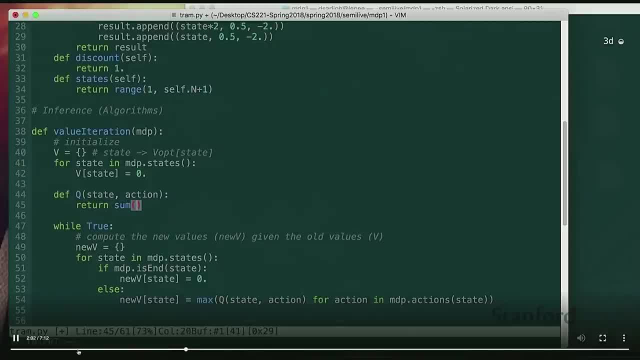 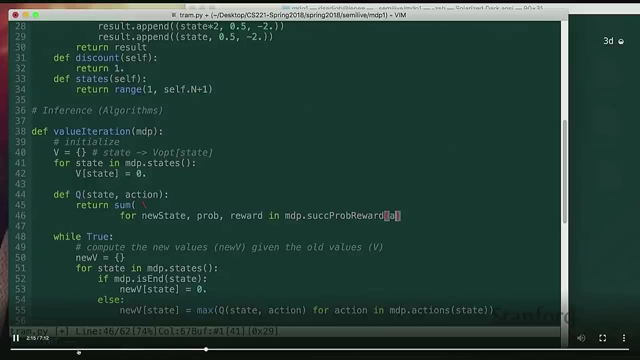 So it's gonna return sum and it's gonna return sum over S primes. I define this successor probability and reward function that gives me new state probability and reward. So I'm I'm gonna iterate over that and and call that up, uh, here. 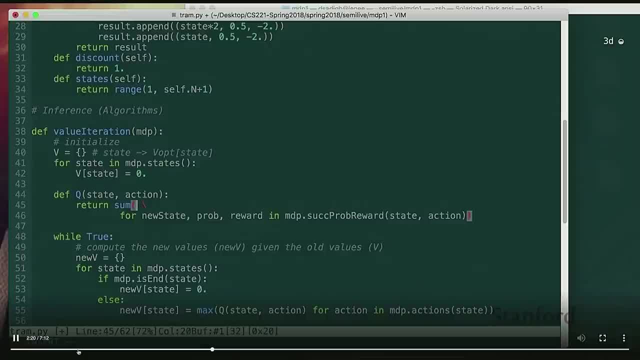 So, given that I have a state and action, I can get new state, probability and reward. What are we summing? We are summing the probability, the transition probabilities, times the immediate reward, which is reward here, times my- plus my discount. 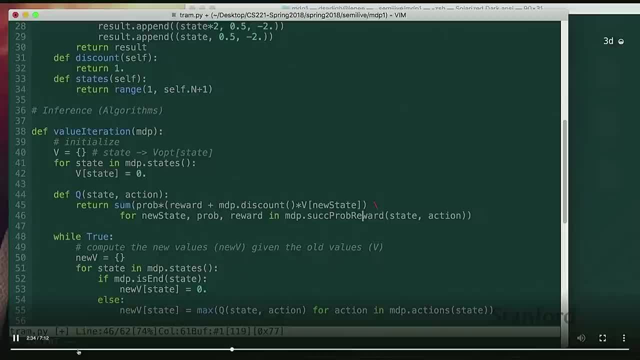 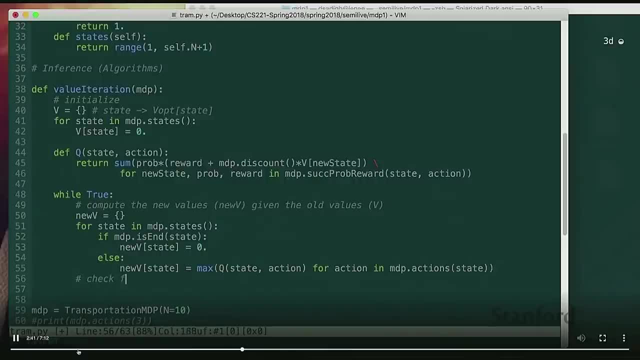 times my V, which is the old value of V over S prime, over my new state. So that is my Q, that is my V and that's pretty pretty much done. We just need to check for convergence, To check for convergence. 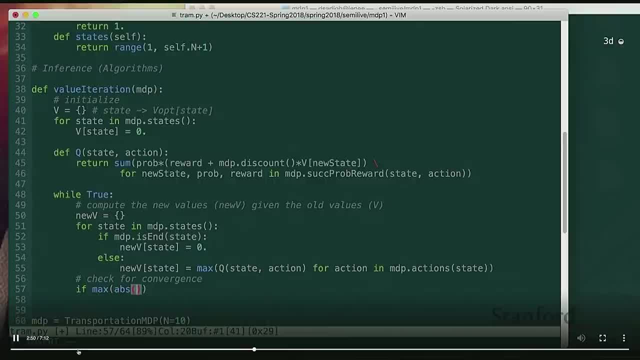 we kind of do the same thing as before. We check if value of V and new V are close enough to to each other that we can call it done. I'm gonna skip these parts, So so you can basically check if V minus. 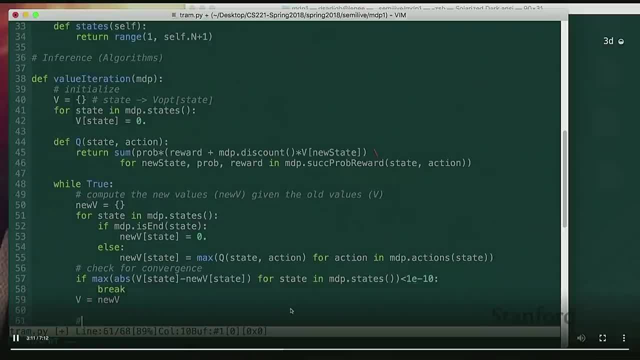 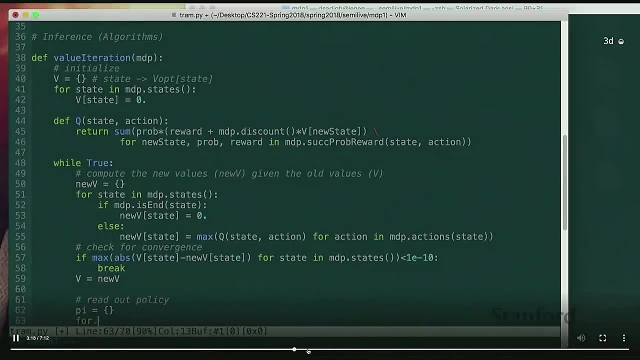 uh, new V are within some threshold for for all states, And if they are, then um V is equal to new V. We need to read the policy. So policy is just argmax of Q, So, um, I'm gonna make this a little bit faster. 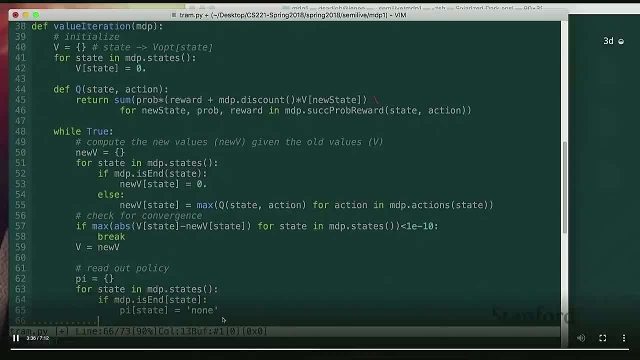 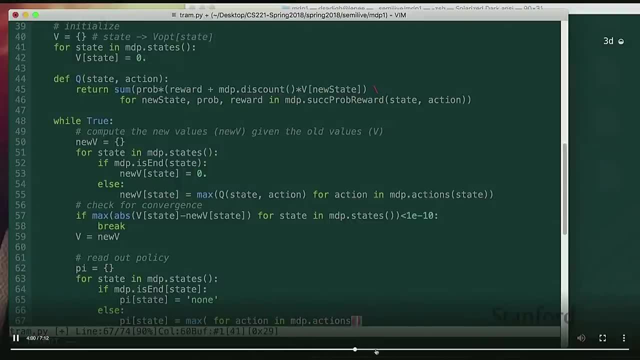 So the policy is just going to be well, none if you are in an end state and otherwise it's just going to be argmax, um of of our Q values. So I'm just writing argmax here, pretty much. 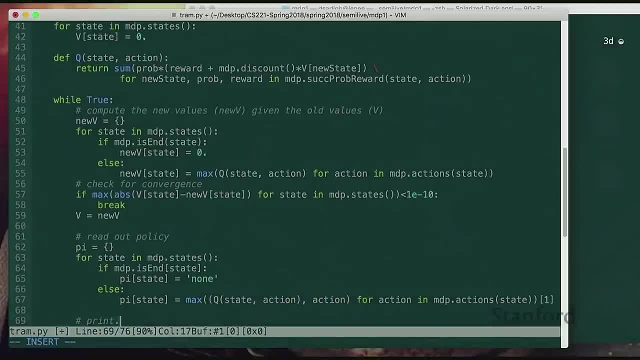 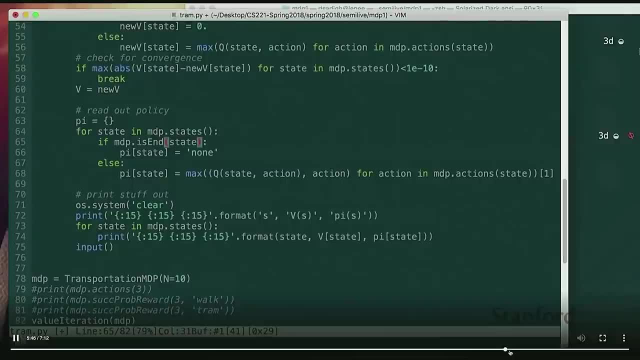 I'm just returning the action that maximizes the Q, And then we need to spend a bunch of time getting the printing working, So let me actually get yeah, okay, All right, Actually, right here. So I'm running this function. 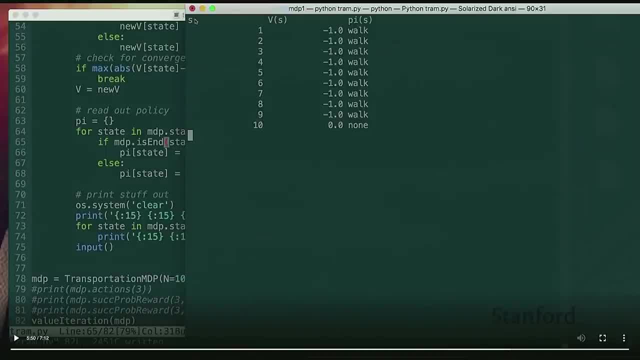 I'm re- I'm writing out- actually these are a little shifted here: states, values and then pi, which is the policy. Okay, So it starts off: walk, walk, walk. Remember this is the case where we have 50% probability of tram failing. 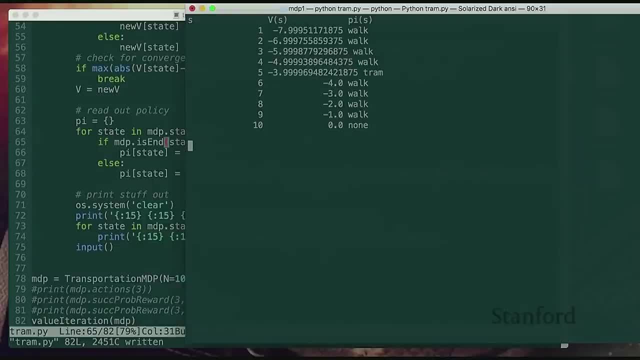 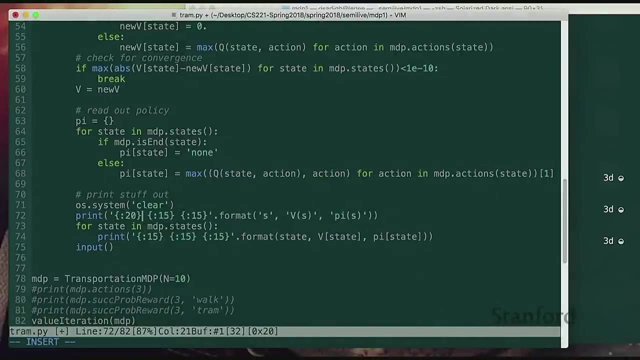 And with 50% probability of tram failing. these are the values we are gonna get, And the policy is still: walk until state five and then take the tram from from state five. Okay, Which is kind of interesting, because the policy of the search problem was the same thing too. 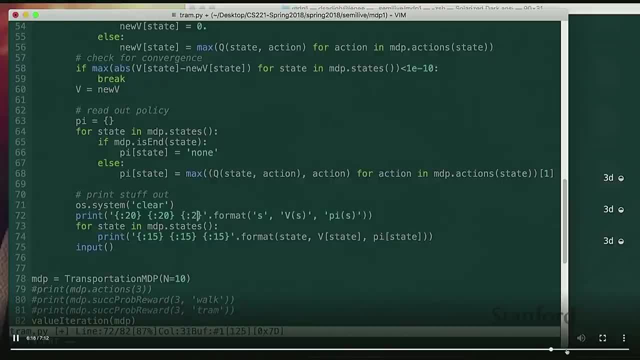 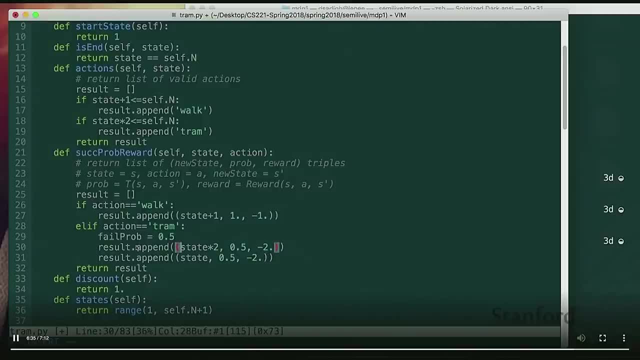 Okay, So the thing we can do is: um, we can actually- let me move this a little bit forward- We can actually define this fail probability, which um becomes just a variable. So you can play around with this If you pick different fail probabilities. 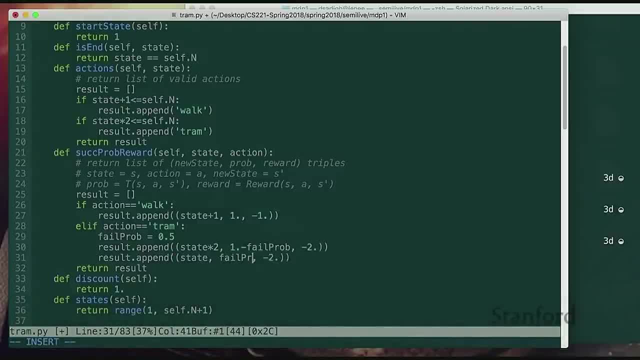 you're gonna get different policies. So, for example, if you pick a fail probability that is large, then probably like the policy is going to be: just just walk and never take the tram, because the tram is failing all the time. 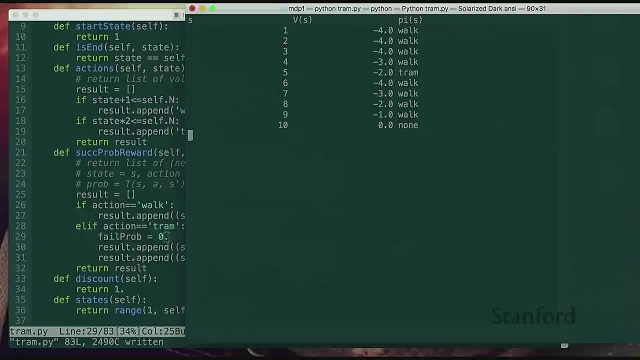 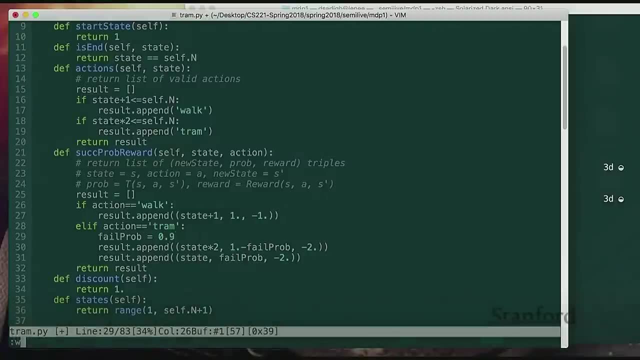 But if, if you decide to take a fail probability that's close to zero, then then this is your optimal policy, which is close to the search problem. So it's basically the solution to the search problem. So play around with this. 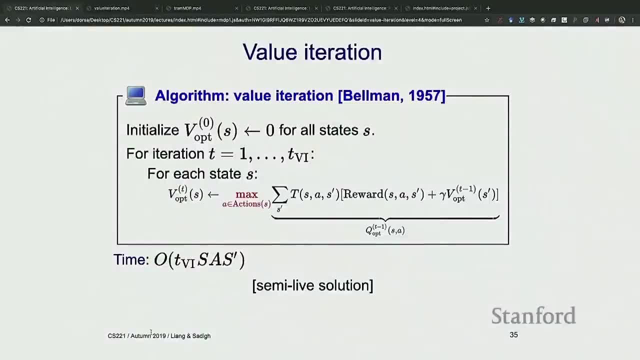 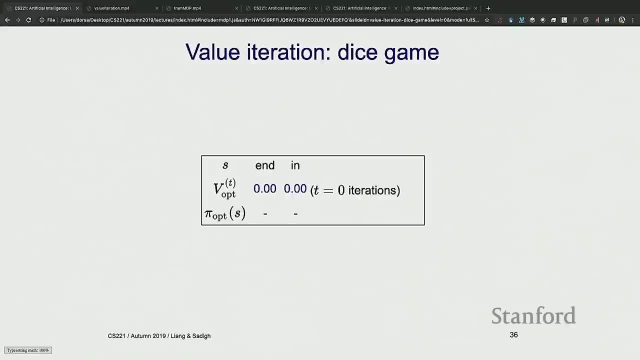 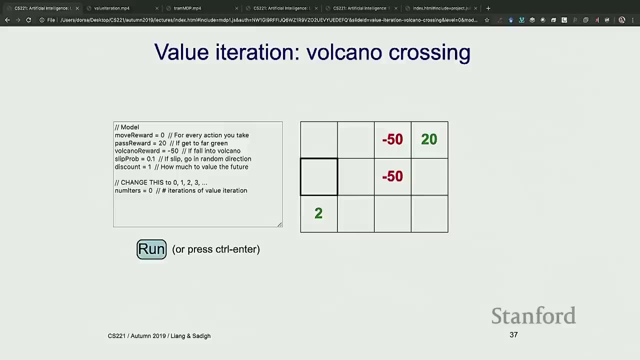 The code is online. This was just value iteration, um value iteration And um use it on this tram problem. Okay, So I'm gonna skip this one too, All right, So, um, yeah, And, and this is also uh. 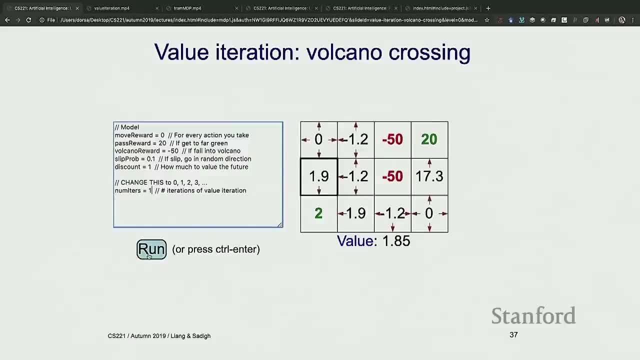 showing like how, over multiple iterations, you can kind of get to the get to the optimal, optimal value and optimal policy using value iteration, So with one iterations. it hasn't seen it yet, So it thinks that the value, the optimal value, is 1.85.. 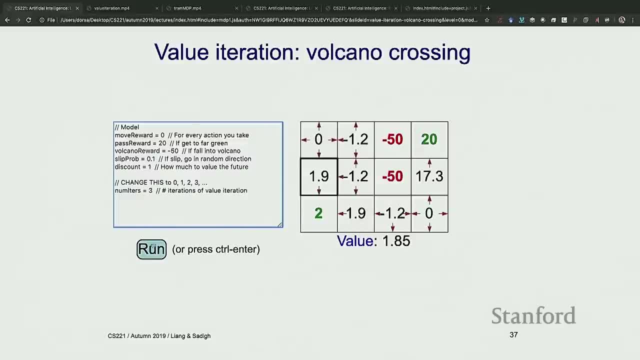 It hasn't updated the values. Uh, so like, with I don't know three iterations it gets better, but it hasn't still updated it. It still thinks it can't get to the other side. And remember, this is with the probability of 10 percent. 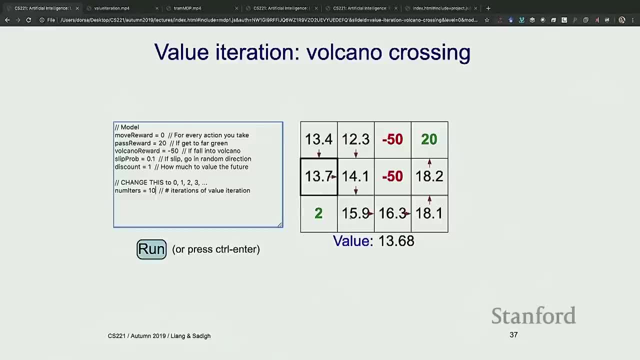 Uh, but if I get to like, I think, 10,, then it eventually learns. the best policy is to get to 20, and the value is 13.68.. And if you go even like higher iterations after that point it's just fine-tuning. 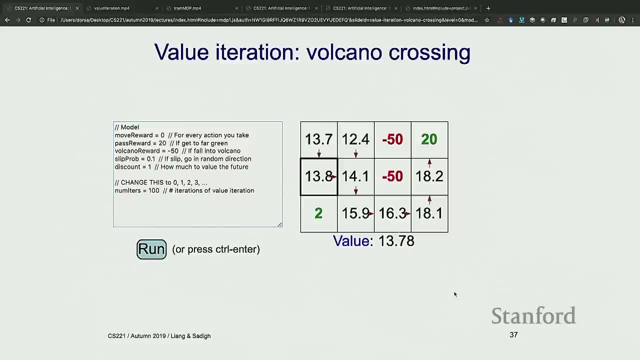 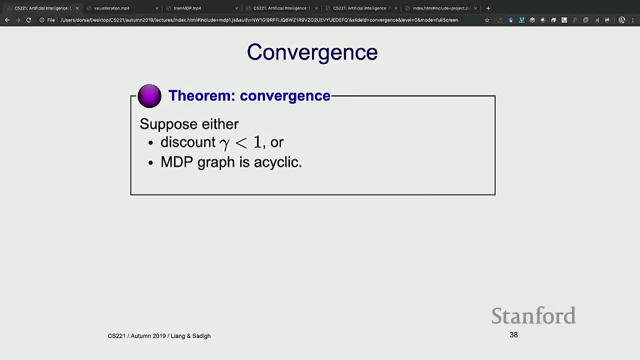 So the values are around 13, still, Okay, So you can play around with the volcano problem, Okay. So when does this converge? So, um, if the discount factor is less than one or your MDP graph is acyclic, 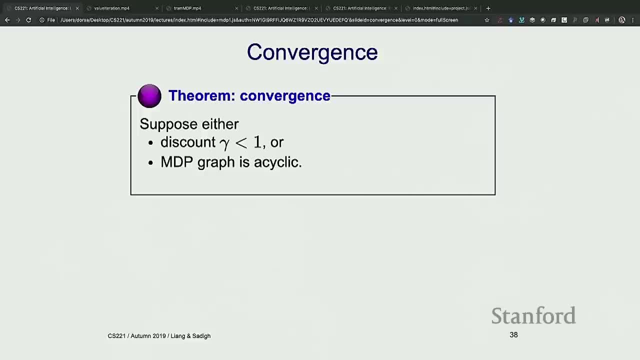 then this is going to converge. So if MDP graph is acyclic, that's kind of obvious. You're just doing dynamic programming over your full thing, so- so that's going to. that's going to converge If you have cycles, 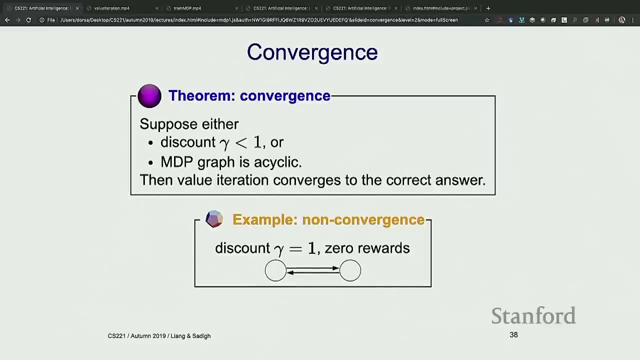 you will want your, your discount to be less than 1.. Cause if you- if you have cycles and your discount is, let's say, 1, and let's say you're getting zero rewards from uh, then you're never going to change. 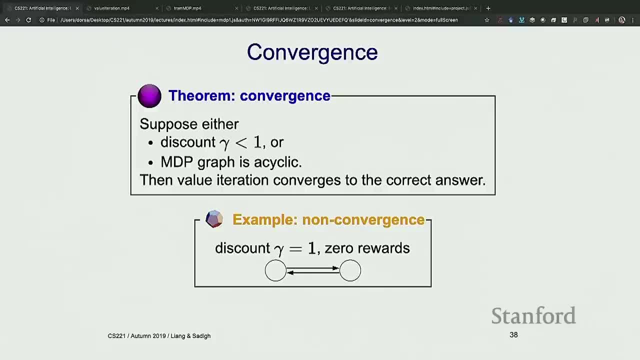 you're never going to move, move from your state. You're always going to be stuck in your state And if you have non-zero rewards, you're going to get this unbounded reward and keep going, because you have cycles and and it's just going to end up becoming numerically difficult. 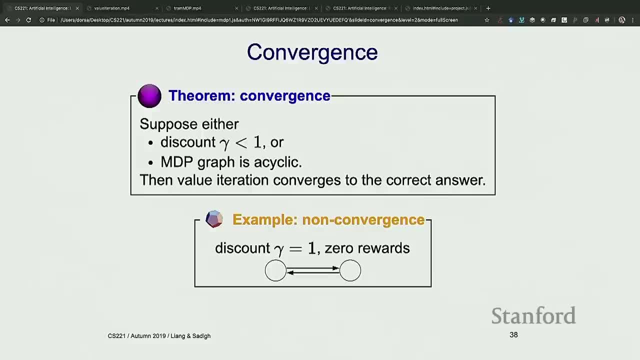 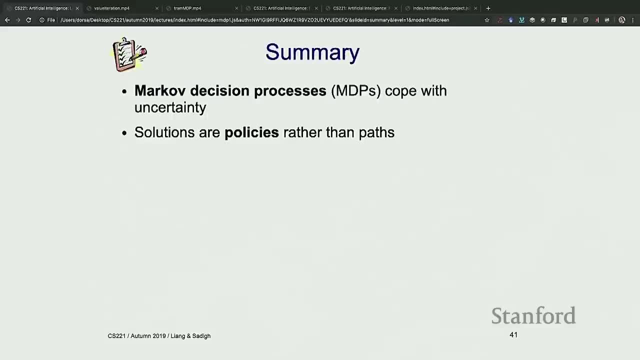 So so just a good rule of thumb is: pick a Gamma that's less than one then. then you kind of get this convergence property. Okay, All right, So yeah. summary: so far is we have MDPs Now. we've talked about finding policies rather than path. 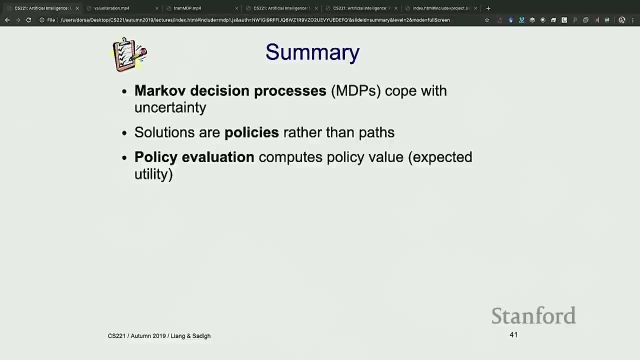 Policy evaluation is just a way of computing like how good a policy is, And the reason I talked about policy evaluation is there's this other algorithm called policy iteration which uses policy evaluation, And we didn't discuss that in the class, But it's kind of like a not equivalent. 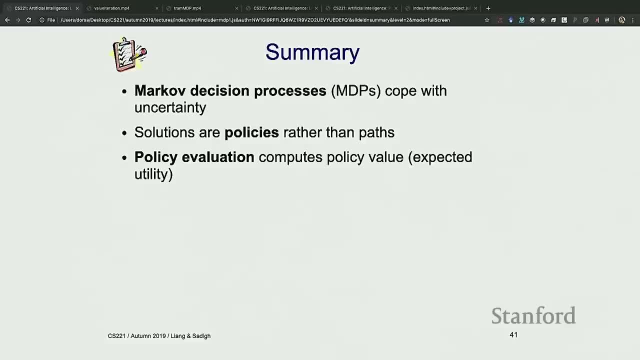 but you could use it in a similar manner as value iteration. It has its pros and cons. So policy evaluation is used in those settings. Do not leave, please. We have more stuff to cover. And then, uh, we have value iteration. 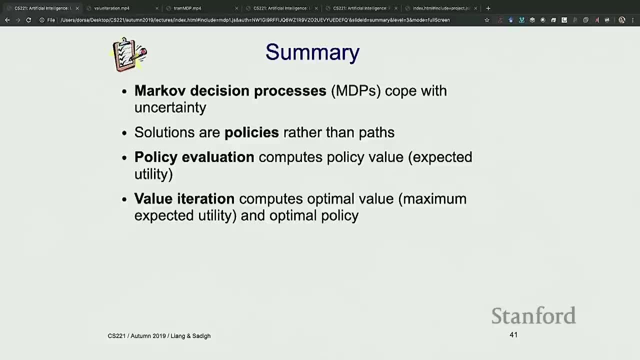 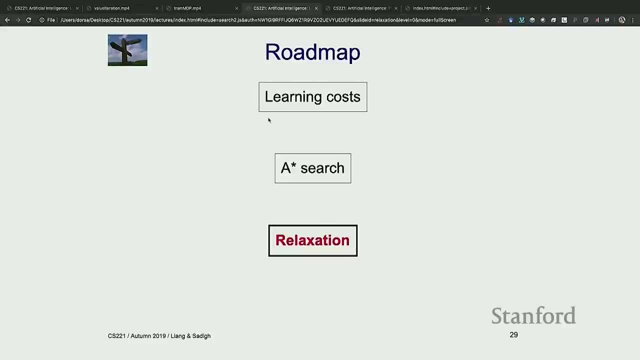 uh, which uh computes this optimal value, which is the maximum expected utility. Okay, And next time we are going to talk about reinforcement learning, and that's gonna be awesome, So we'll talk about unknown rewards. All right, So that was MDPs doing inference and 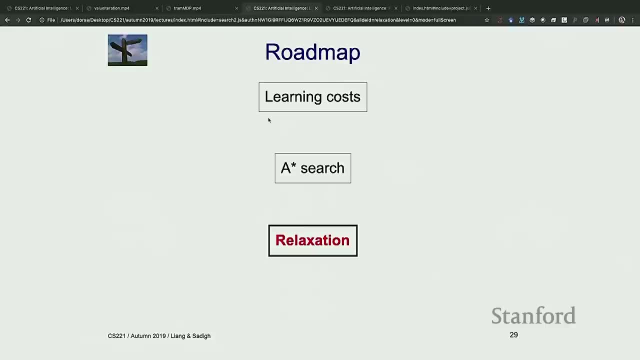 and, uh, kind of defining them. I'm going back to the last lecture just to kind of talk about some of the stuff that we didn't cover Last time. Okay, All right. So if you remember, last time we were talking about search problems. 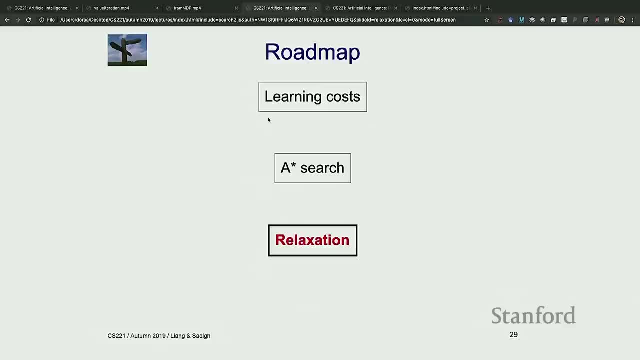 So a big switch now: search problems where, uh, we don't have probabilities, And we talked about A star as a way of just making things faster, And we talked about this idea of relaxations, which was, uh, a way of finding good heuristics. 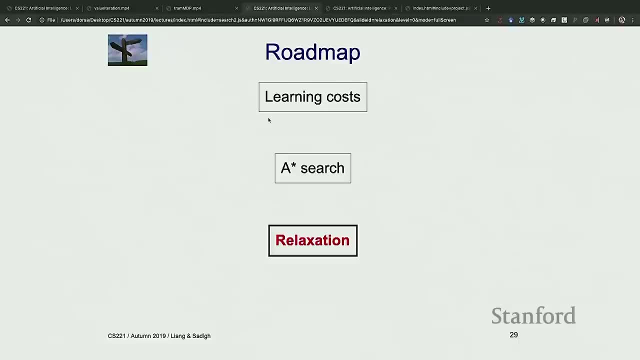 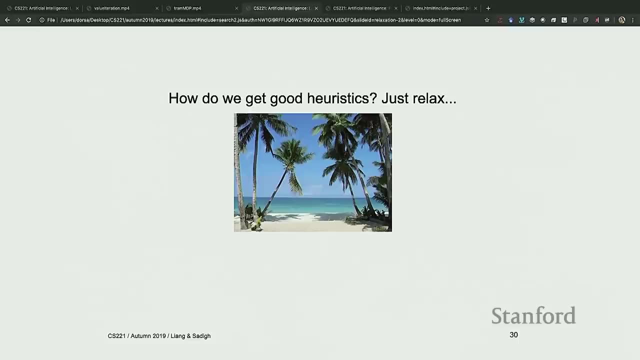 So A star had this heuristic. Heuristic was an estimate of future cost. We wanted to figure out how to find these heuristics, Like how do we go about finding this heuristic? And one idea was just to relax everything that allows you to come up with. 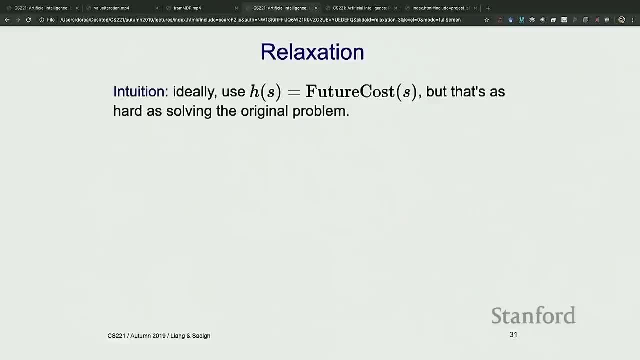 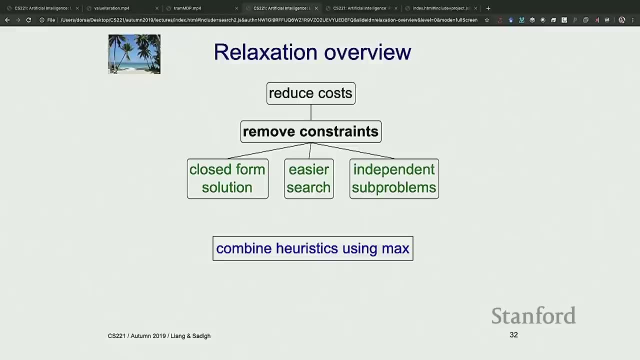 an easier search problem, or just easier problem, And that helps you to find what the heuristic is. Okay, So, um, so we talked about this idea of removing constraints, And when you remove constraints, then you can end up in nice situations. 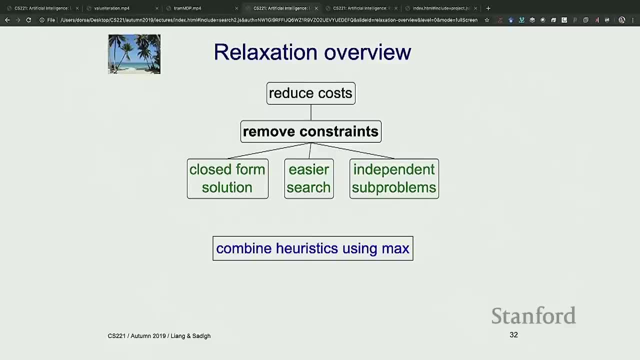 Like in some settings you have a closed-form solution. In some other settings you have just an easier search problem and you can solve that, And in some other settings you have like independent solve problems. So when you remove constraints then then you have this easier problem. 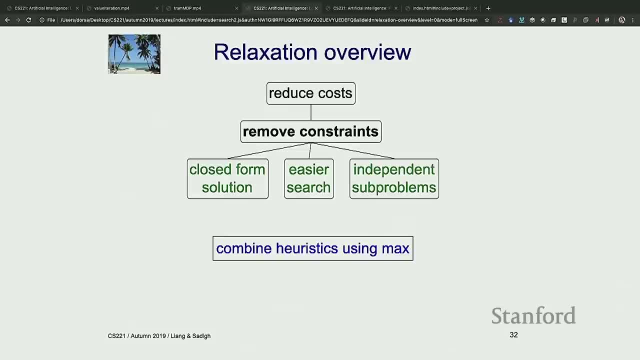 You can solve that easier problem and that gives you a heuristic. You're not done yet, right You're- you have a heuristic. you take that heuristic and then change your costs and and just run uniform cost. search on your original problem. 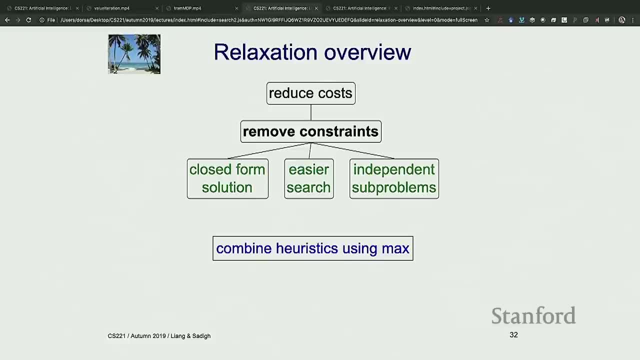 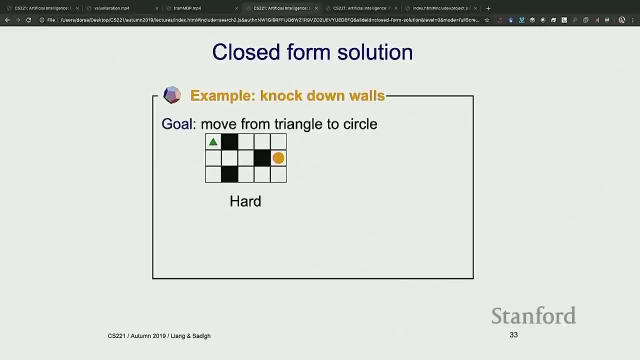 So so solving an easier problem is like you're not done. when you solve the easier problem, It just helps you to find a thing that helps for the original problem, So it's kind of like a multi-step thing. So examples of that is if you have walls. 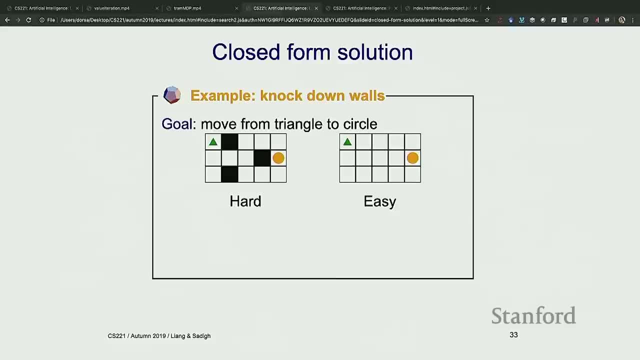 remove all the walls, you have an easier problem. If you solve that easier problem, that gives you a heuristic And in this case, like when you knock down these walls, that easier problem, you have a closed-form solution for it. You don't need to do anything fancy. 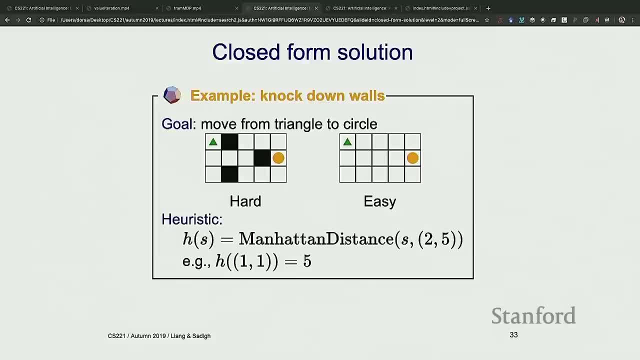 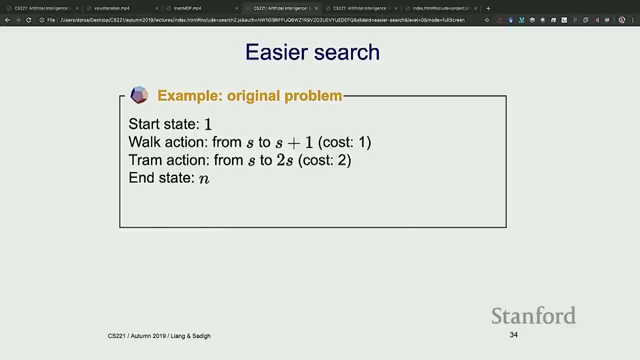 You don't need to do uniform cost search, any of that. You just compute the Manhattan distance and and that gives you a heuristic. With that heuristic you go and solve your original problem. That was one example. Another example is when you remove constraints. 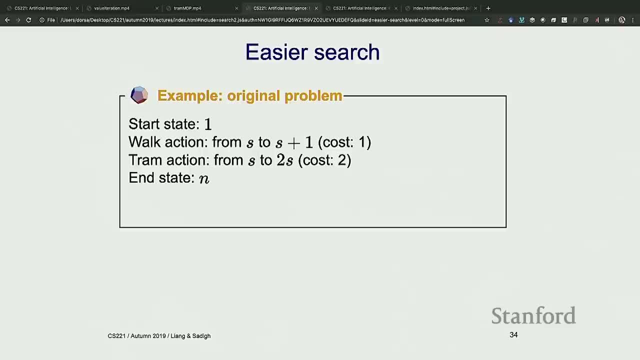 you have an easier search problem So you don't have closed-form solutions. but you have an easier search problem, So you might have a really difficult search problem with a bunch of constraints that are hard to do: Remove the constraints. So when you remove the constraints, 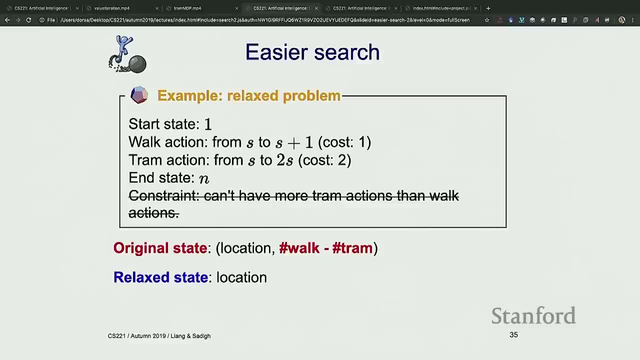 you have a relaxed problem which is just the original problem, without the constraint. That's a search problem. You can solve that search problem using uniform cost search or dynamic programming And and solving that allows you to find the heuristic. Again, you're not done yet, right. 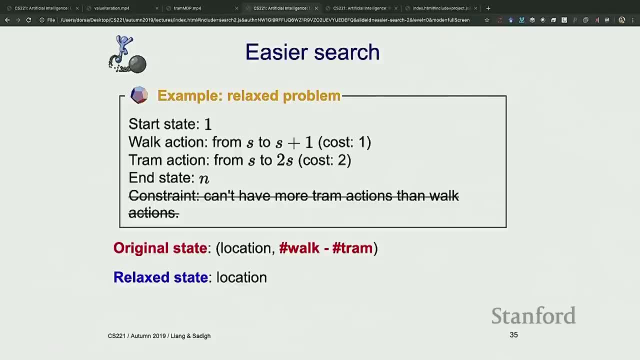 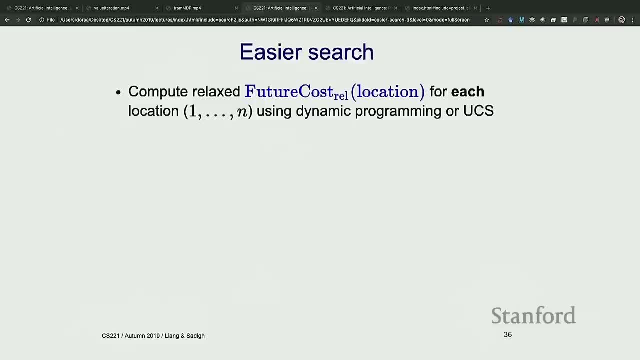 You take the heuristic and then you go to the original problem, change the cost and and run uniform cost search, And just one quick kind of example here was: uh, when you're computing these relaxed problems, the thing you wanna find is the future costs of this. 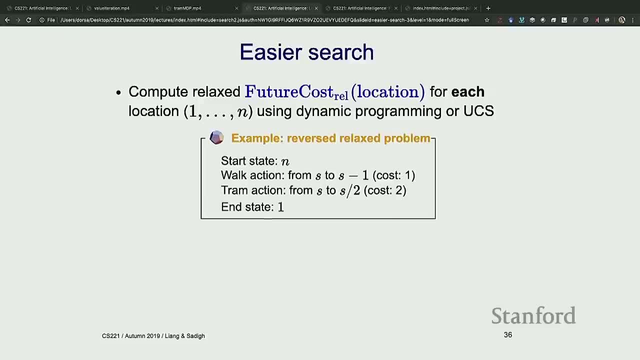 this relaxed problem And- and to do that you have this easier search problem- you still need to run uniform cost search or dynamic programming In this case. if you decide to run uniform cost search, remember uniform cost search computes past costs. 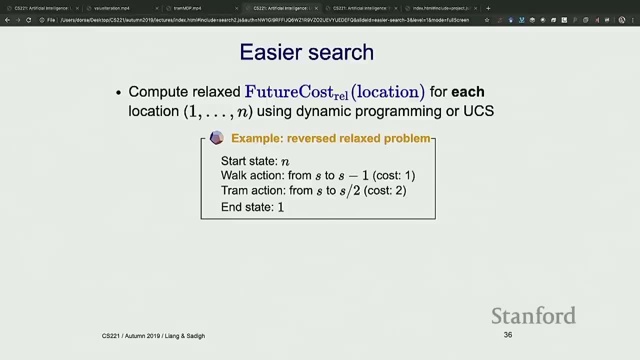 In this case, I really wanna compute future costs. Uh, so you need to do a bunch of engineering to get that working. In this particular case, the relaxed problem, you need to reverse it, because when you you reverse it, past cost of the reversed relaxed problem. 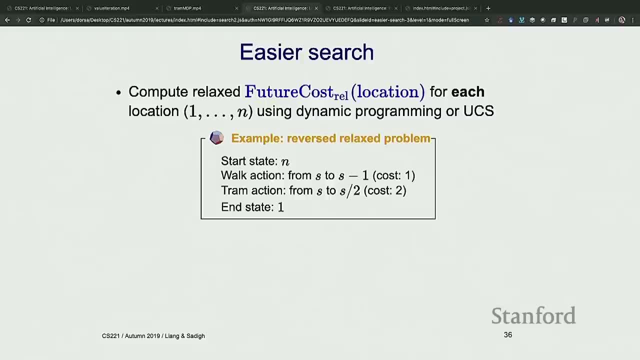 becomes future cost of the relaxed problem, if that makes sense. So so the way I'm reversing this is I'm basically saying start state is n, end state is 1, and my walk action takes me to s minus 1 instead of s plus 1,. 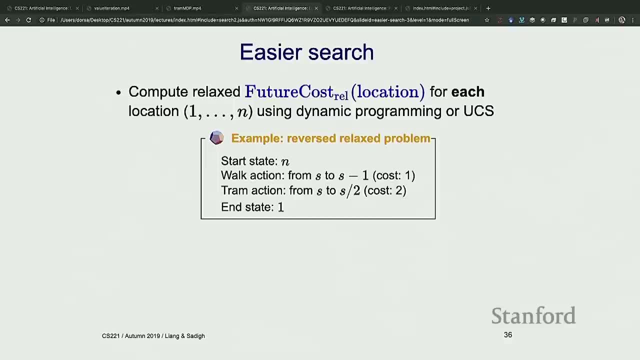 and my tram action takes me to s over 2 instead of s times 2.. And the whole reason I'm doing that is is that the past cost of this new problem is the future cost of the non-reversed version. Okay, Because I, I'm, I need to. 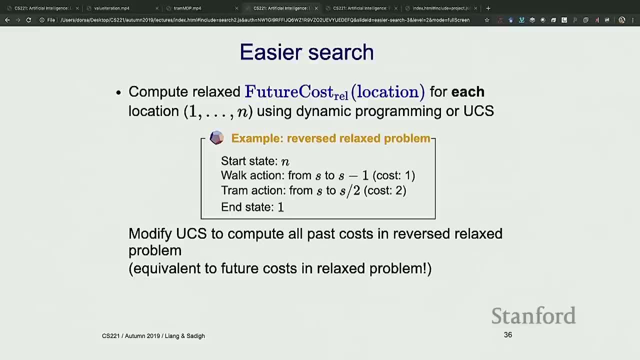 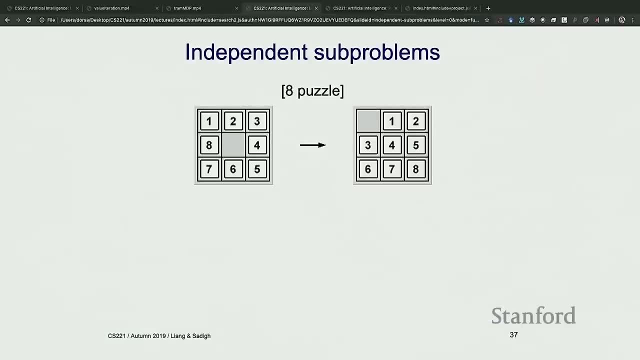 I need to use uniform cost search here. Okay, So I run my uniform cost search. that gives me a heuristic and that heuristic gives me this future cost of the relaxed problem and everything will be great. Another example is I can have independent sub-problems using my heuristic. 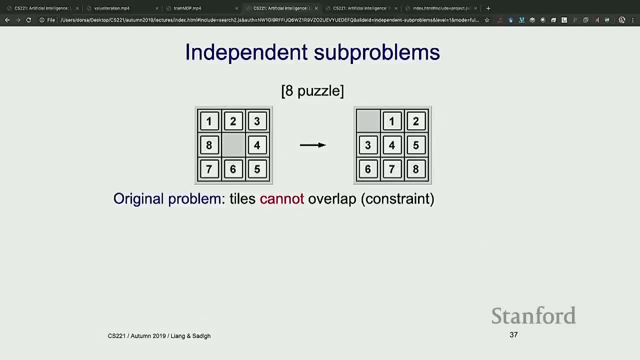 So in this case, like we have these tiles, they technically cannot overlap. Instead, what we are allowing is you're allowing them to overlap. So if they allow them to overlap, I have eight independent sub-problems that I can solve. These sub-problems- give me heuristics. 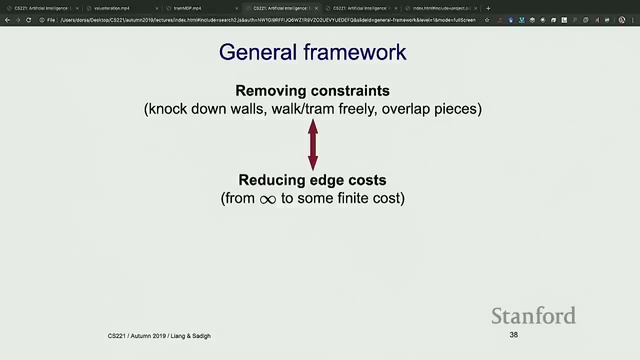 and I can just go with them, Okay, So. so these were just a bunch of examples And kind of the key idea was reducing edge. like when we are coming up with this relaxed problems, we're reducing edge costs from infinity to some finite cost. 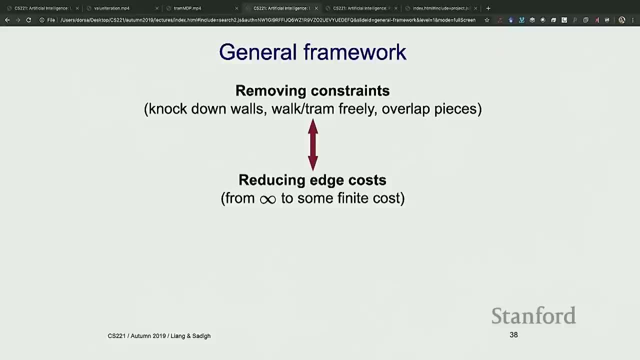 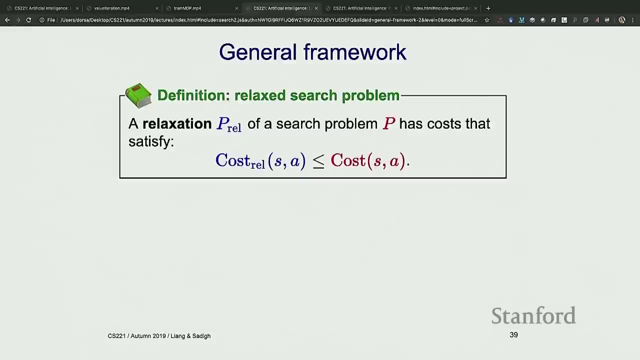 Okay, So I'm getting rid of walls. before I couldn't cross, like it was infinity. cost of that was infinity, But if I get rid of the wall I'm making it a finite cost. So this type of method, um, this is a general framework. 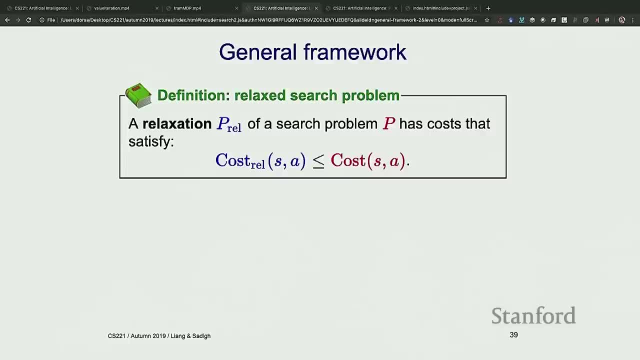 So the point I want to make is: generally you can talk about the relaxation of a search problem. So if you have a search problem P, a relaxation of a search problem- I'm gonna call that P-R-P-R-E-L- is going to be a problem where the cost of the relaxation for 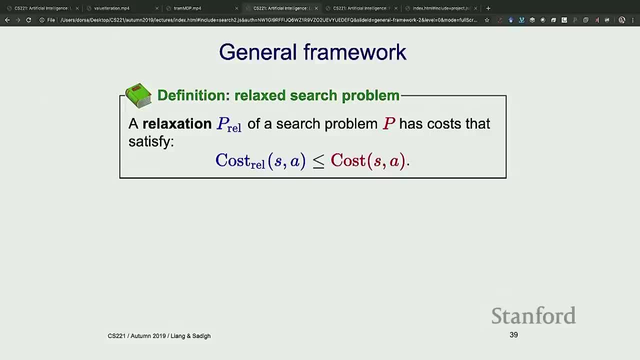 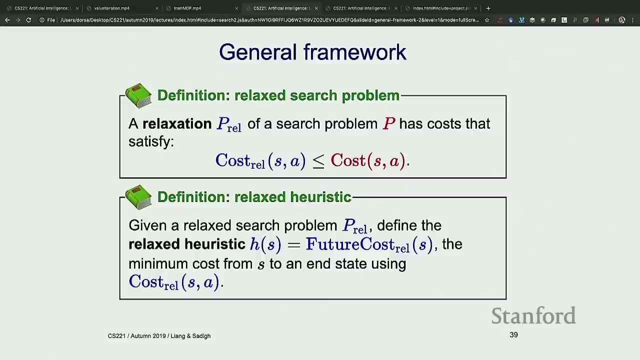 any state action is less than or equal to cost of state in action. I'll take questions afterwards, All right, So, uh, so that is a relaxed problem, Okay, So the cool thing about that is if you're given a relaxed problem. 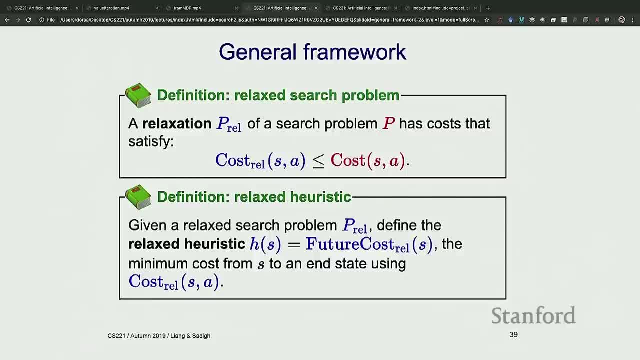 then you can pick your heuristic to be the future cost of the relaxed problem And that is called the relaxed heuristic. Okay, So so this is kind of a recipe, a general framework, Like if someone asks you: find a good heuristic, find a relaxed problem. 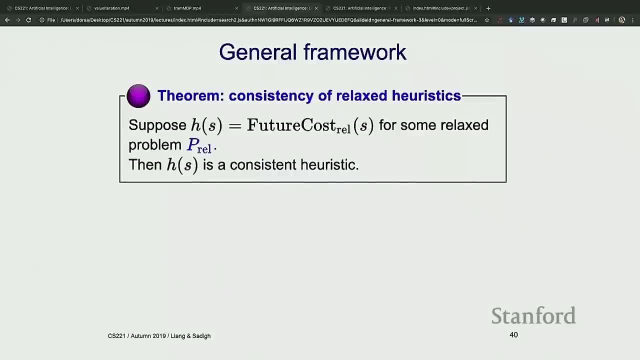 future cost of the relaxed problem is a heuristic, And the cool thing about that is it turns out that that that that future cost of the relaxed problem, which you're deciding to be a heuristic, is also consistent, Because we talked about all these consistency properties and 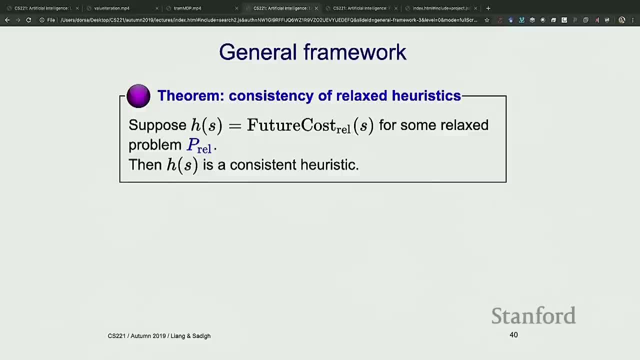 and how you want to find the heuristic to be consistent, for the solution to be correct. And how in the world am I gonna find a consistent heuristic? Well, here is one. Here is one way of finding consistent heuristics. Pick your problem, make it relaxed. 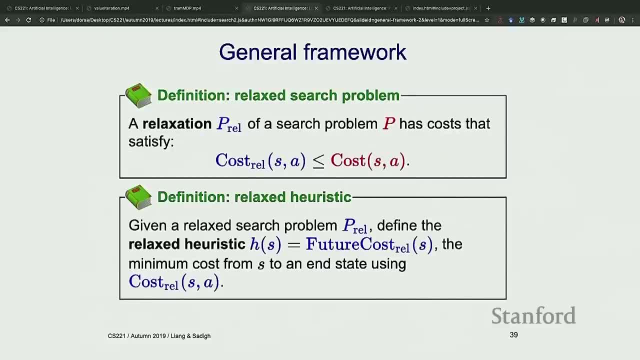 Making it relaxed means that pick a cost that's less pick, pick a relaxed problem where the cost is less than the cost of the original problem, and then future cost of that relaxed problem is just going to be your heuristic, And then it's gonna be consistent. 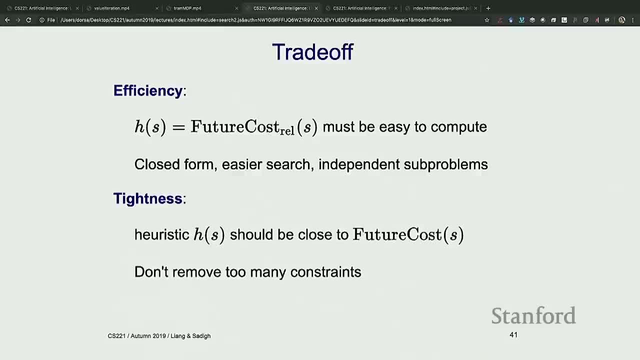 So proof of that is two lines, So I'm gonna skip that. And and the quick thing about this- like, like note about this- is there is a trade-off here. There's a trade-off between efficiency and tightness, So sure, like making things relaxed and removing constraints. 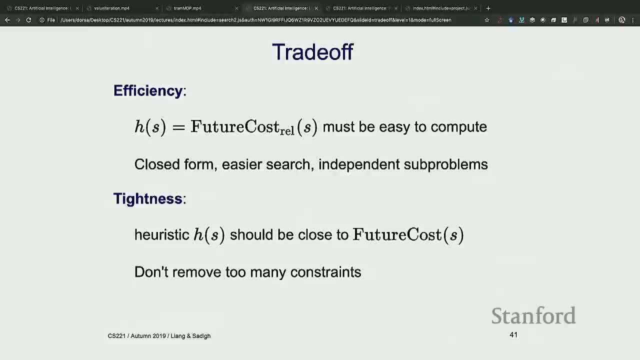 it's kind of fun, right. You have this easier problem and you just solve it and everything is great about it. But it's not like like there is kind of a trade-off between how tight you want your heuristic to be, Like you shouldn't remove too many constraints. 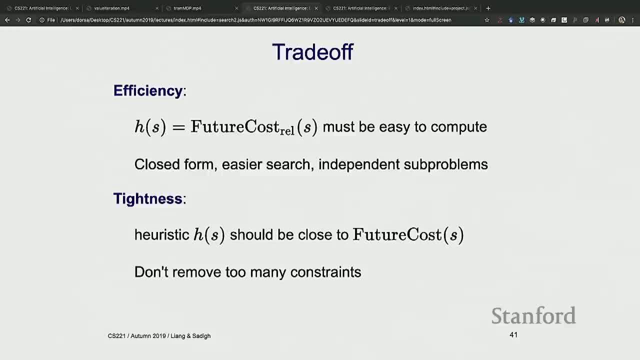 Because if you remove too many constraints, then your heuristic is not a good estimate of future cost. Remember, your heuristic is supposed to be an estimate of future cost. So so if it is not a good estimate of future cost, then it's not tight and it's not that great. 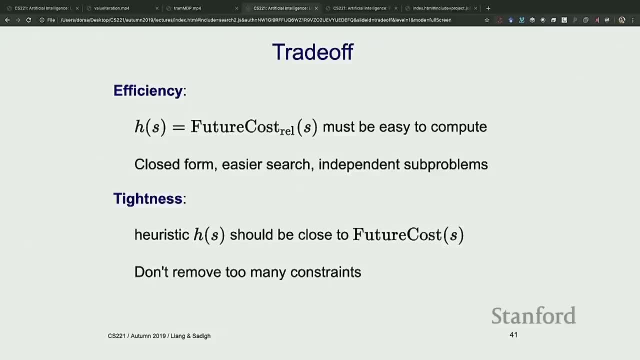 So so there is a balance between how much you're removing your constra-, your constraints, and and how that makes finding the heuristic easier, versus the fact that you want your heuristics to be tight and be close to your future cost. So so don't remove everything. 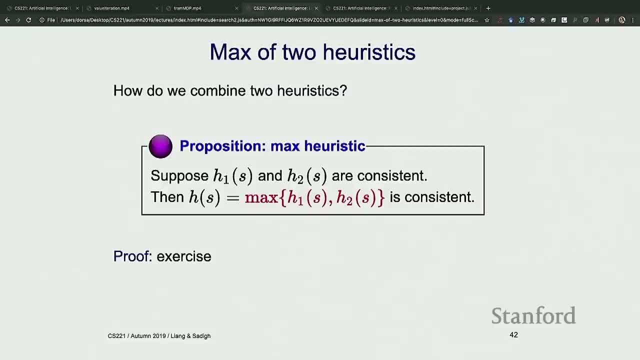 Leave some constraints and then solve it, And you can also do things like: if you have two heuristics that are both consistent, you can take the max of that, and if you take the max of that, it's it's a little bit more restrictive. 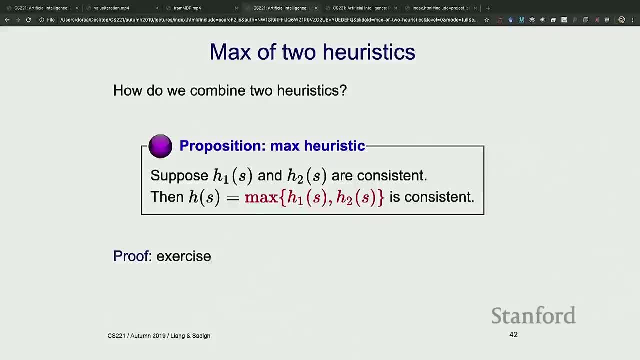 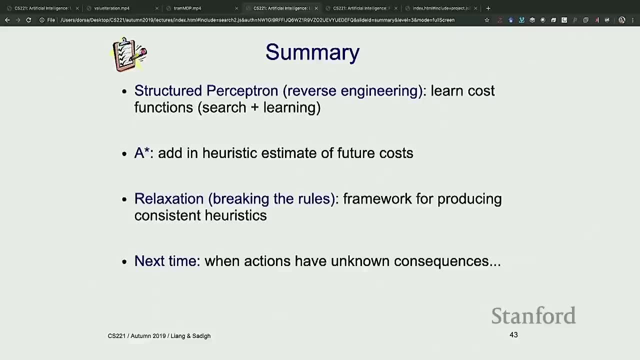 Maybe, maybe that is closer to your future cost and that is, and then you can actually show the max of. that is also consistent, okay, Uh, so we talked about um, like relaxations. A is star. One other quick thing I want to mention, because that wasn't very clear last time. 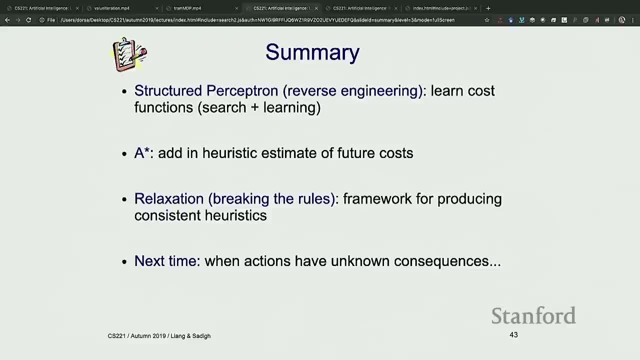 is structured perceptron. We talked about that a little bit too, and we talked about convergence of that. So quick things on: that Structured perceptron actually converges. There was this question that, uh, if we have if that-, if we have a path that is. 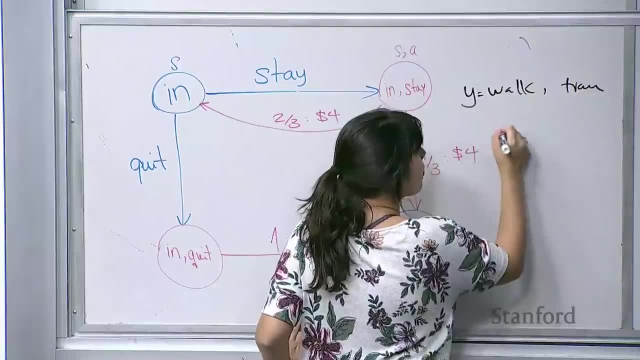 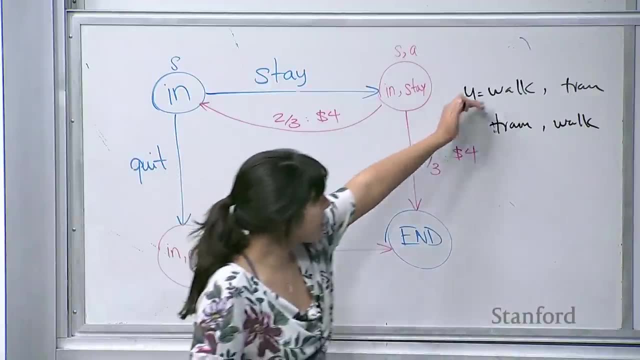 let's say, walk, tram, and, and we end up recovering another path that is tram walk. is that bad, Is that good? Well, turns out that the cost of both of these paths are the same thing. So if I end up getting this path, 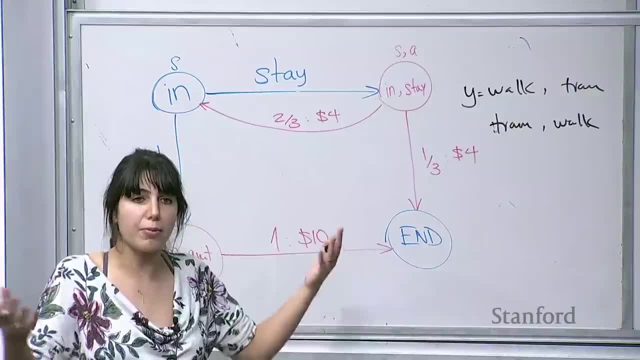 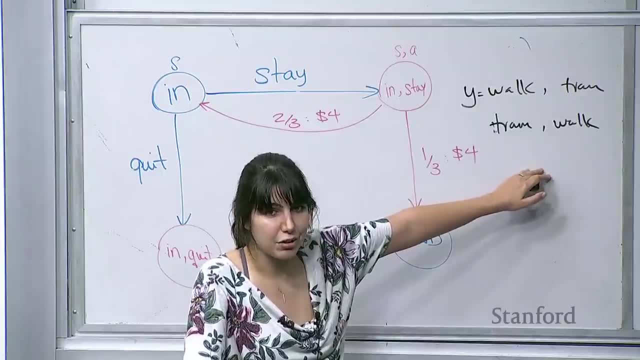 like that's perfectly fine, too right Like that, that is, also with the same optimal weight In the example that we have shown in a tram example. I don't think we are able to get two paths that look like this because of the nature of the example. 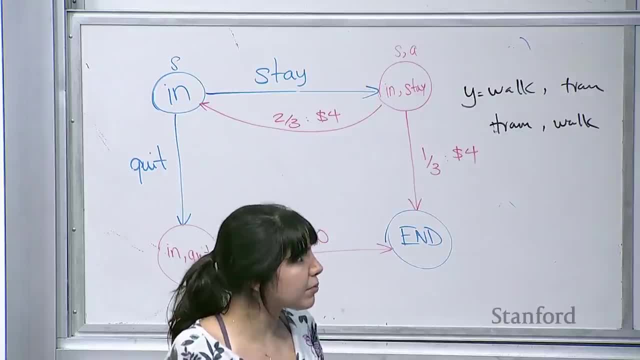 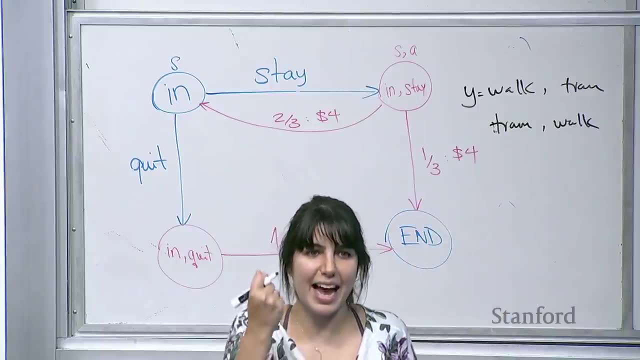 So. so, in general, things to remember from structured perceptron is it does converge. it does converge in a way that it can recover the two y's, but it doesn't necessarily get the exact w's, as we saw last time. right Like you might get two and four. 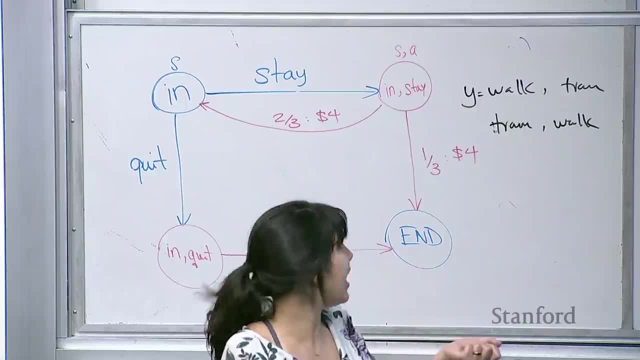 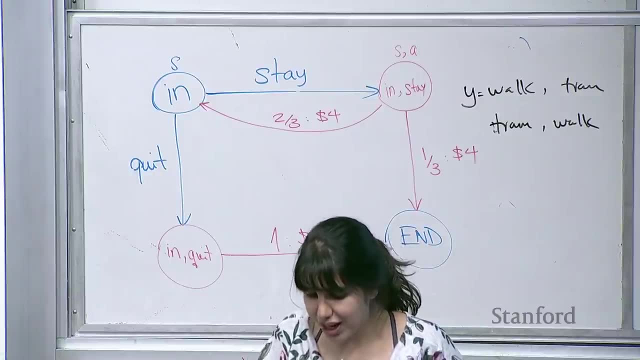 you might get four and eight, like. as long as you have the same relationships, that is. that is enough, But but you are going to be able to get the actual y's and it does converge. So with that, um project conversation is going to be next time. 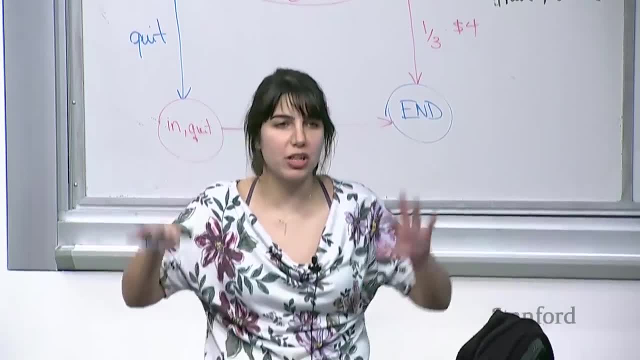 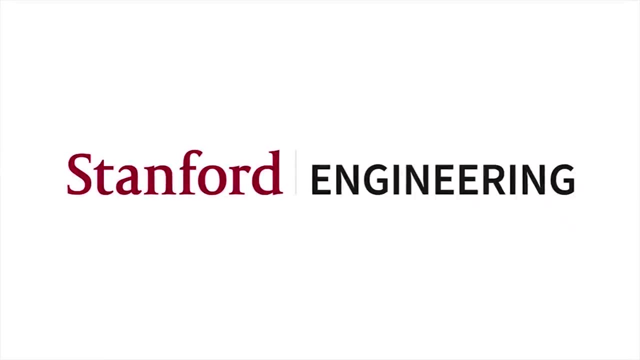 Do take a look at. do take a look at the website. So all the information on the project is on the website. So if you started thinking about it, look at the project page and that has some info And it tells us that you need to get the you need to say you have the first w's and then you don't. So I think it's nice to have that in mind, thinking about what we know about this as a project, and you got to get the first w's, So it's a lot of fun.